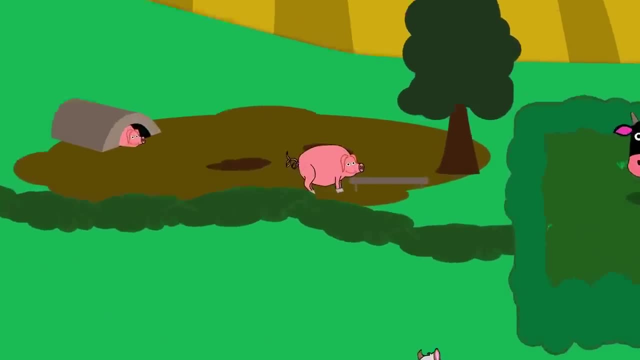 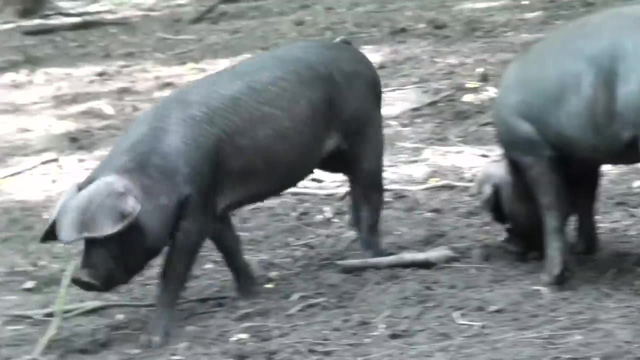 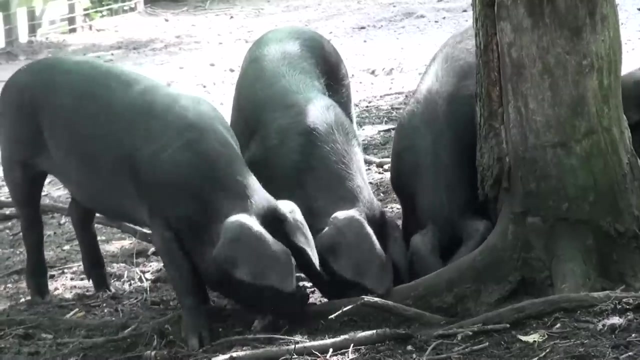 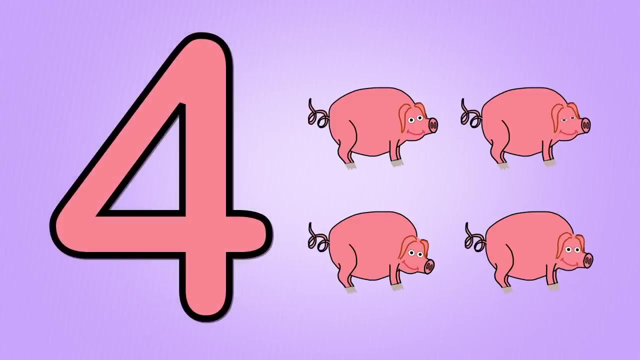 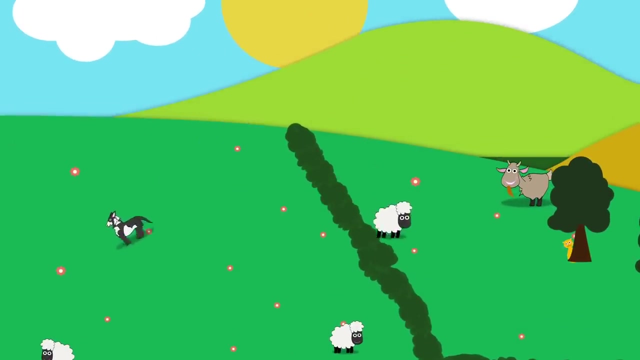 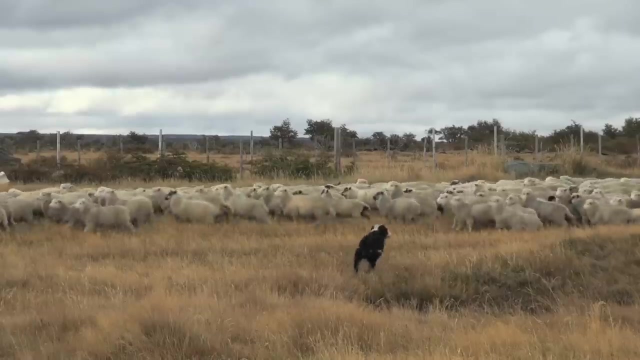 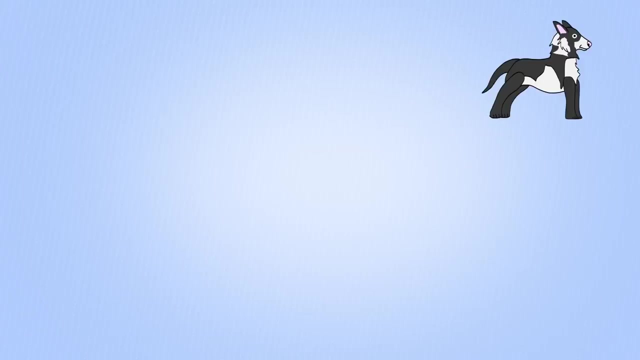 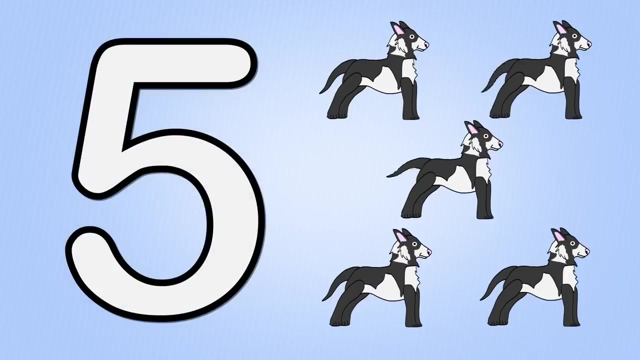 One, two, three, four. Hello, pink pig. One, two, three, four, Four pigs. One, two, three, four. Hello there, clever sheepdog. One, two, three, four, five, Five sheepdogs. 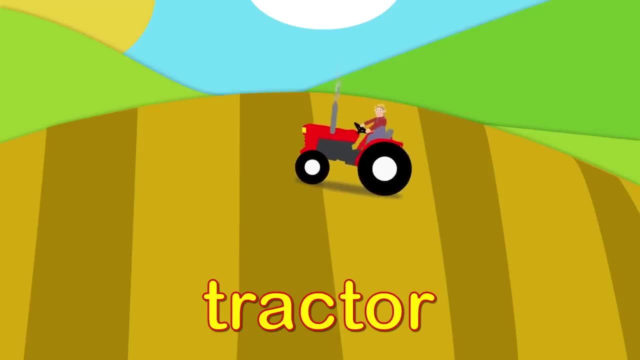 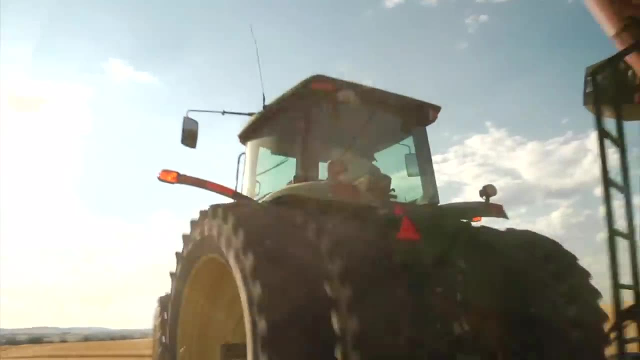 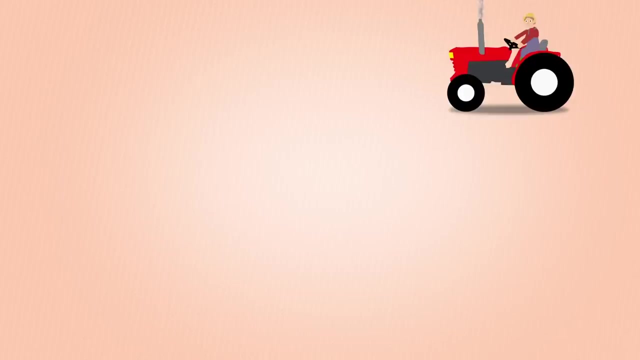 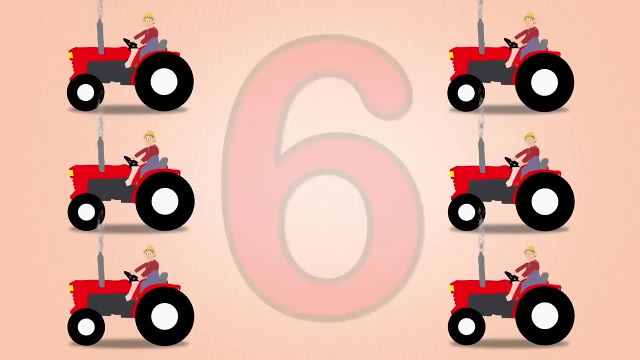 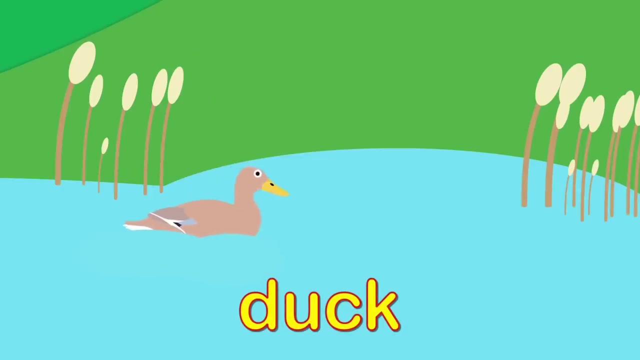 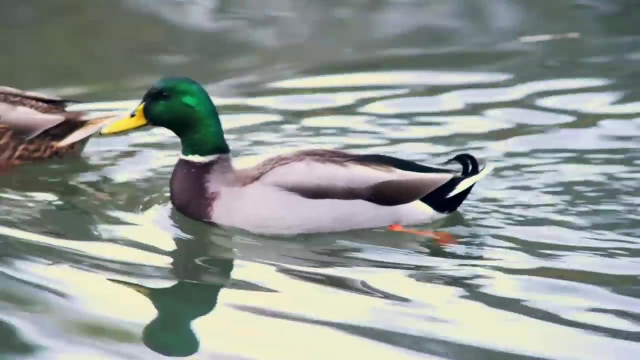 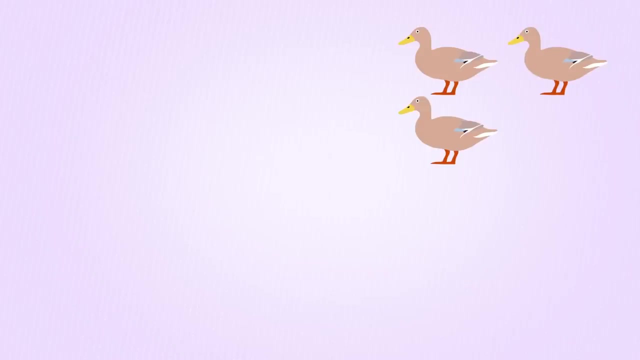 Hello red tractor. One, two, three, four, five, six, Six tractors. Hello quacking duck. One, two, three, four, five, six, seven, Seven ducks: One, two, three, four, five, six. 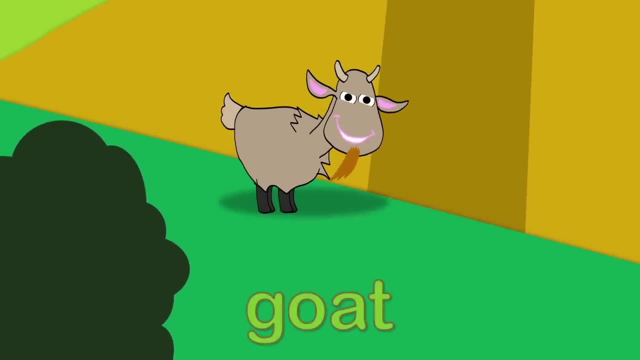 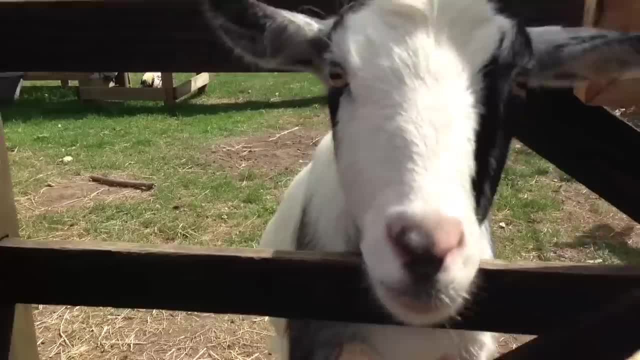 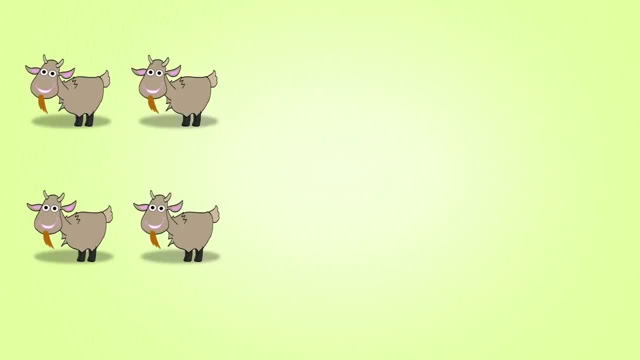 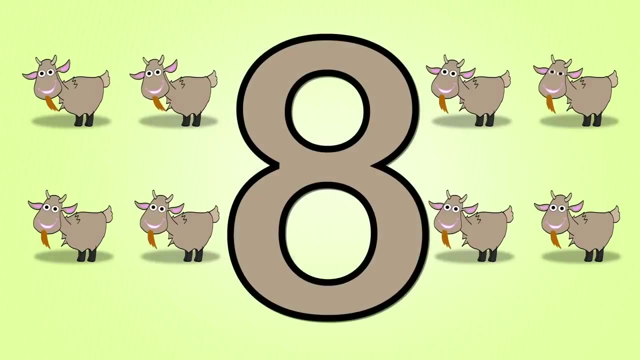 Seven goats. One, two, three, four, five, six. Seven goats. One, two, three, four, five. six Seven goats. One, two, three, four, five, six, six, seven, eight, Eight goats. 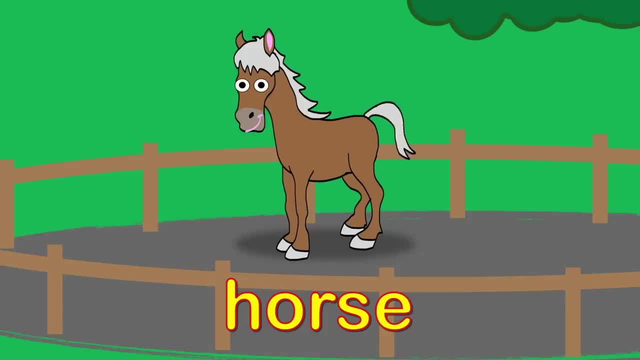 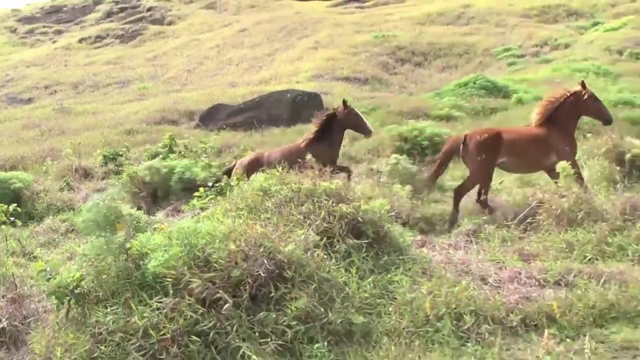 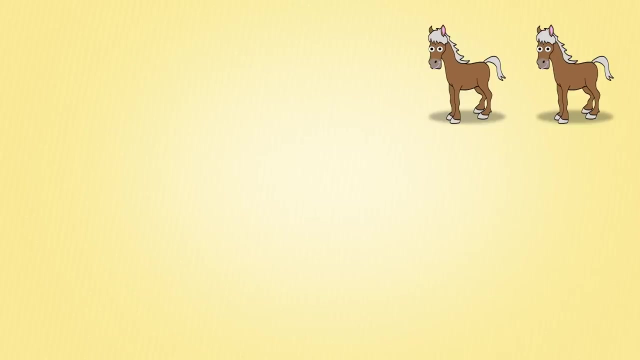 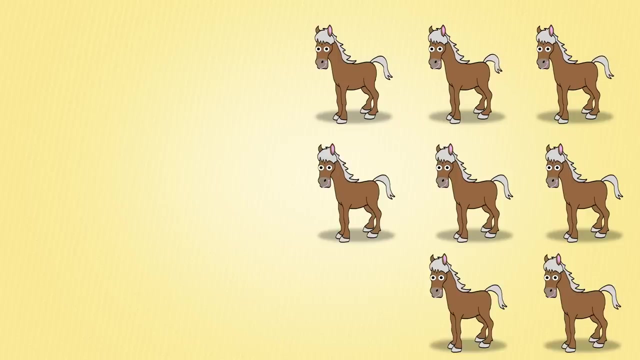 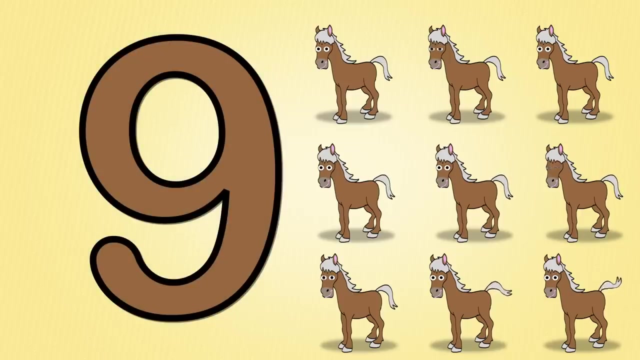 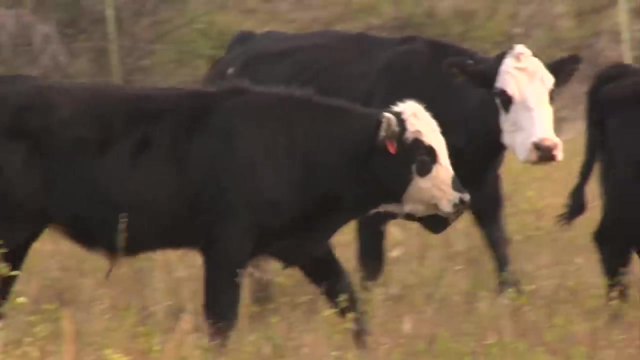 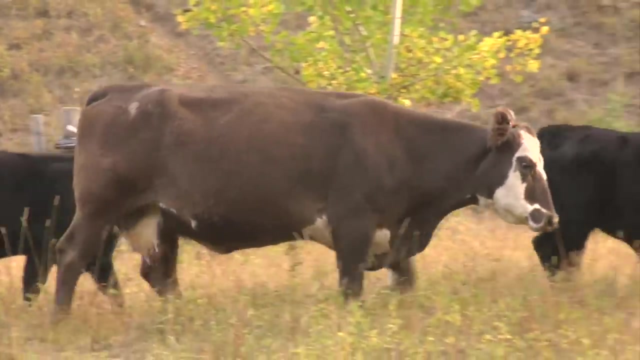 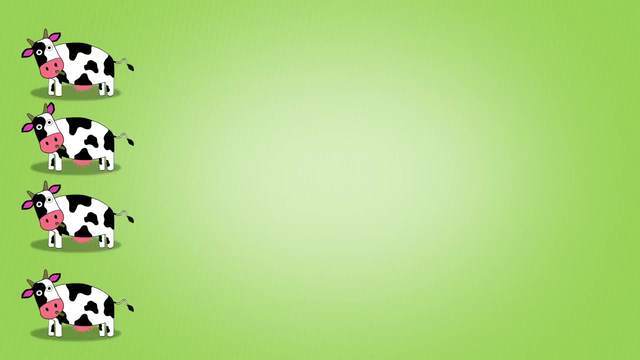 Hello lovely brown horse. One, two, three, four, five, six, seven, eight, nine, Nine horses. Hello moo moo cow: One, two, three, four, five, six, seven, eight, nine, ten. 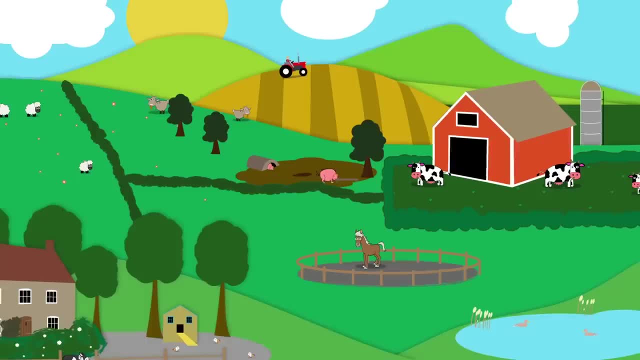 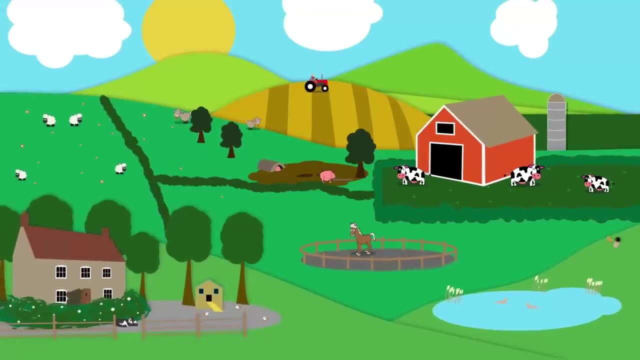 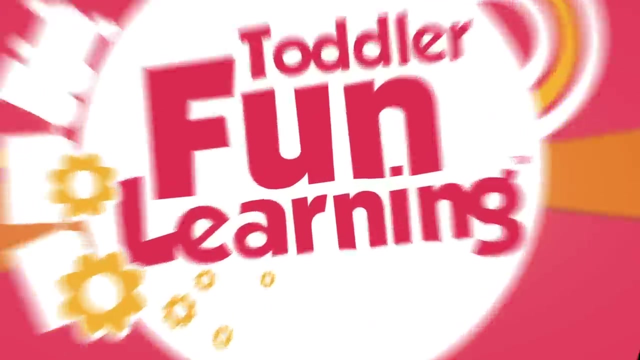 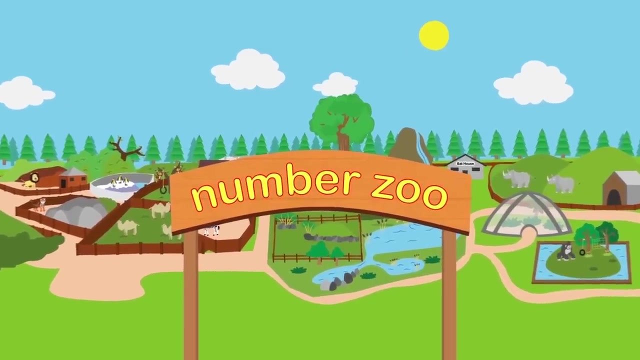 Ten cows. Thank you for visiting Number Farm. Have a good day. See you again soon. I'm Kirsty the Chameleon and I've lost my colours. Maybe my friends at Number Zoo can help me find them. Have you met the animals? There are quite a few. 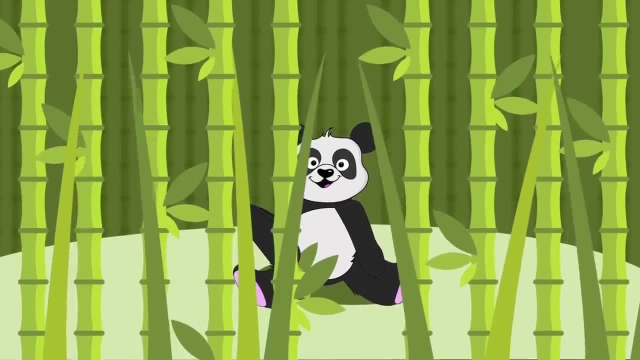 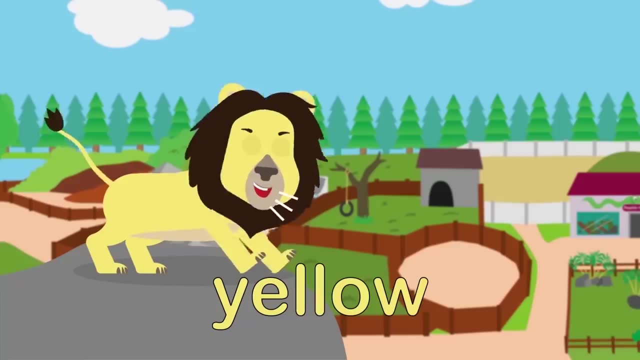 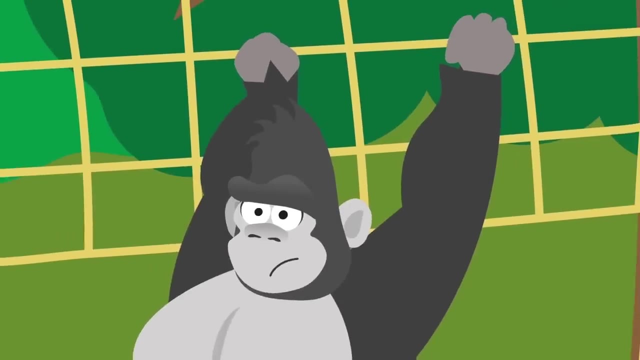 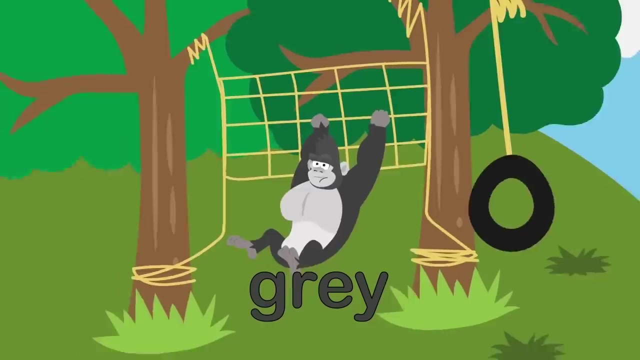 Let's look for my colours as we go round the zoo. The lion's the king, with a fine yellow coat and a roar that rumbles from the back of his throat. The gorilla is strong and his fur is dark grey. He might look quite scary, but he just loves to play. 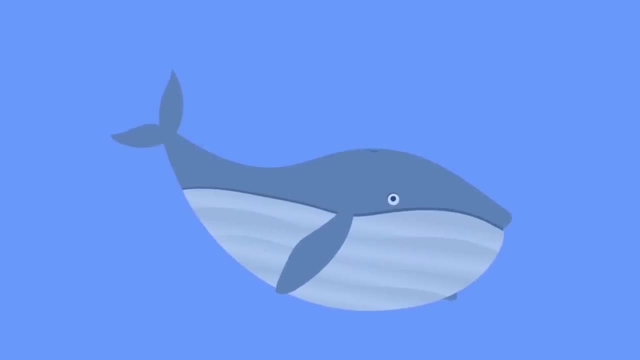 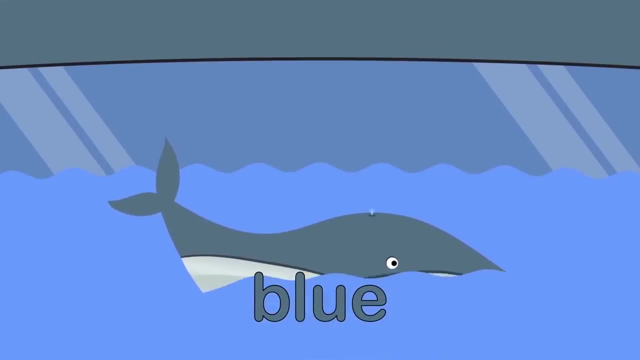 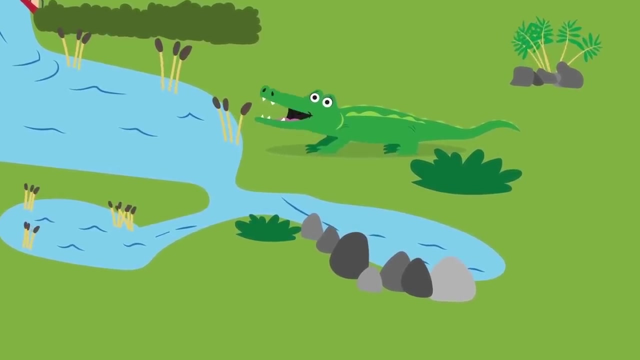 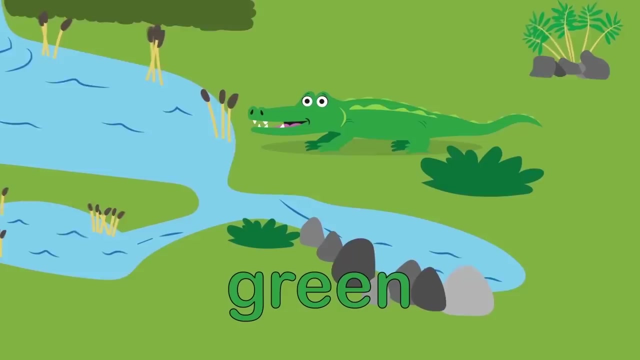 Down in the deep lives. Harry the Whale. His thick skin is blue, from his nose to his tail. Alligator yawns: His teeth look so mean, His claws are quite sharp and his scales are dark green. He's got a lot of hair. He's got a lot of hair. 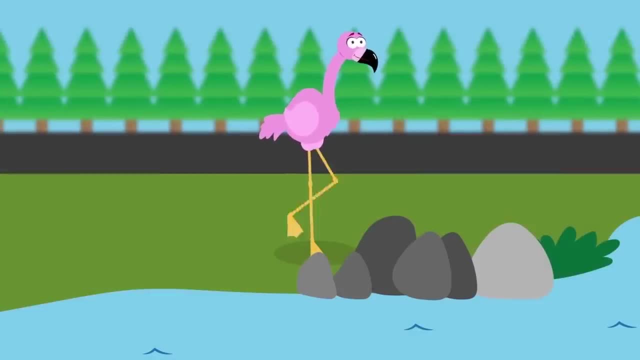 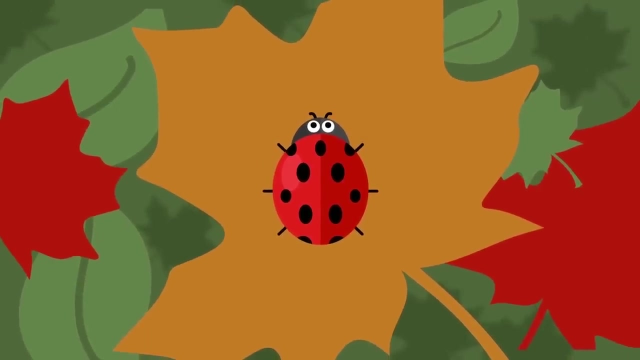 He's got a lot of hair. My friend the flamingo loves to stand and just think His feathers are soft and a lovely bright pink. His feathers are soft and a lovely bright pink. The ladybird has wings tucked into her back. Her colour is red with a few spots of black. 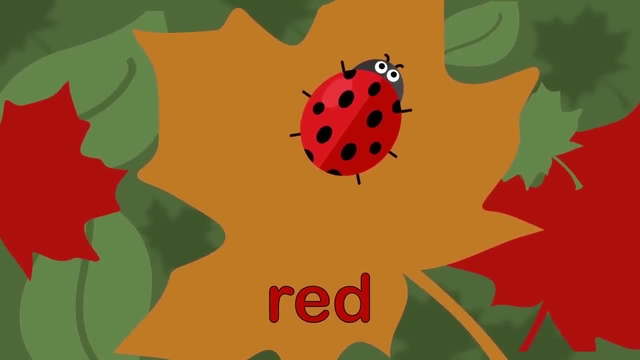 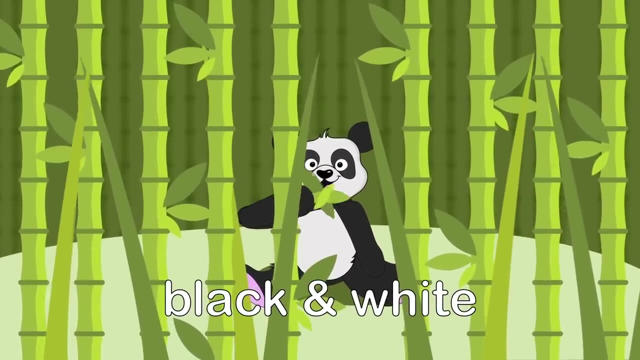 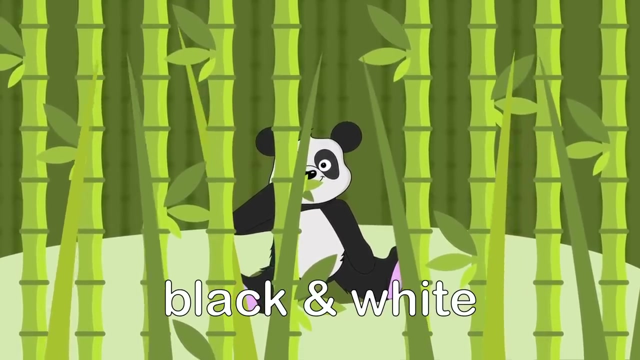 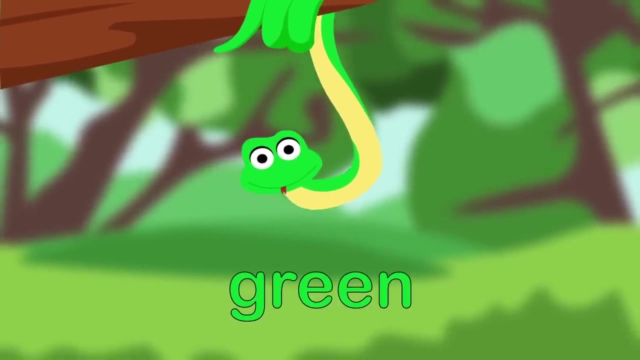 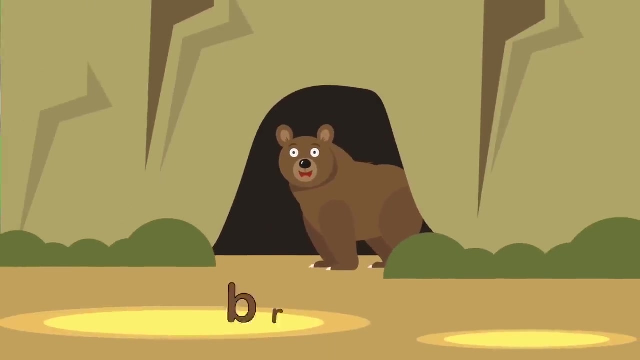 The black and white panda is cheeky and funny. She eats lots of bamboo and then rests when it's sunny. Coiled around a branch, you cannot mistake The shiny green shape of Lucinda the snake With a shaggy brown coat. the bear lives in a cave. 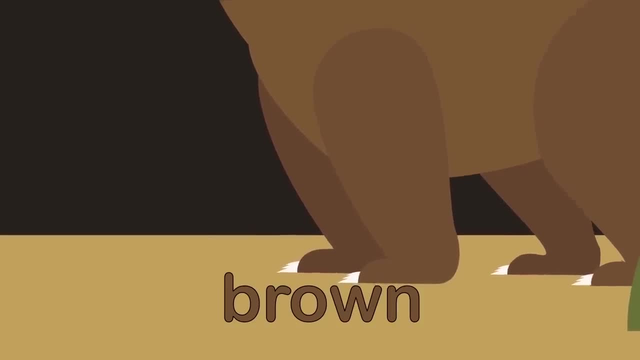 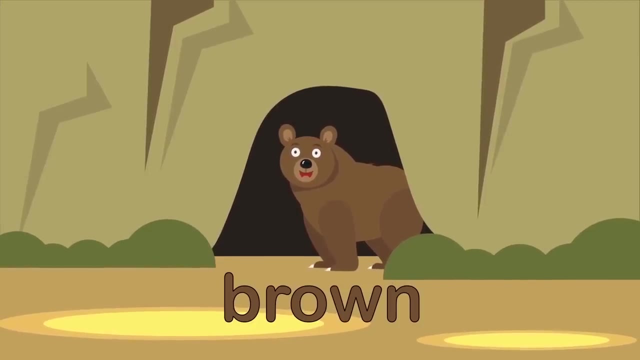 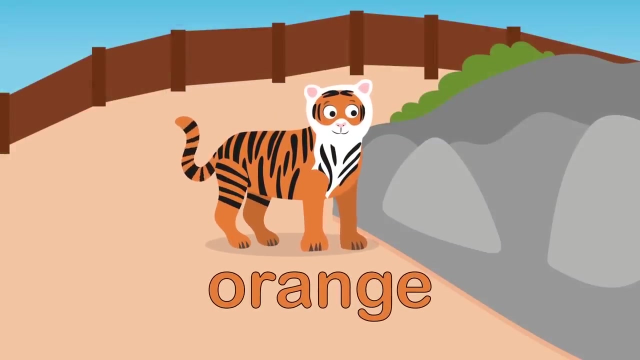 His claws may be sharp, but he knows how to behave. The orange striped tiger pads around on all fours. She swishes her tail and she sharpens her claws. The pink tiger has a big tail. She's got a lot of hair. The penguin looks smart in a black and white suit. 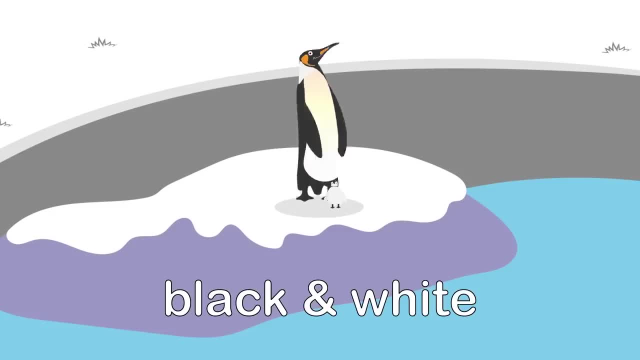 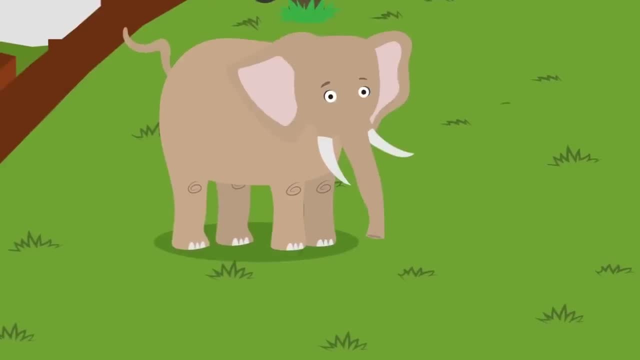 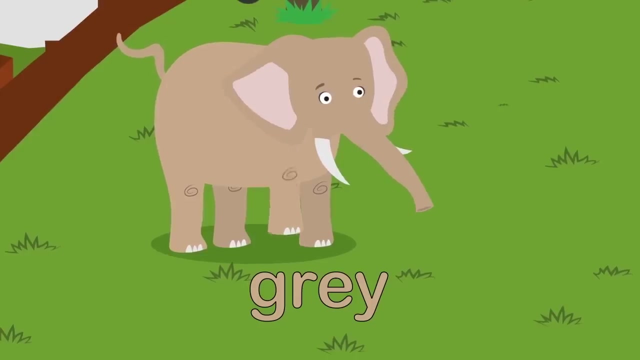 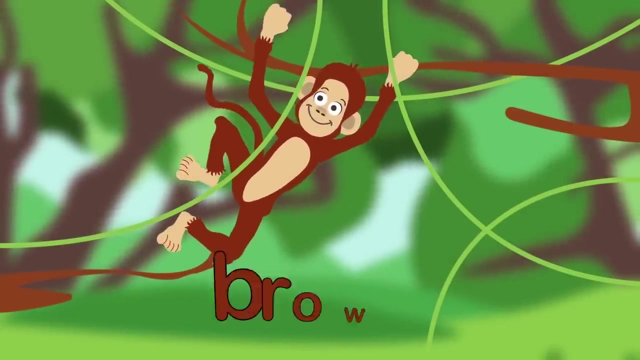 And his baby is soft and so fluffy and cute. This elephant is one of the kindest you'll meet. She's wrinkly and grey And she's got massive feet. The monkey loves climbing And his fur is light brown. From up in the tree he loves to swing down. 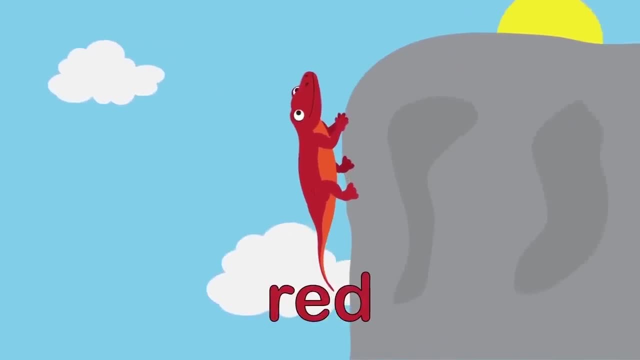 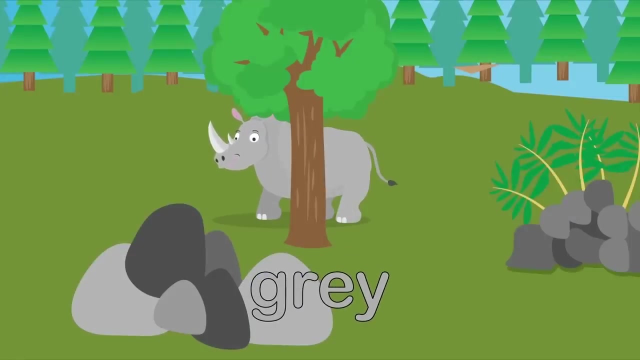 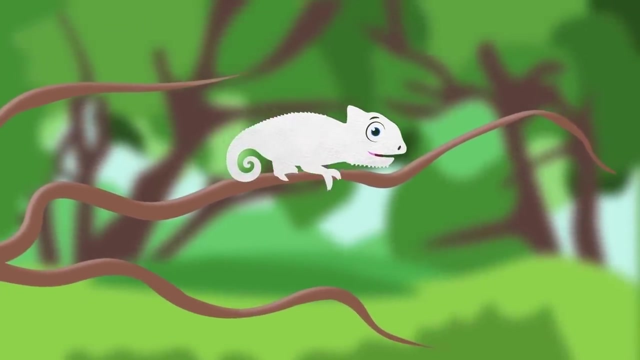 With a slimy red body and sticky red toes. How does Newt do it, Nobody knows. With a dusty grey hide and a horn on her nose, The rhino stands out wherever she goes. It's zoo closing time, so we must say goodbye. 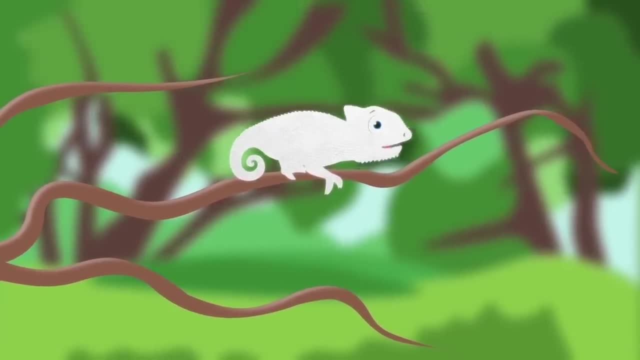 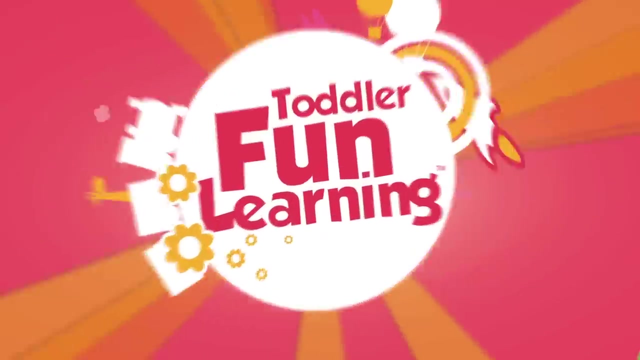 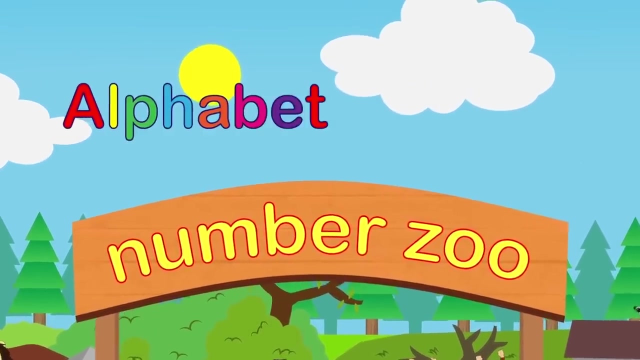 Are my colours back? I'll give it a try. Look at my skin. It's starting to glow, Shimmering and bright, Just like a rainbow. Newt Report, Alphabet Animals. can you see? Will you sing the letters with me? 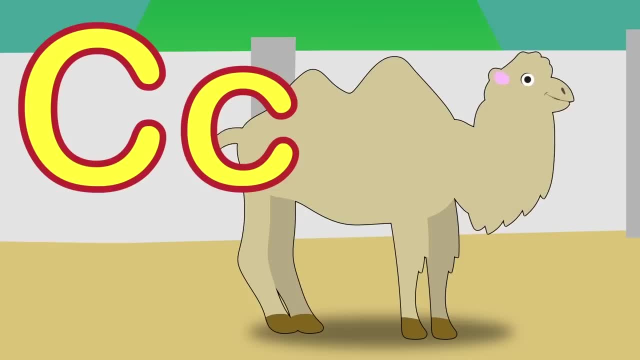 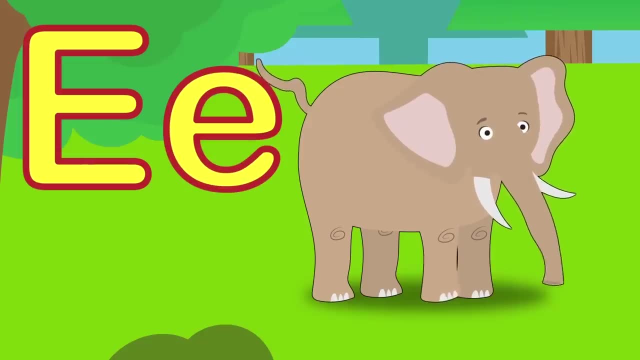 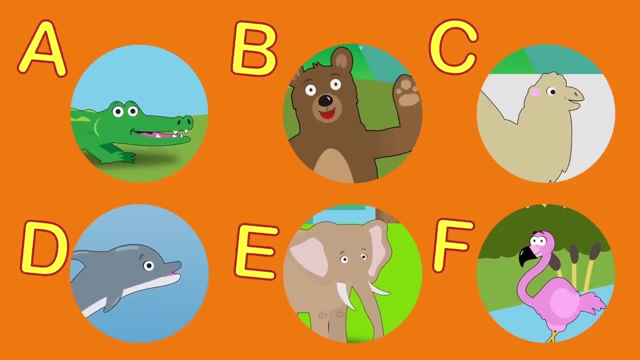 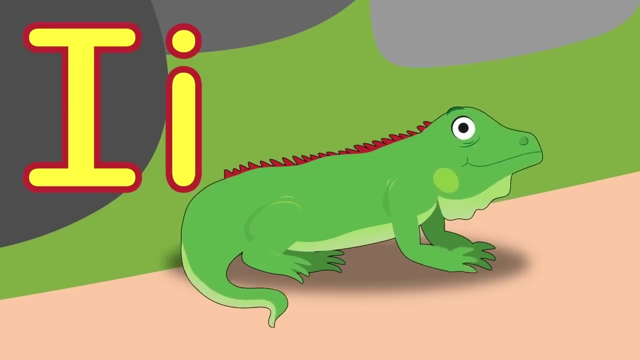 A for alligator. B for bear. C is for camel all covered in hair. D for dolphin. E for elephant. F for flamingo with pink, pink feathers. Alphabet Animals: A, B, C. will you sing the letters with me? G for Gorilla. H for Hippo. I for Iguana. he's green and slippy though. 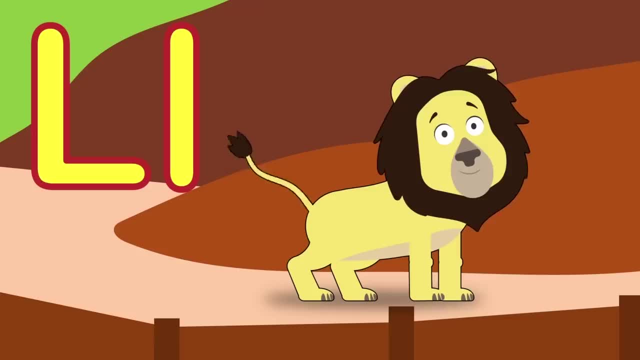 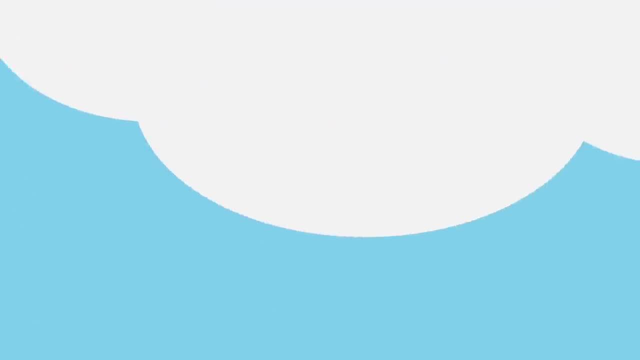 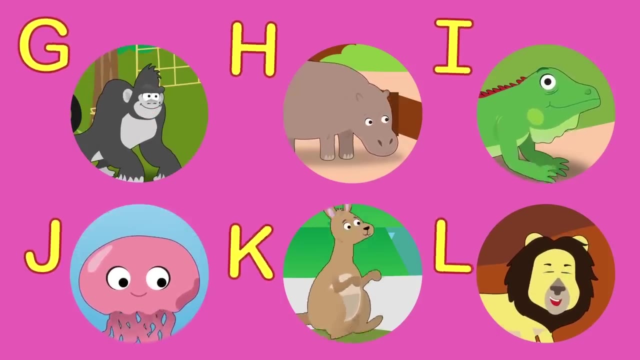 J for Jellyfish, K for Kangaroo, L for Lion. he's sure to roar at you. Alphabet Animals. look and see. will you sing the letters with me? M for Monkey, N for Newt, O for Owl. can you hear her hoot? 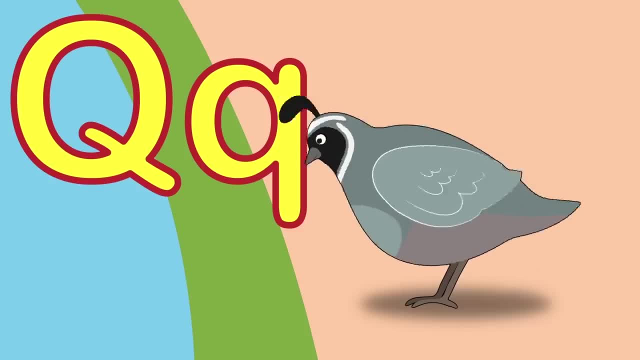 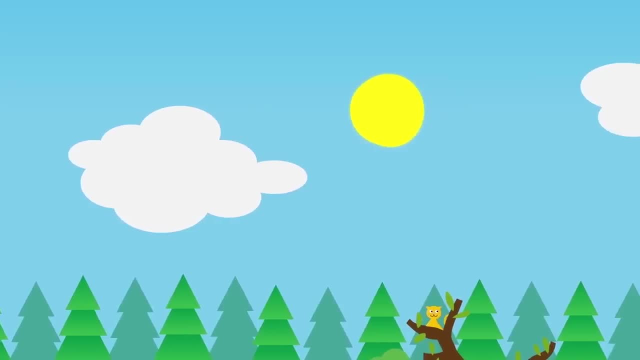 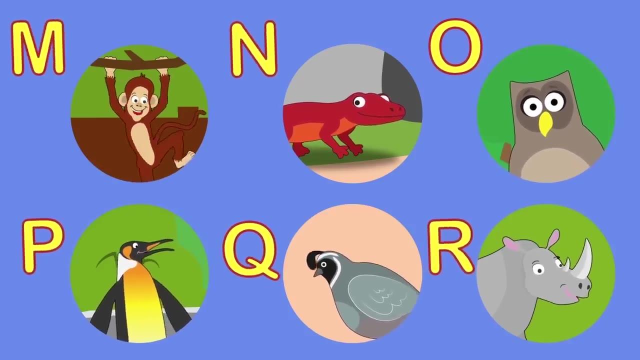 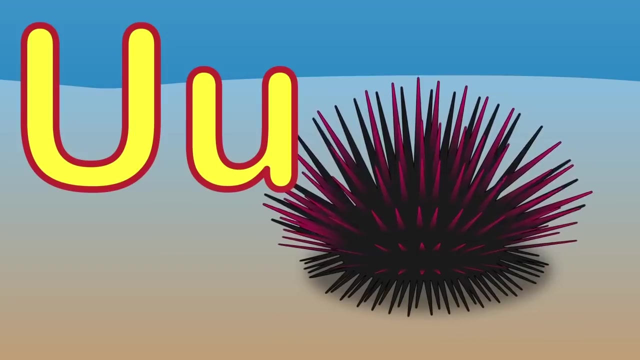 P for Penguin, Wibble wobble, wibble wobble. Q for Quail, R for Rhino. he's as tough as nails. Alphabet Animals. Can you see, will you sing the letters with me? S for Snake and T for Tiger, U for Urchin. it's like a spiky spider. 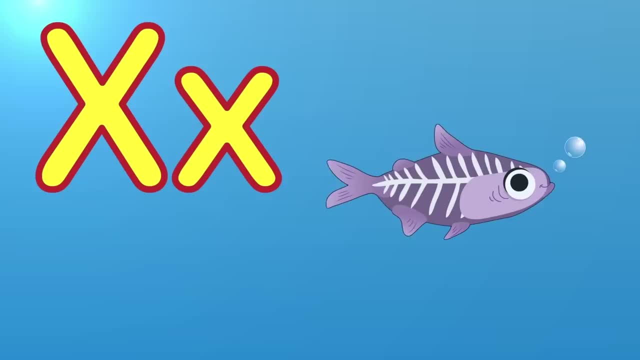 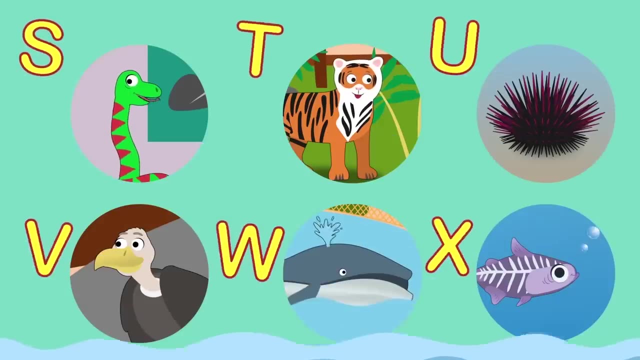 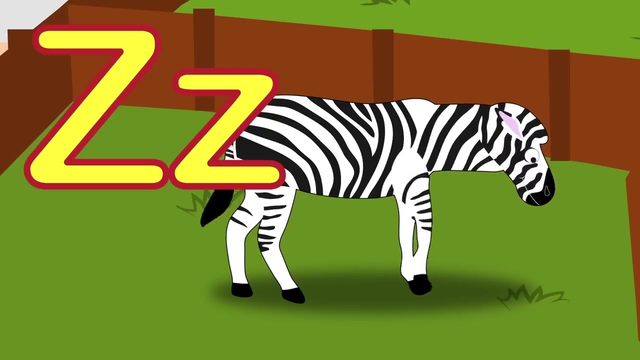 V for Vulture, W for Whale, X for X-Ray Fish. she looks very pale. Alphabet Animals. can you see? will you sing the letters with me: Y for Yak and Z for Zebra. now you've sung the Animal Alphabet. 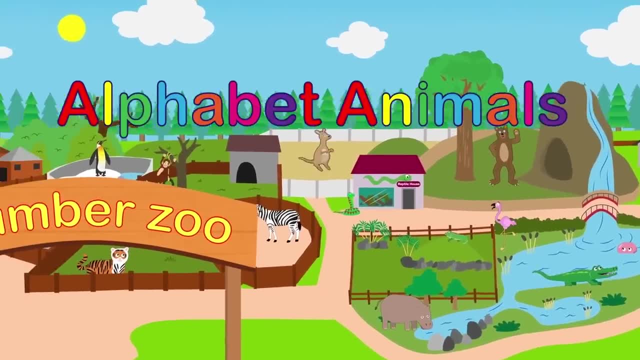 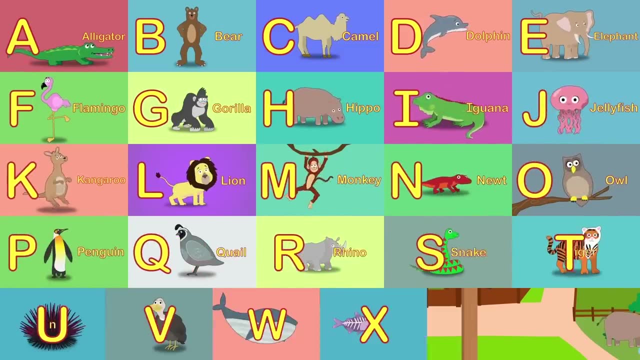 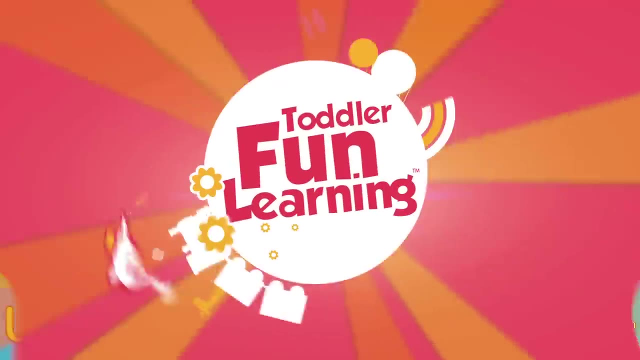 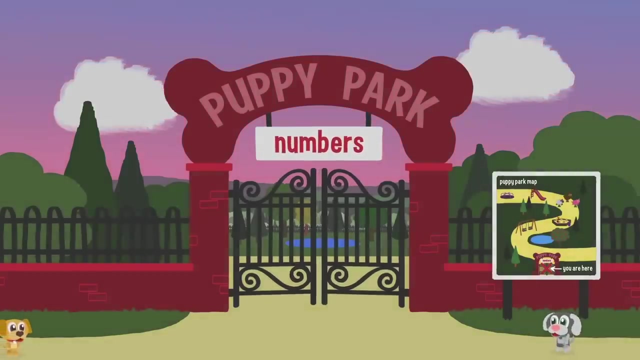 Alphabet Animals: A, B, C. now you've sung the letters with me. Alphabet Animals. can you see, now you've sung the Animal Alphabet. now you've sung the Animal Alphabet. Hello, everyone, welcome to Puppy Park. 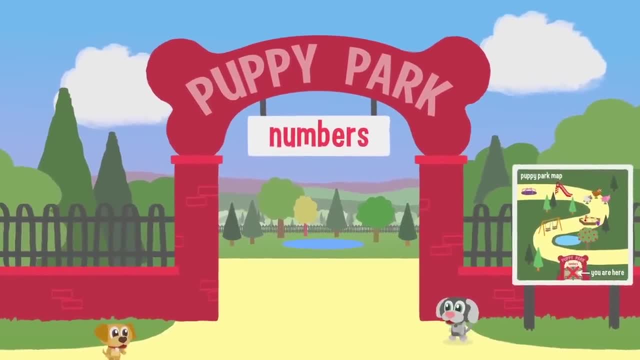 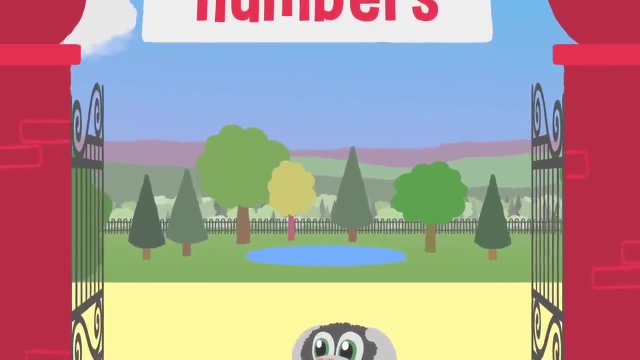 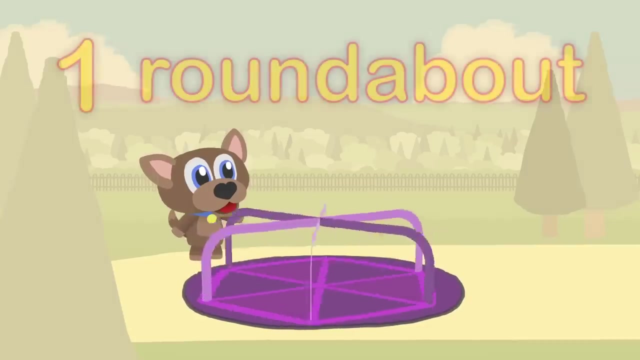 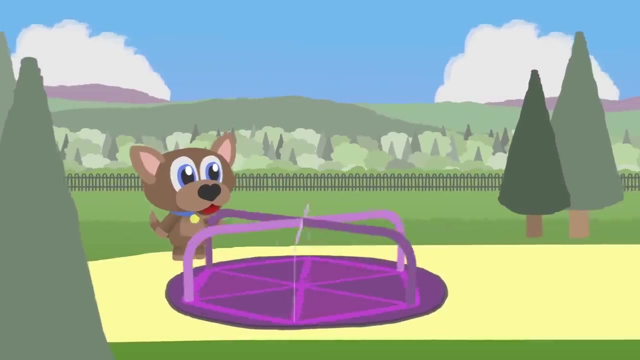 Today we are going to learn to count to ten. Would you like to help us? Are you ready? Let's count. Hello, Freddy, One One, One roundabout. Ollie is on the big red slide, but Henry likes the small blue slide. 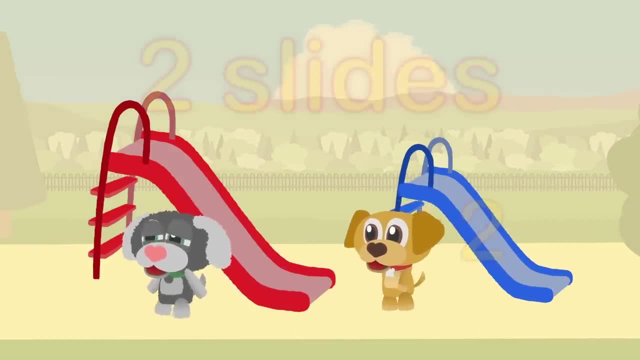 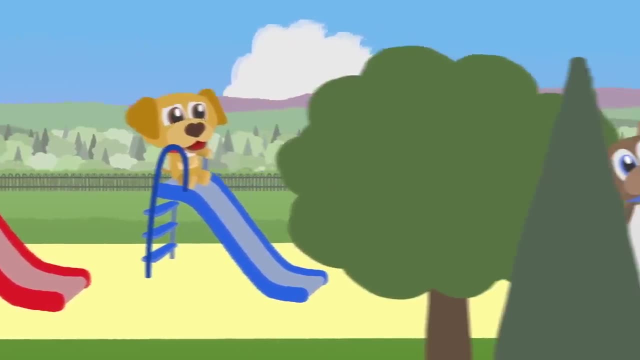 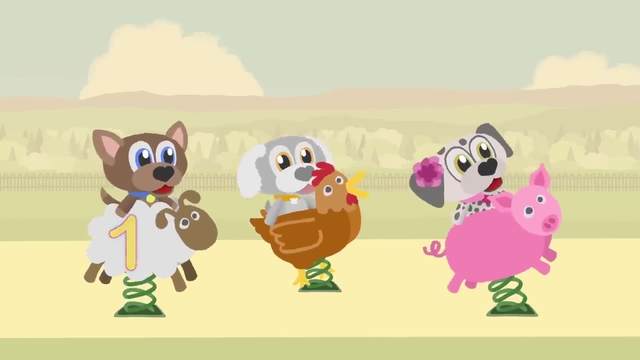 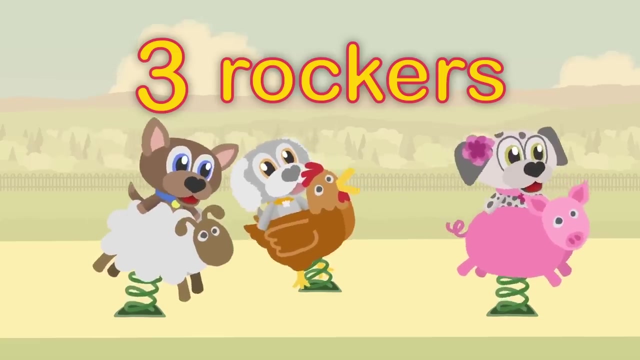 There's one, two, two slides. Peter and his friends are having fun on the springy animals. Let's count them: One One, Two, One, One, Two, One, Two, One, Two, Three, Three rockers. 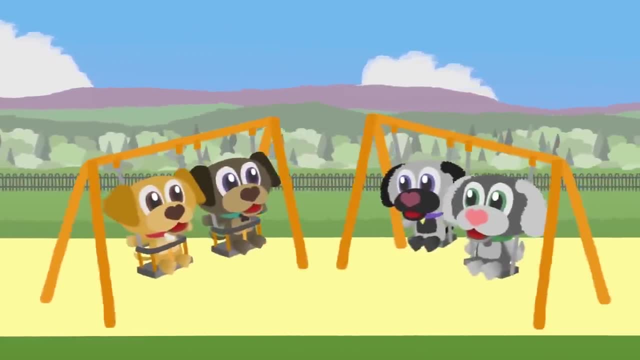 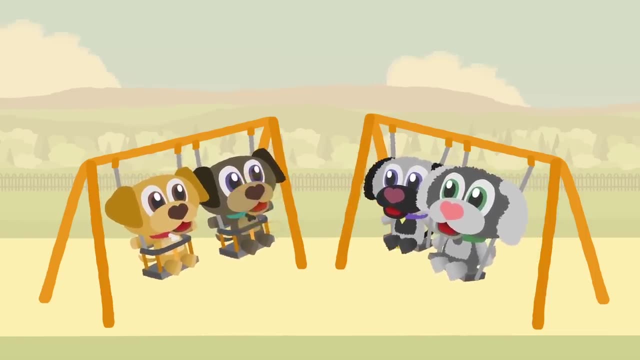 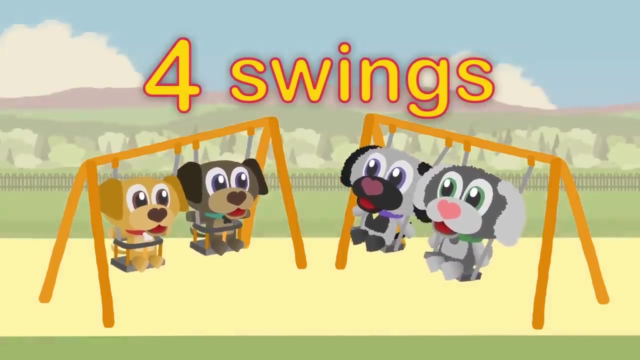 Look how much fun they're having on the swings. Who can swing the highest? One One One One Two, Two, Two, Three, Three, Four, Four, Four swings. One One, One, One One. 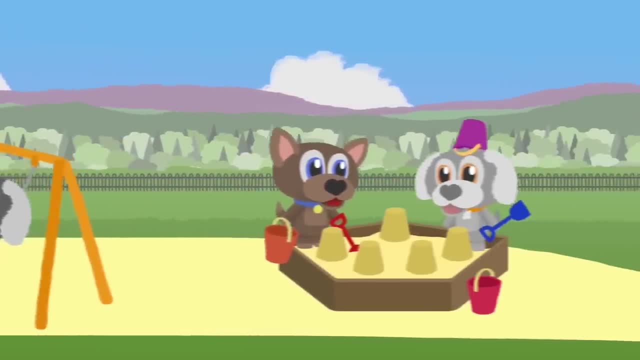 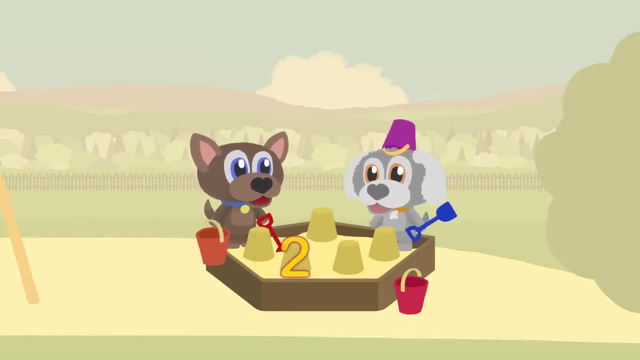 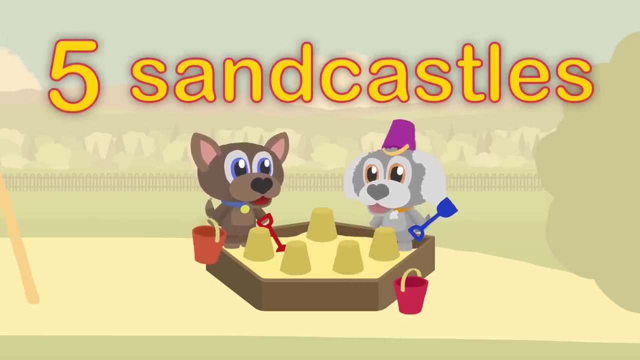 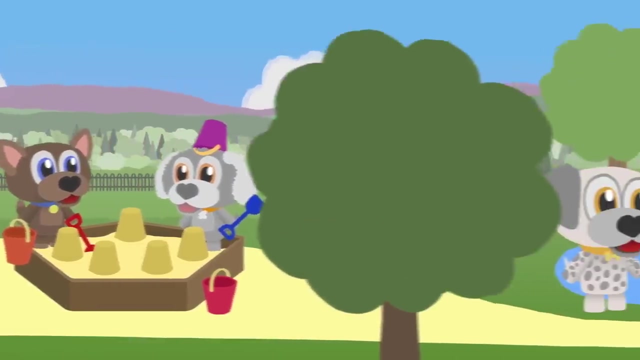 One. Peter and Bertie are in the sandpit. How many sand castles can you see? One, Two, Two, Three, Four, Four, Five, Five sand castles. Dottie is feeding the ducks with Grandpa dog. 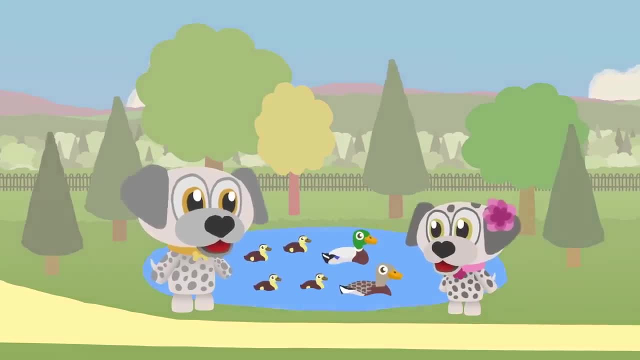 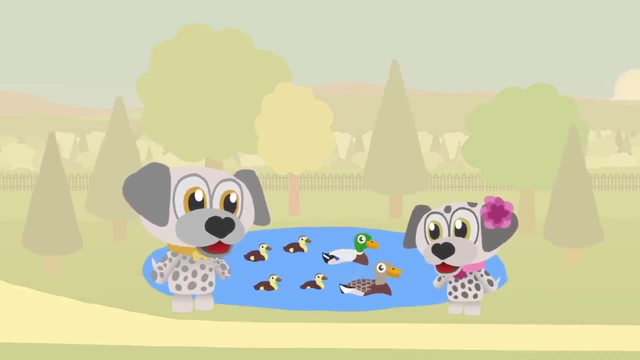 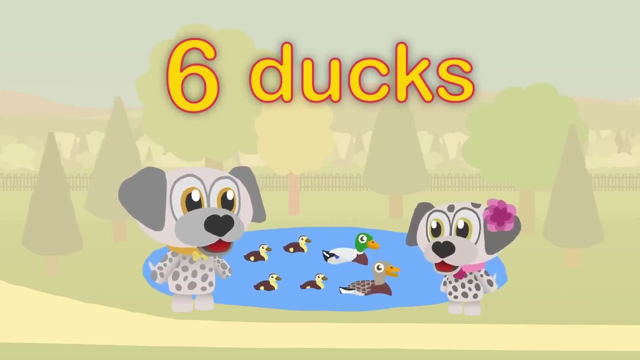 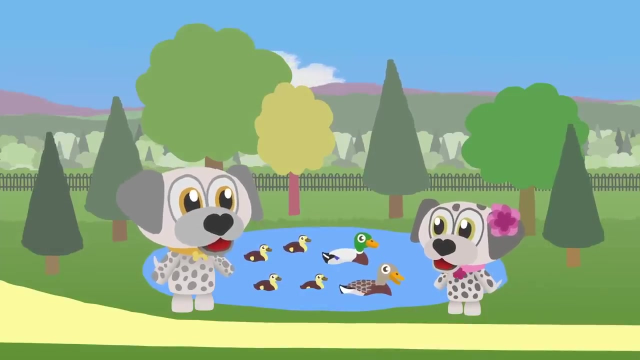 grandpa dog, How many ducks are in the pond? One, two, three, four, five, six, Six ducks: One mummy, one daddy and four ducklings. What else can we count? Oh, look, there's some trees. 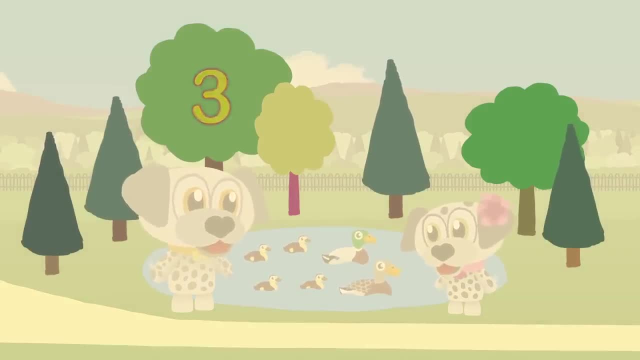 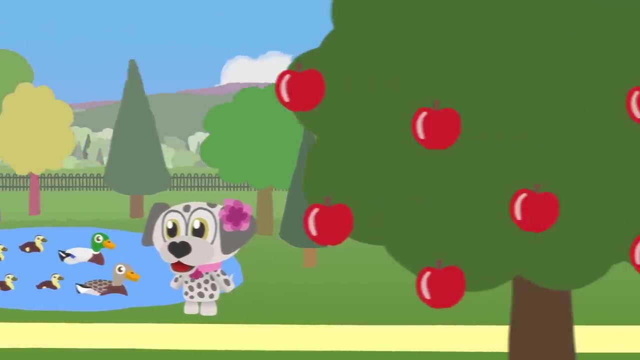 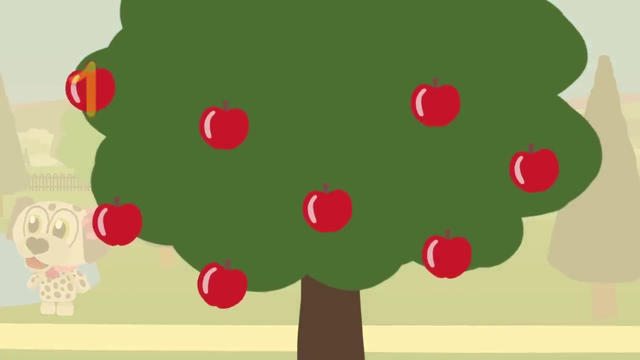 One, two, three, four, five, six, seven. There are seven trees. Ooh, look at those juicy red apples. How many are there? One, two, three, four, five, six, seven, Eight juicy red apples. It's a perfect windy day for flying kites. 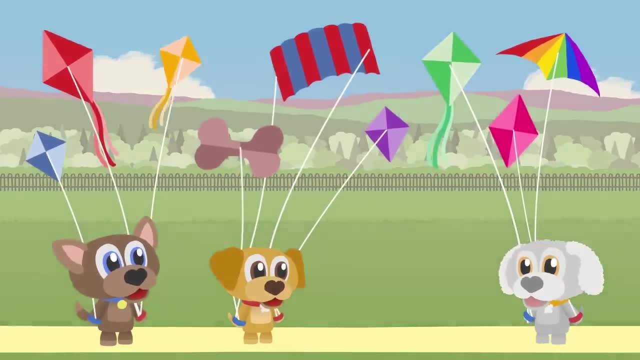 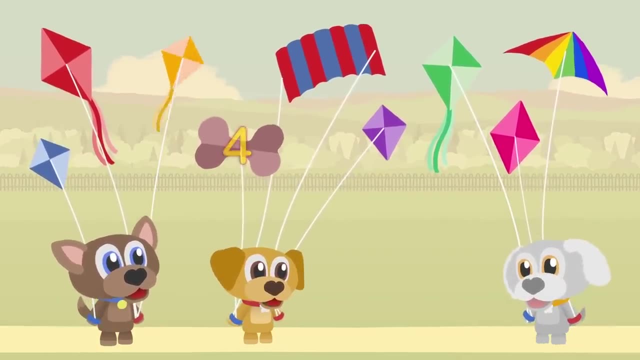 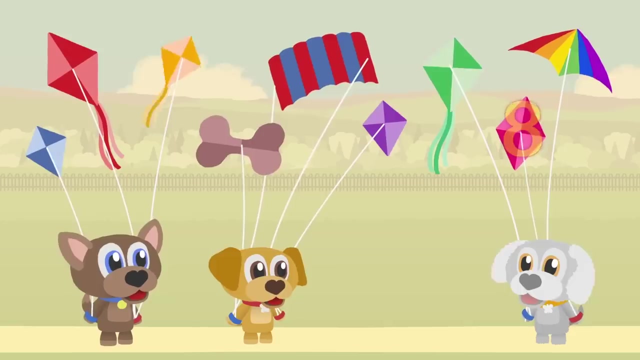 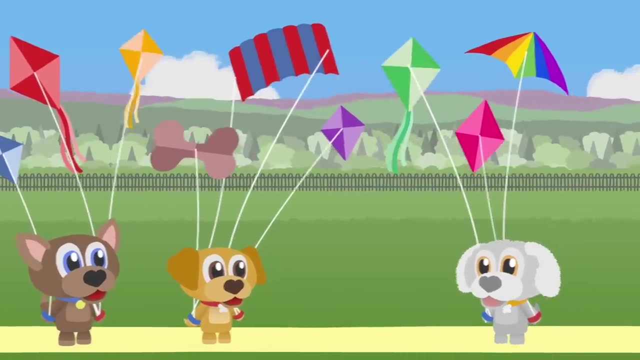 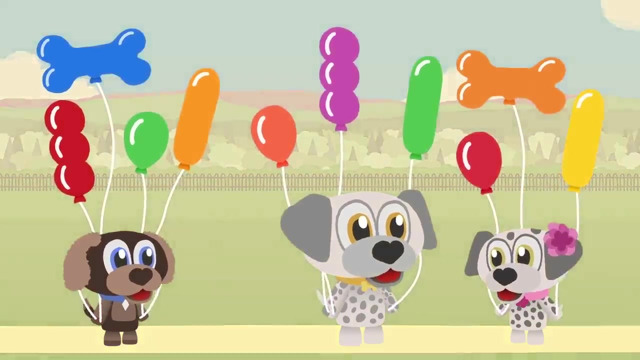 How many kites can you see in the sky? One, two, three, four, five, six, seven, eight, eight, nine, nine kites? Look at all the colourful balloons. How many are there? One, two, three? 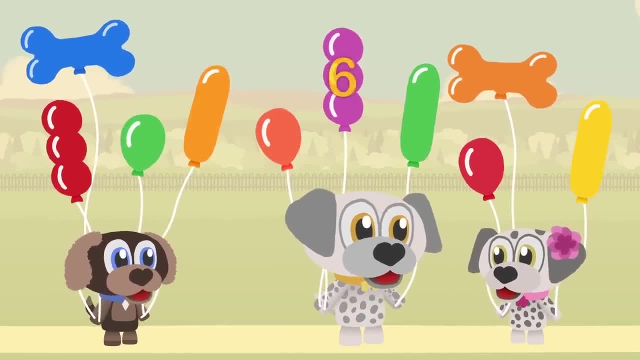 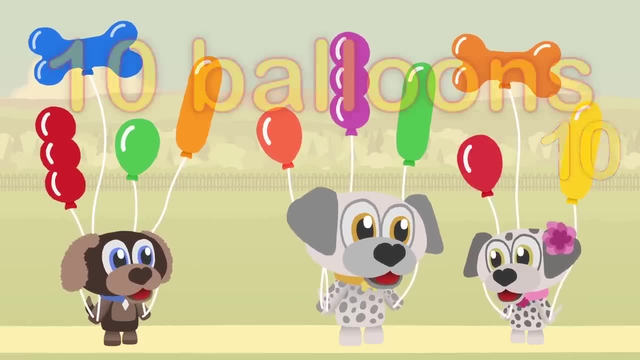 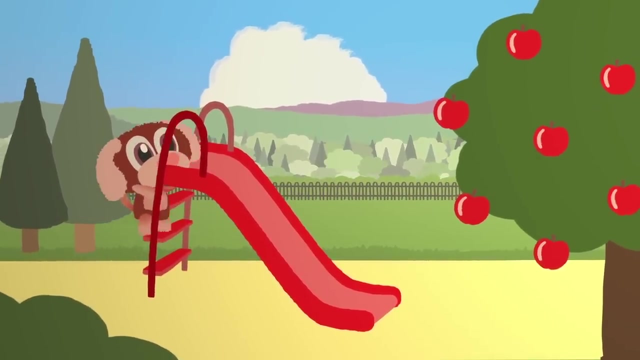 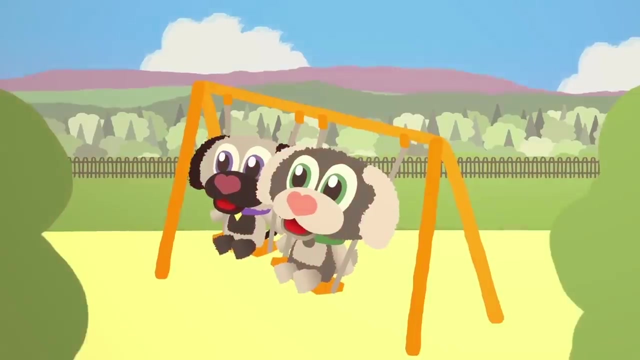 four, five, six, seven, eight, nine, ten, Ten balloons. Red Ollie is enjoying going down the red slide. Can you see anything else that's red? Oh, look, the apples in the tree are red Orange. 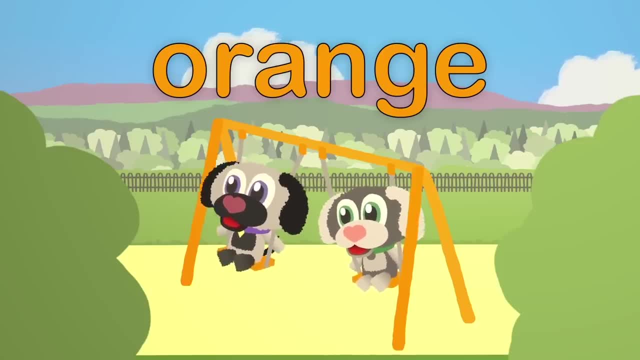 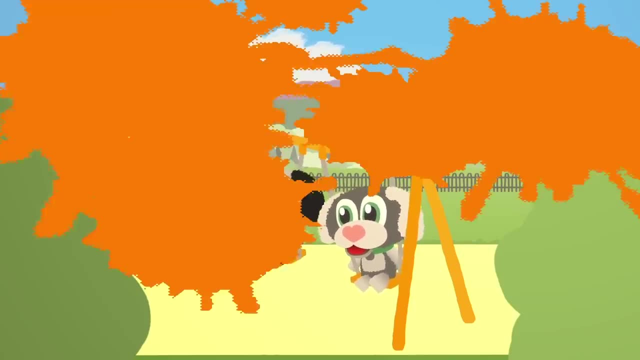 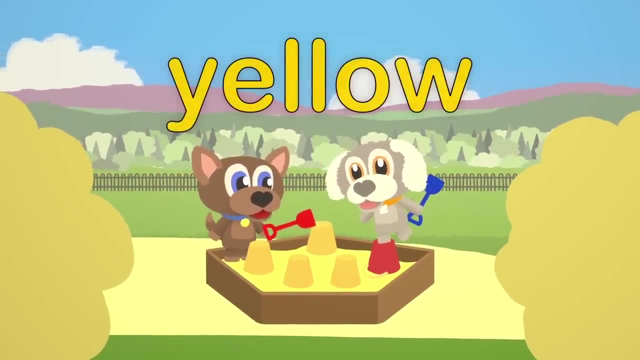 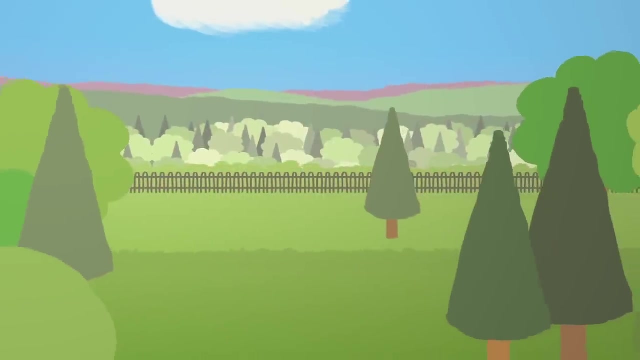 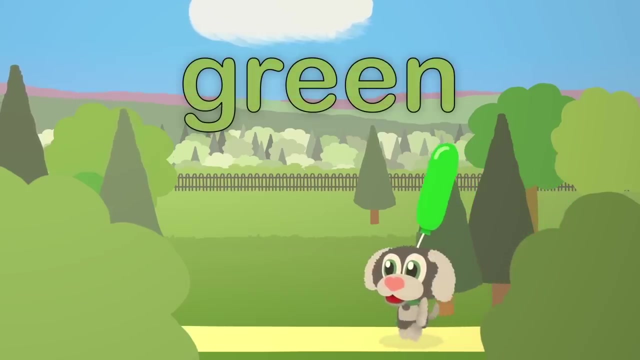 The pups are swinging high on the orange swings. Yellow Peter and Bertie are playing in the yellow sand. Silly Bertie is balancing on a bucket Green. There are lots of things in the park that are green. What can you spot? 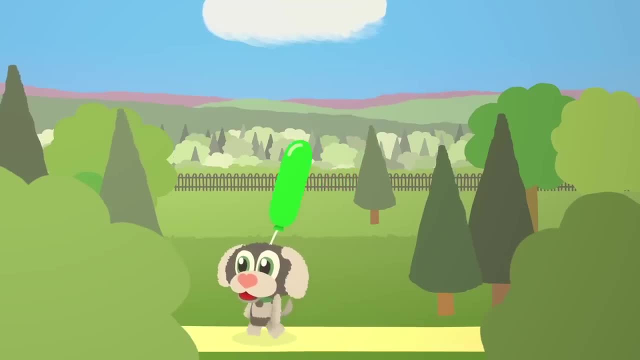 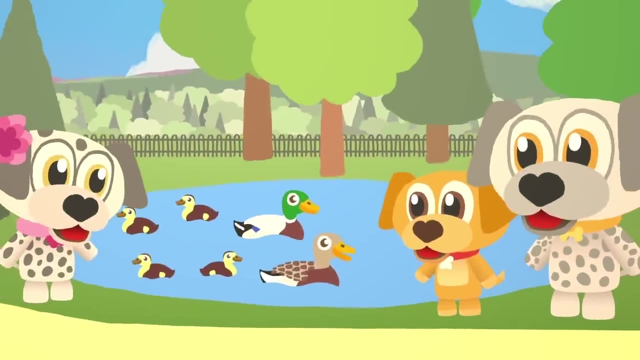 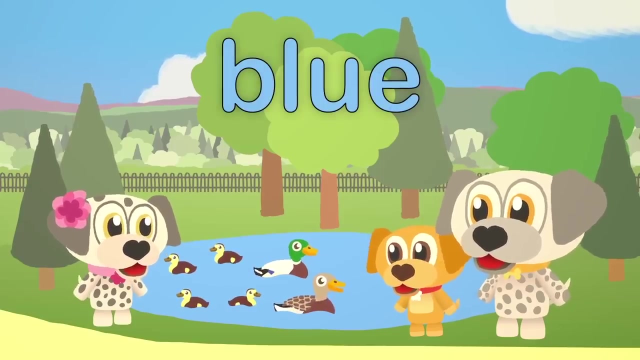 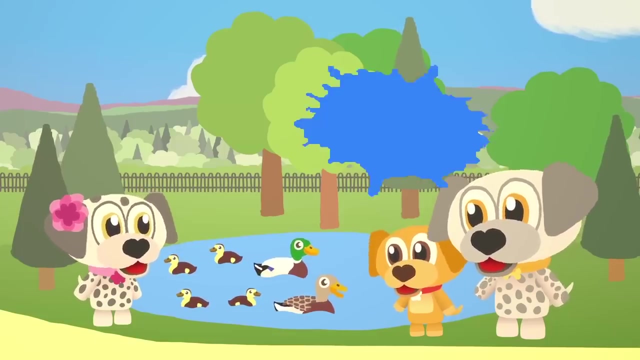 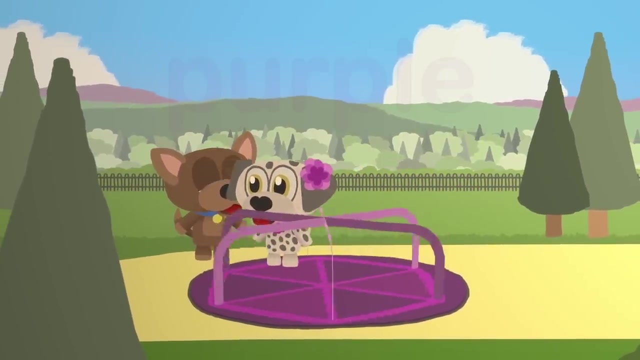 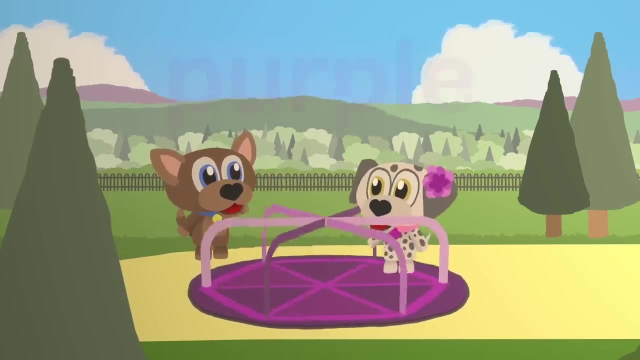 The grass, the trees and the hills Blue. It's a beautiful day. Look at the blue sky And the ducks are swimming in a blue pond. Purple Freddie is spinning Dottie on the purple roundabout- Whee, Oh. and look what colour the flower in Dottie's hair is. 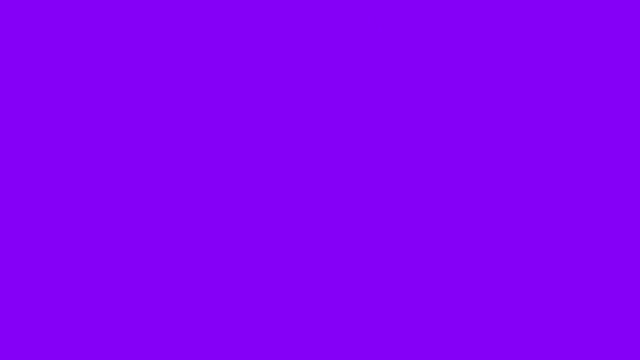 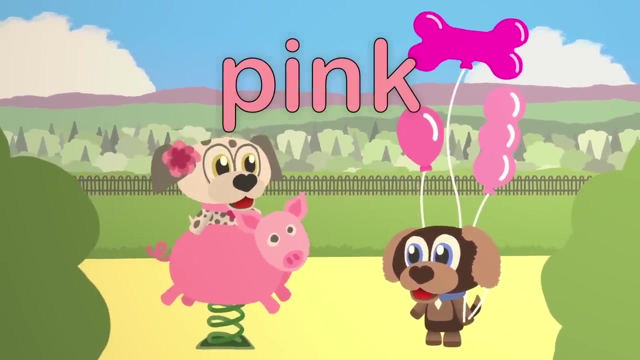 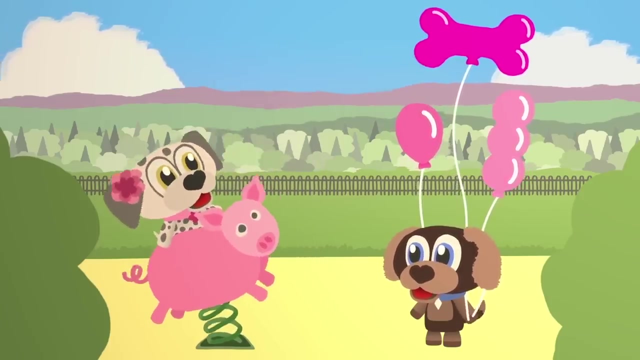 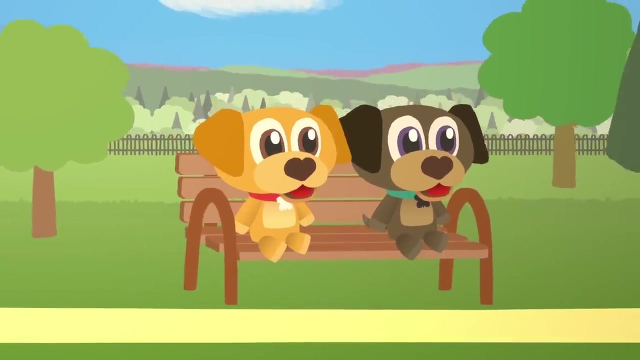 Yes, that's right, it's purple Pink. Now Dottie is enjoying rocking on the pink piggy And look at the balloons. They're pink, too Brown. The puppies are tired. It's time for a rest. The puppies are having a sit down on the brown bench. 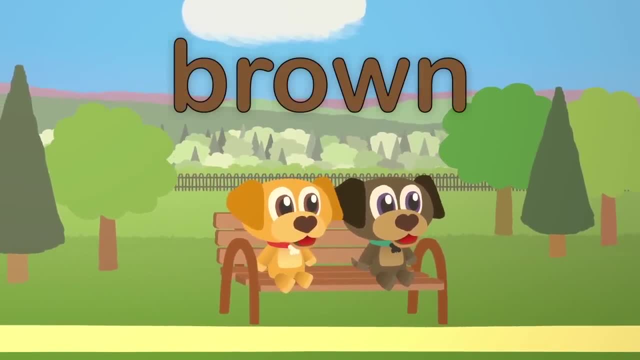 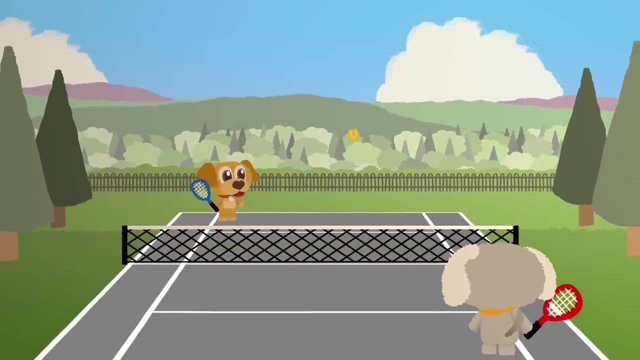 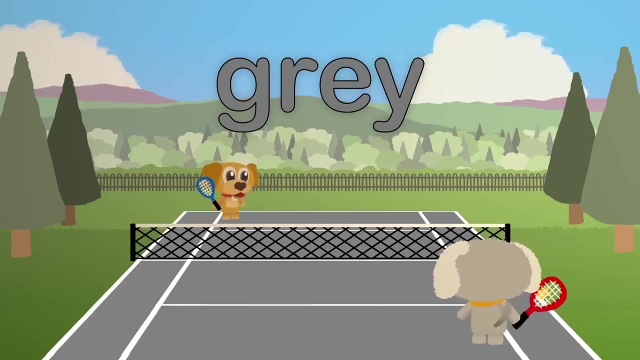 Brown. The puppies are tired. It's time for a rest. The puppies are having a sit down on the brown bench: Brown Brown, Brown, Brown Brown, si style Grey. Two of the pups are playing a game of tennis. 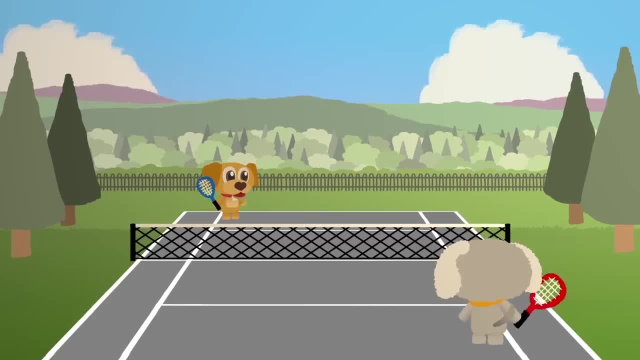 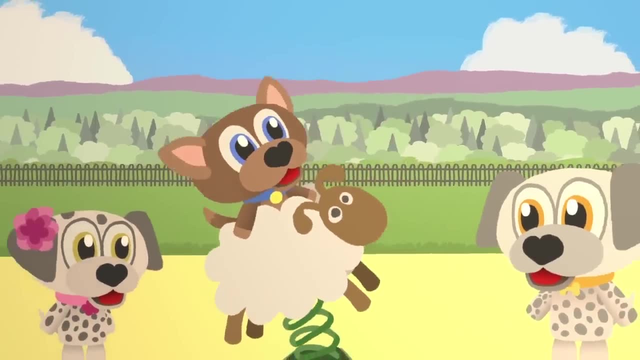 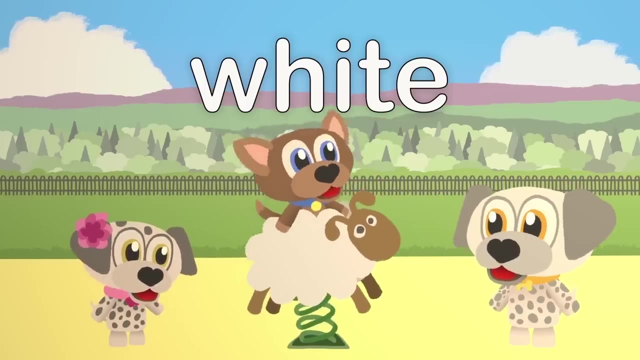 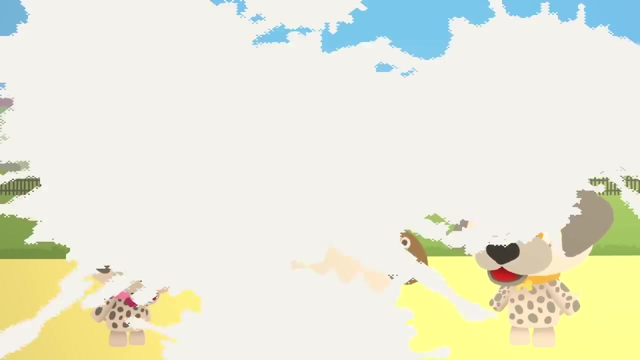 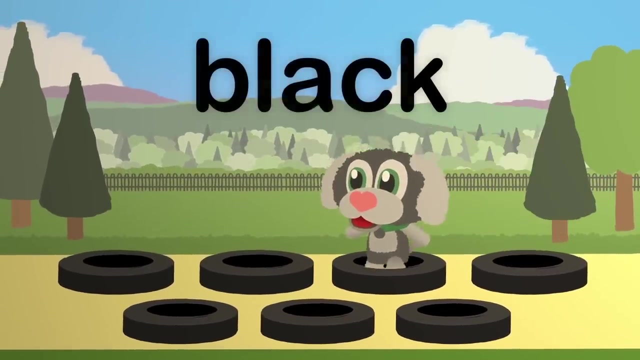 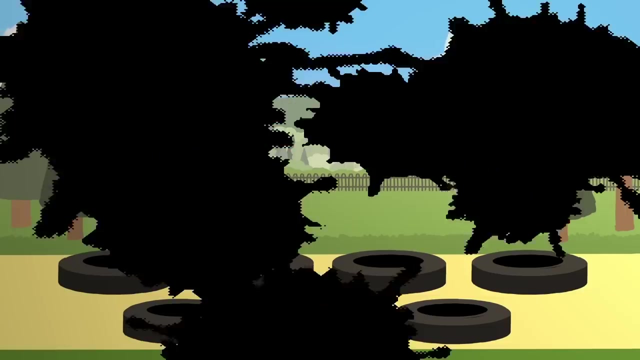 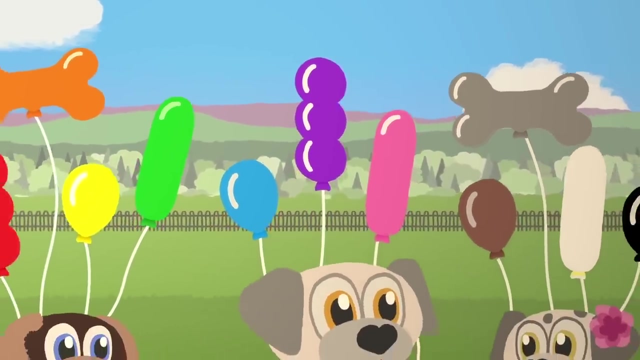 The tennis court is grey. White is riding on the white sheep. Dottie and Grandpa Dog have white fur. Black Jumping in the tyres looks lots of fun. Careful not to trip. Look at all the colourful balloons. Can you spot the colours we've seen today? 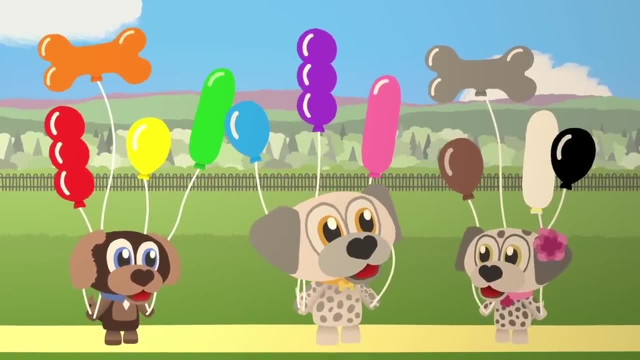 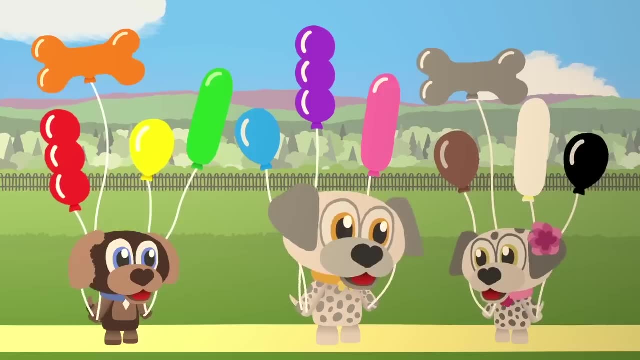 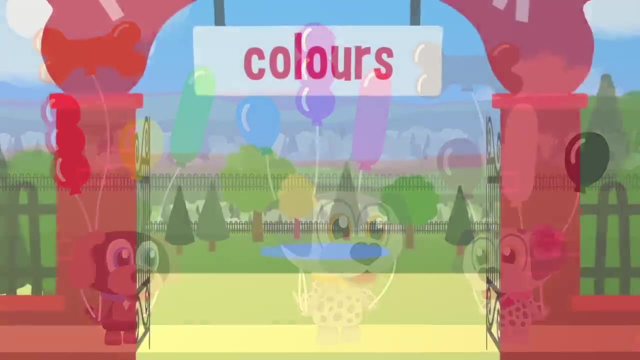 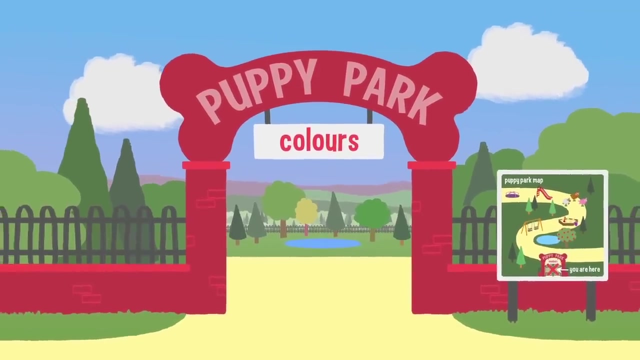 Red, orange, yellow, green, blue, purple, pink, brown, grey, white and black. What's your favourite colour? It's time to leave Puppy Park now. We hope you've enjoyed it. We hope you've enjoyed finding colours with us today. Come back and visit again soon. 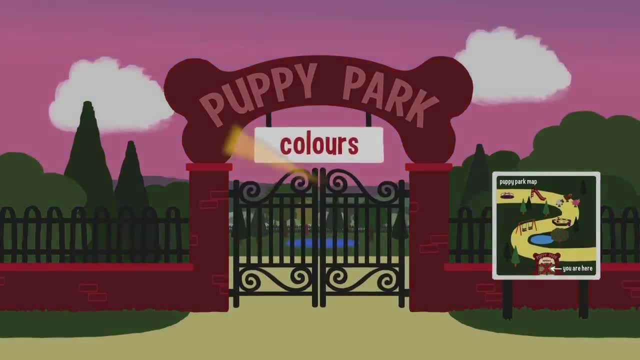 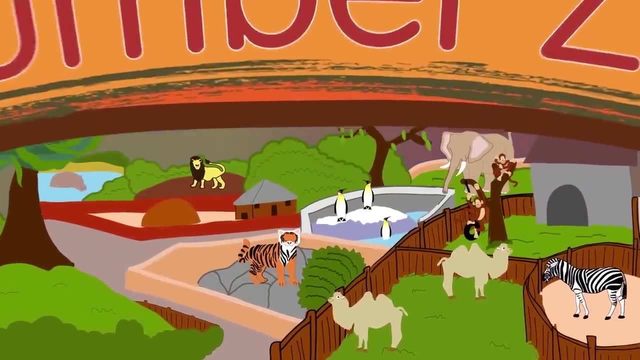 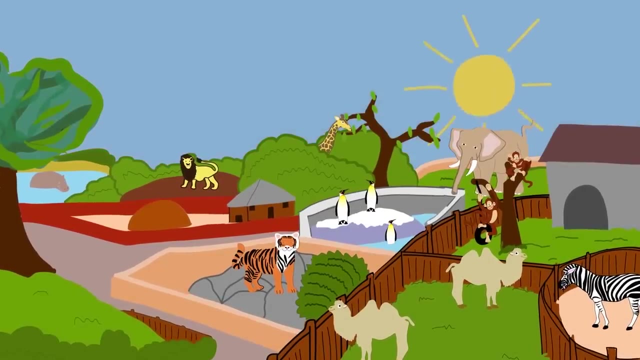 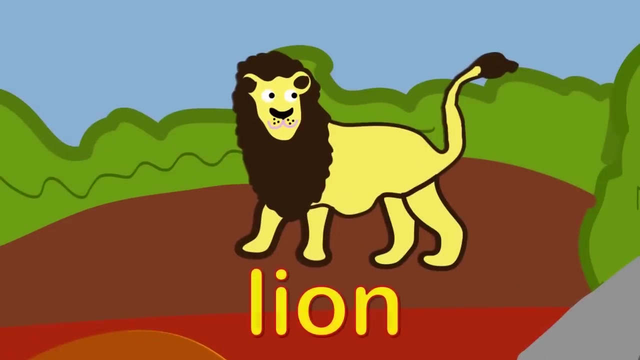 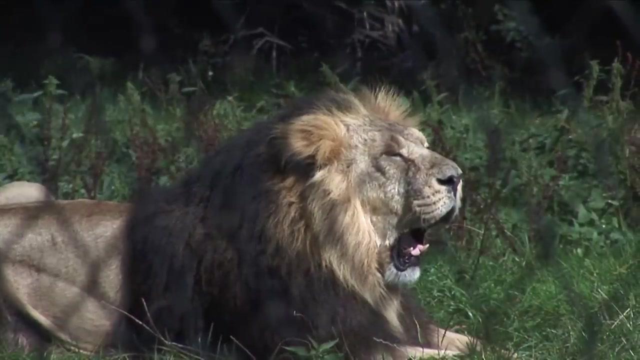 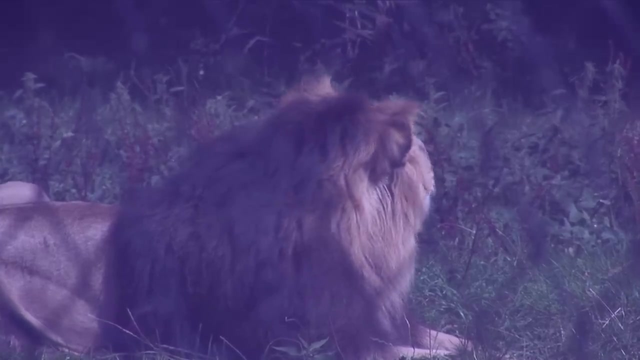 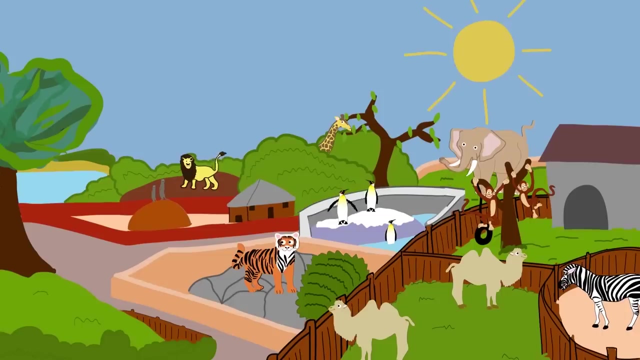 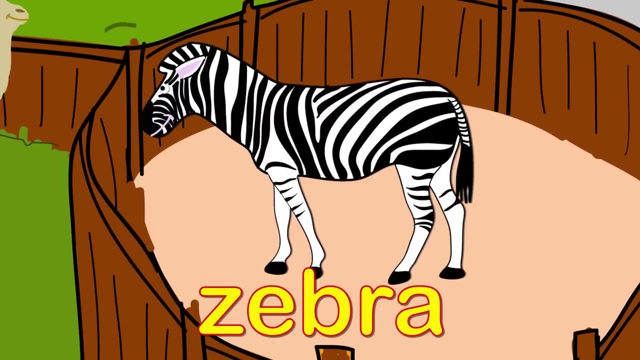 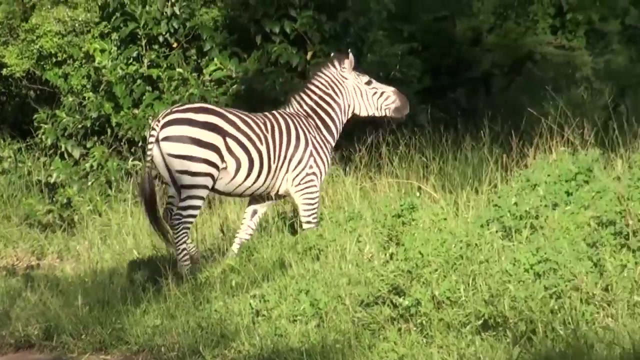 Bye, bye, Welcome to Number Zoo. Good morning animals. It's time to wake up. Wakey, wakey. Hello furry lion. One one lion. Daffodils. Hi fur synths Daffodils. Hello Stripey Zebra. 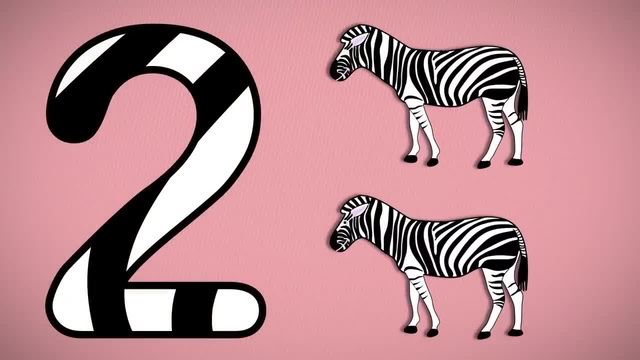 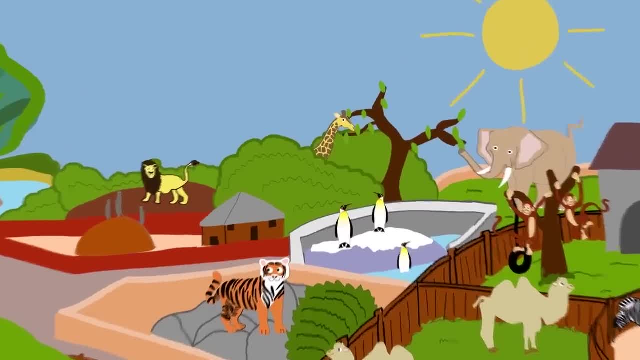 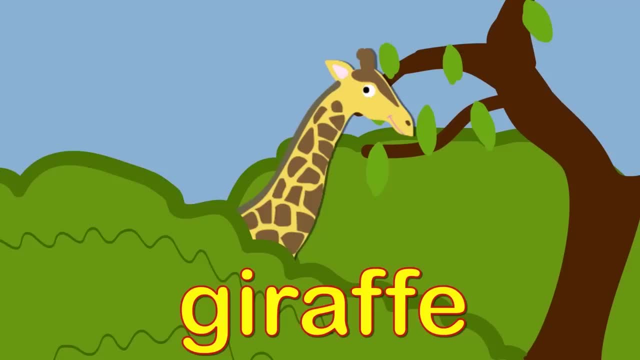 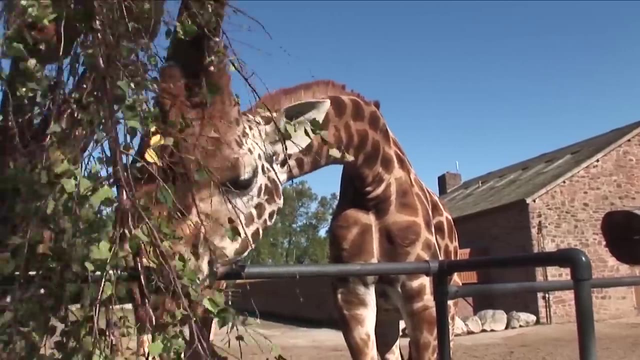 One, Two, Three, Four, Five, Six, Seven, Eight Nine, 10, 11, 12, 13, 14, 15, 16, 17, 18, 19, 20, 21, 22, 23, 24, 25, 26, 27, 28, 29, 30. 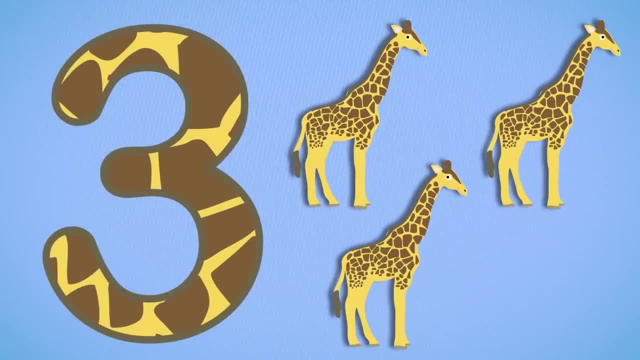 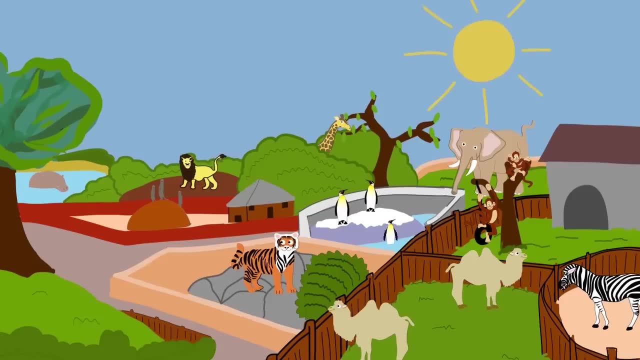 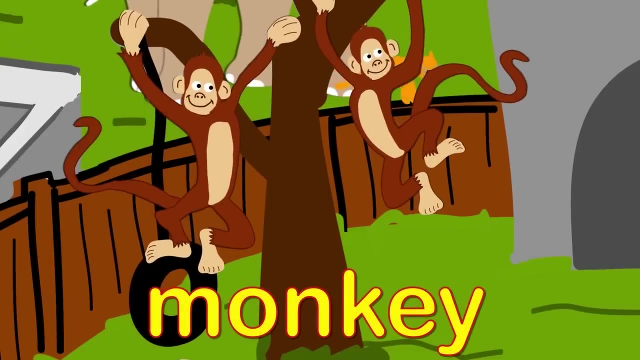 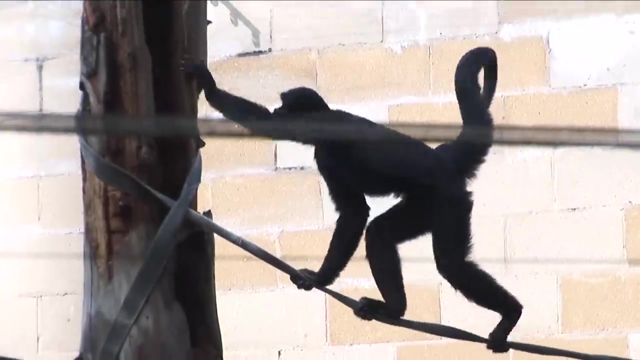 31, 32, 33, 34, 35, 36, 37, 38, 39, 40, 41, 42, 43, 44, 45, 46, 47, 48, 49, 50, 51, 52, 53, 54, 55, 56. 57, 58, 59, 60, 61, 62, 63, 64, 65, 67, 68, 69, 70, 71, 72, 73, 74, 75, 76, 77, 78, 79, 80, 81, 82, 83. 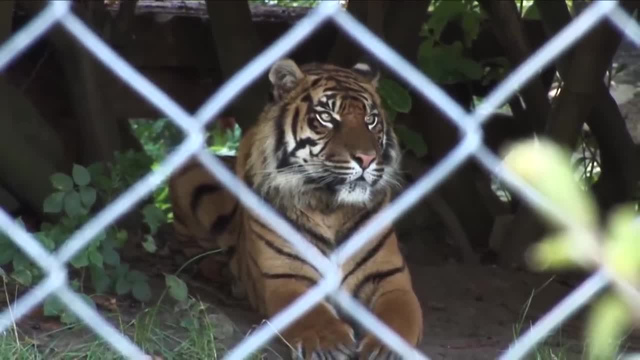 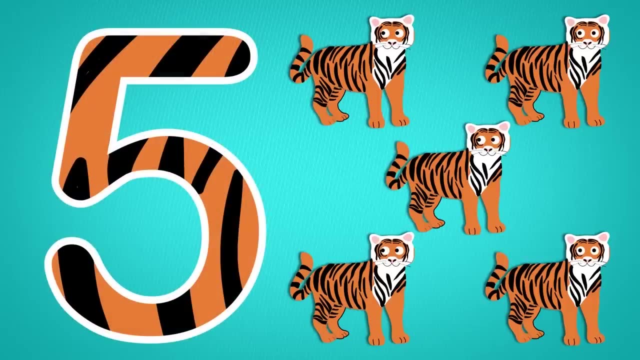 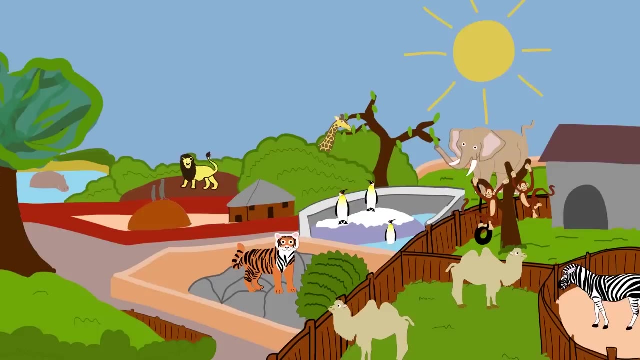 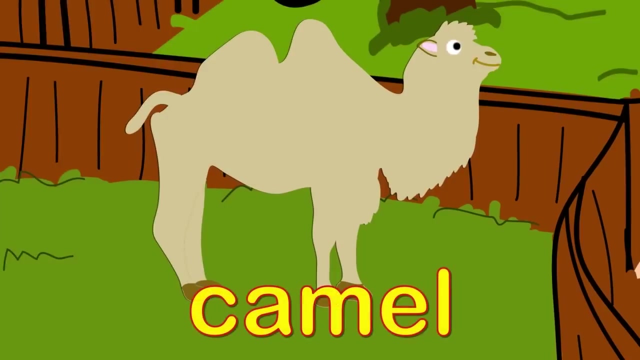 84, 85, 86, 87, 88, 89, 90, 92, 93, 93, 93, 94, 95, 96, 97, 98, 98, 99, 100, 100, 12, 23, 23, 24, 25, 26. 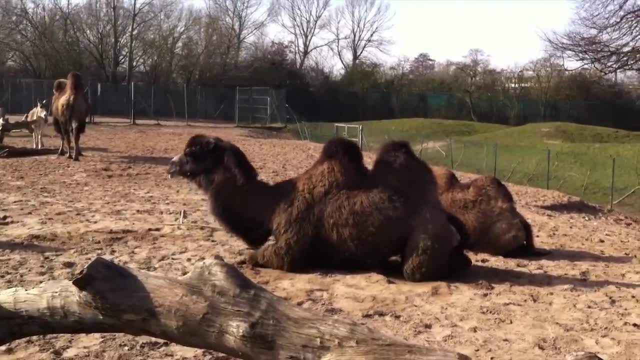 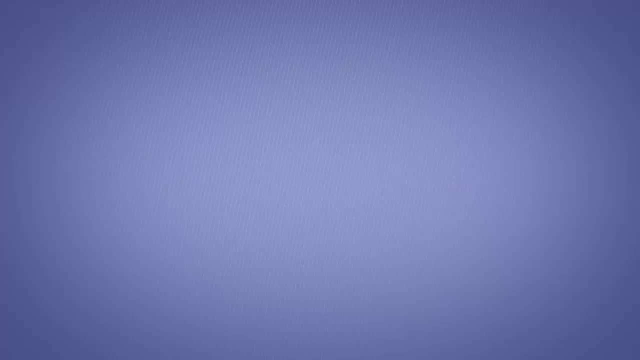 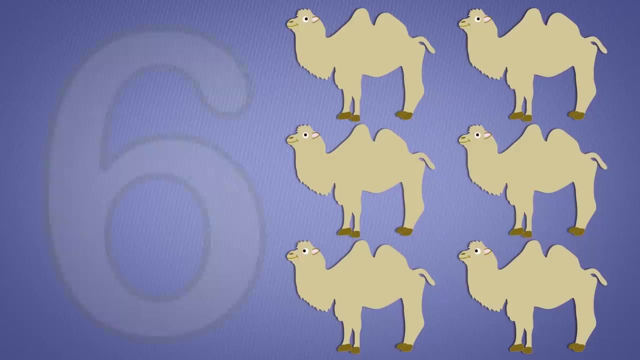 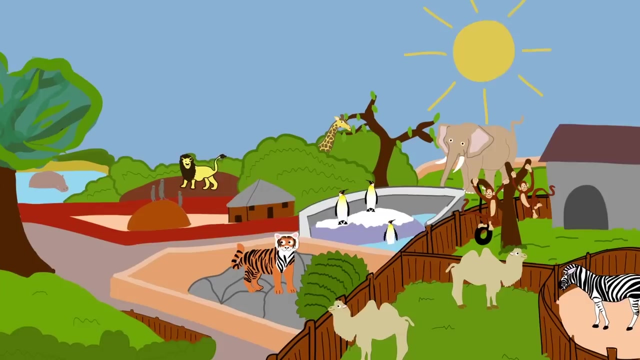 26, 27, 28, 29, 30, 31, 32, 33, 33, 34, 35, 36, 36, 37, 38, 39, 40, 41, 42, 43, 44, 45, 46, 47, 48, 49. 50, 51, 52, 53, 53, 54, 55, 56, 57, 58, 59, 60, 61, 62, 63, 62, 63, 64, 65, 67, 68, 68, 69, 69, 70, 71. 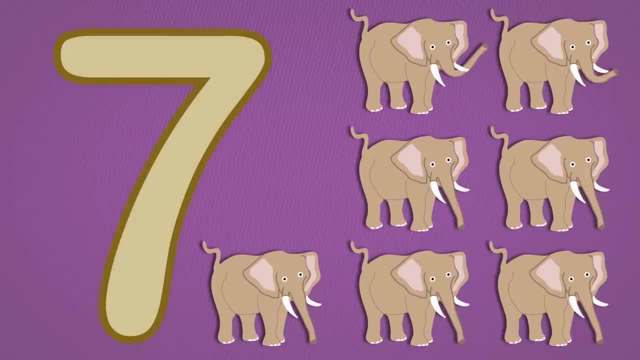 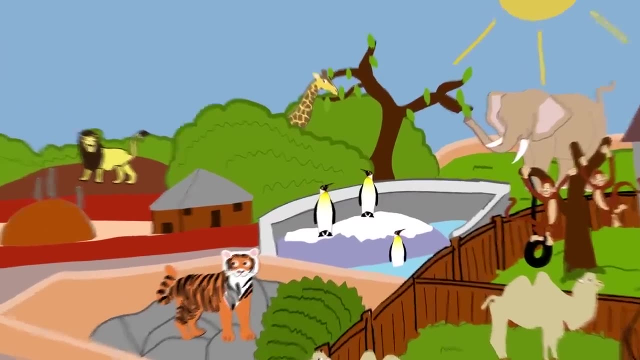 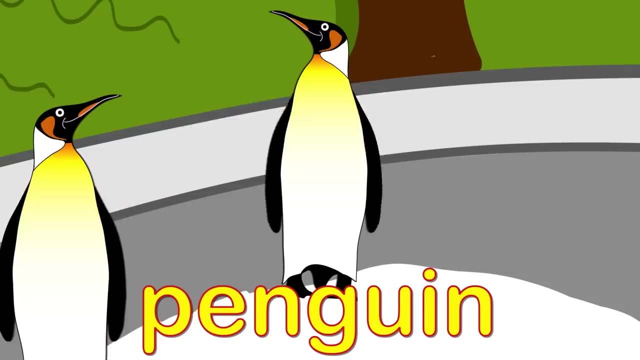 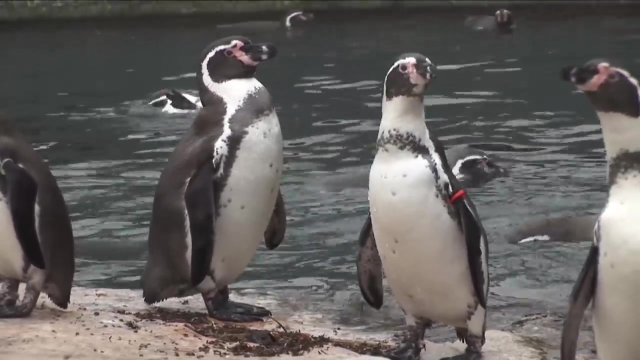 72, 73, 74, 75, 76, 76, 77, 78, 79, 80, 81, 82, 83, 84, 85, 86, 87, 86, 87, 88, 88, 89, 90, 91, 92, 93. 93, 94, 95, 96, 97, 97, 98, 99, 100, 100, 12, 13, 14, 15, 16, 17, 18, 19, 20, 22, 23, 24, 25, 26, 27, 28. 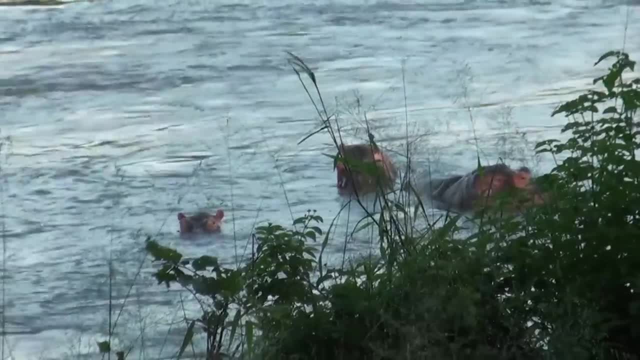 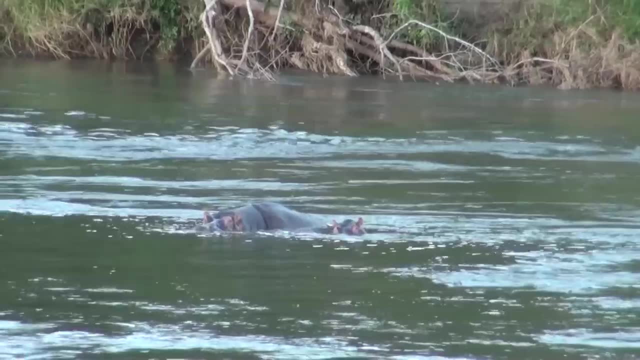 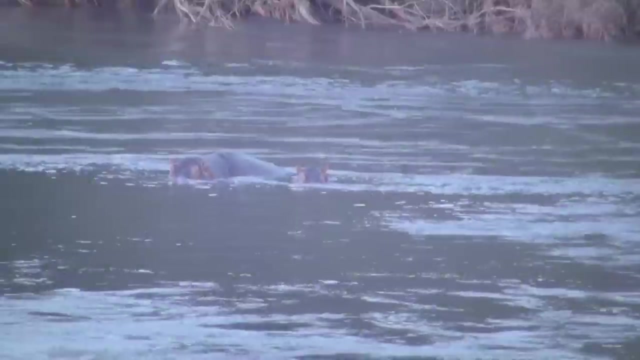 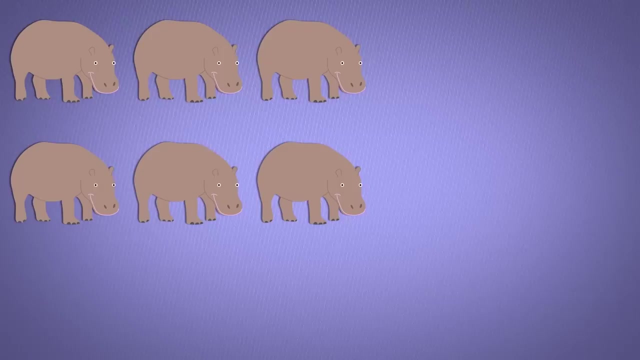 29, 30, 31, 32, 33, 34, 35, 36, 37, 38, 39, 40, 41, 42, 43, 44, 45, 46, 47, 48, 49, 50, 51, 52, 53, 53. 54, 55, 56, 57, 58, 59, 60, 61, 62, 63, 63, 64, 65, 66, 67, 68, 69, 70, 71, 72, 73, 74, 75, 76, 76, 77. 78, 79, 79, 80, 80, 81, 82, 83, 84, 85, 86, 87, 88, 89, 90, 91, 92, 93, 94, 95, 96, 97. 0 0, 0 0. 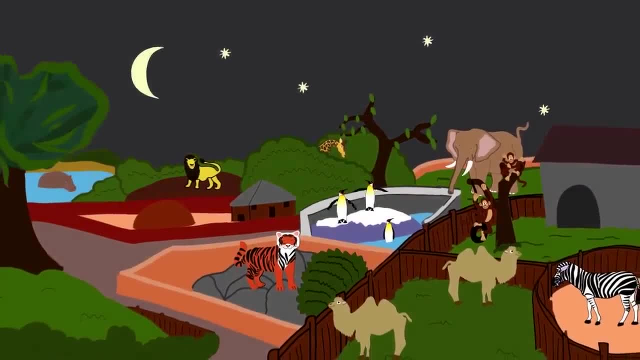 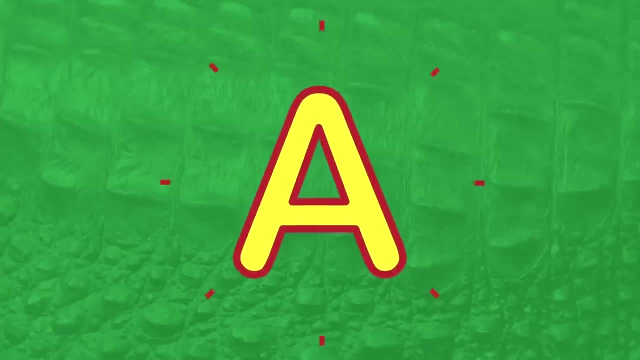 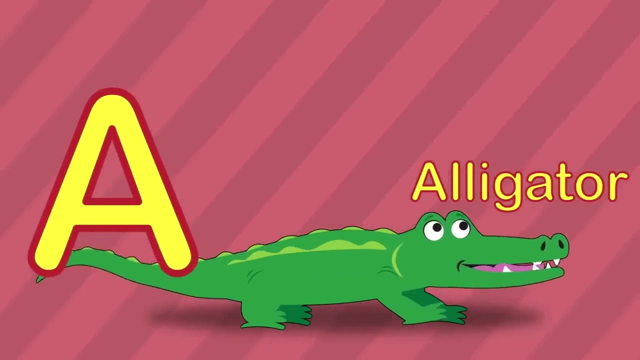 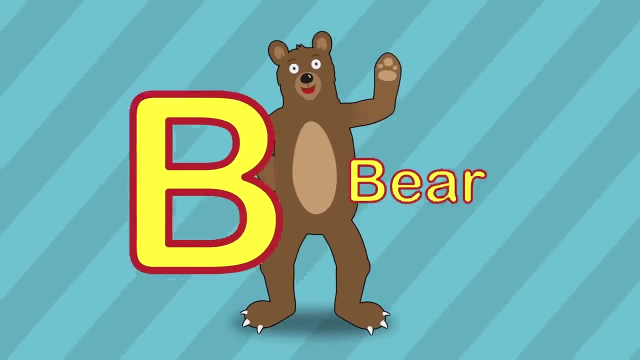 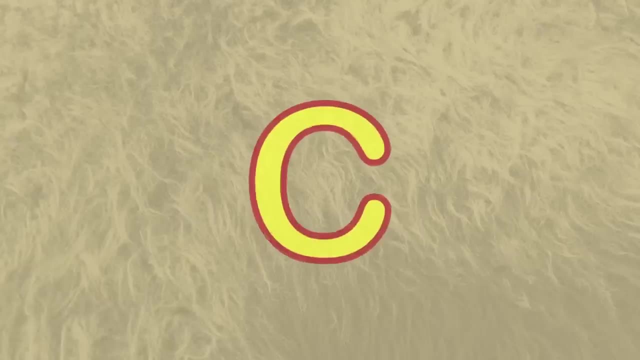 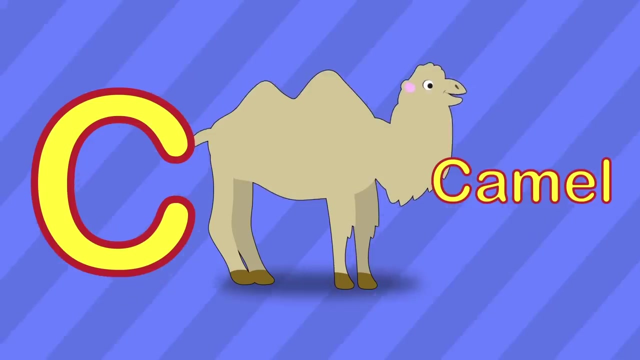 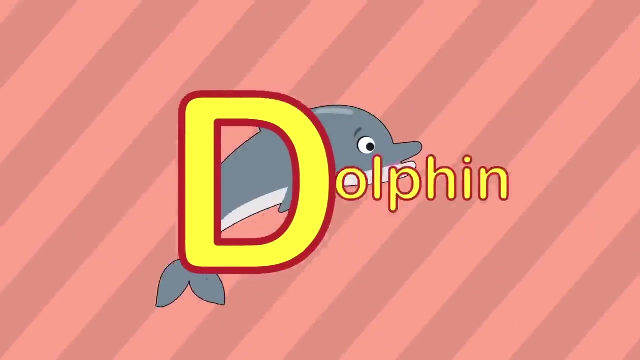 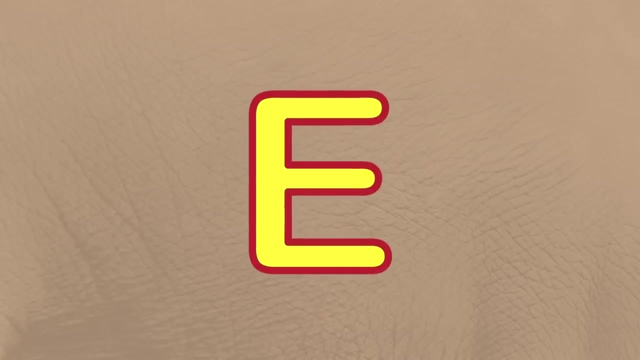 0, 0, 1, 3, 1 1 2021, 2021, 2021. 2, 2, 3, 2, 4, 3, 4, 4, 5, 6, 5, 6 D. D is for Dolphin E- E is for Elephant. 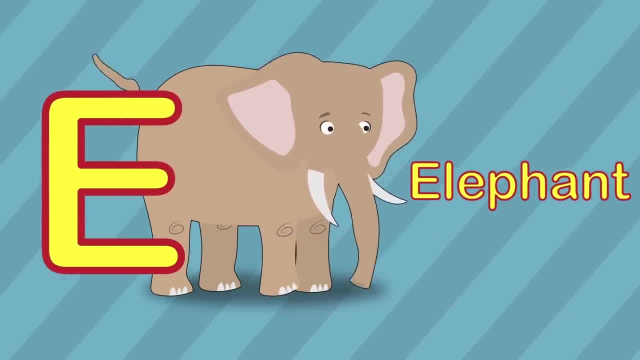 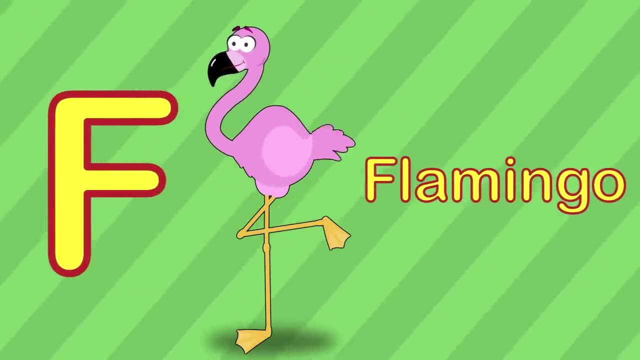 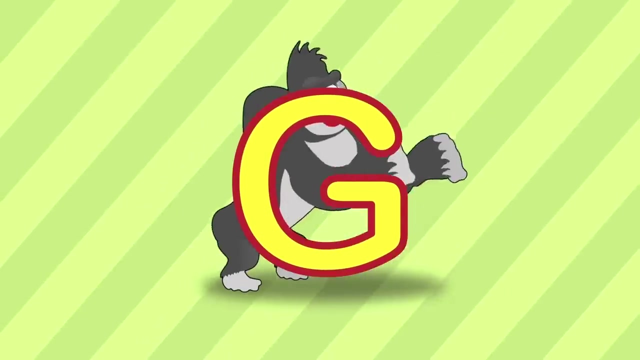 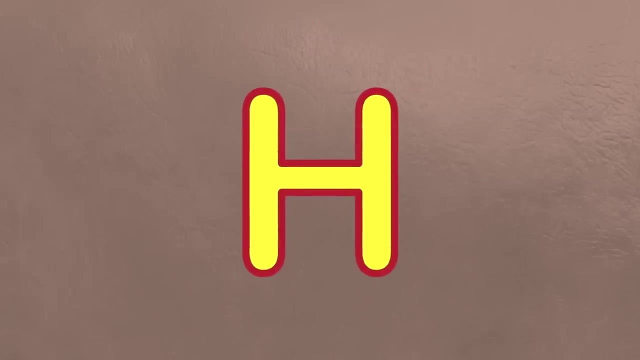 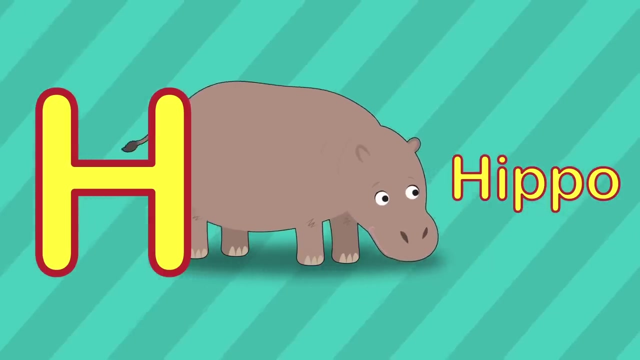 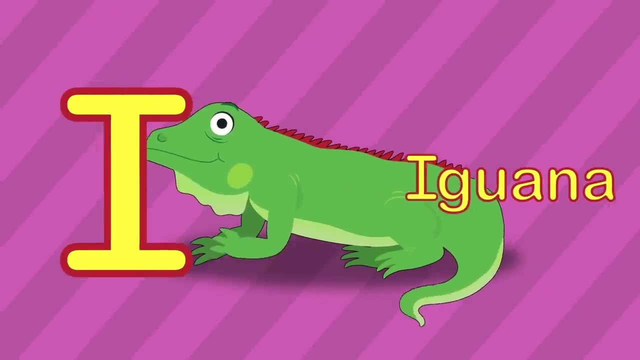 F. F is for Flamingo, G, G is for Gorilla, H, H is for Hippo, I. I is for Iguana Z ZZ, Z, Iguana, ZZ, Iguana. What LX, What LX, Whatютo, Whatageo, Whatageo. 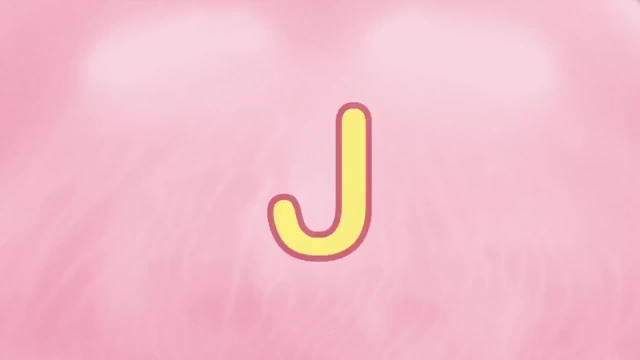 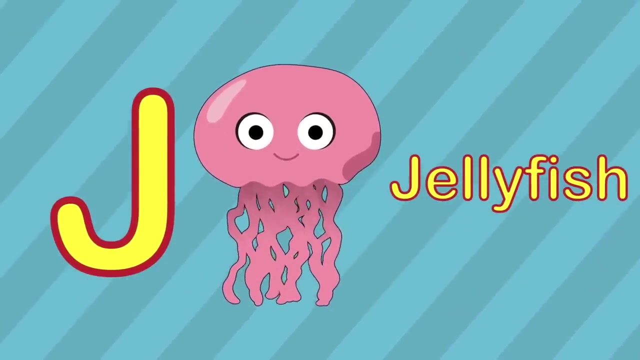 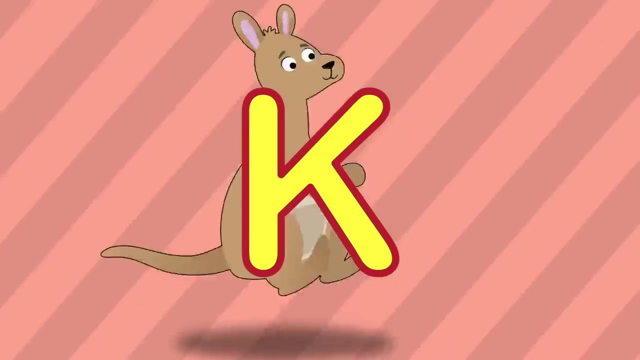 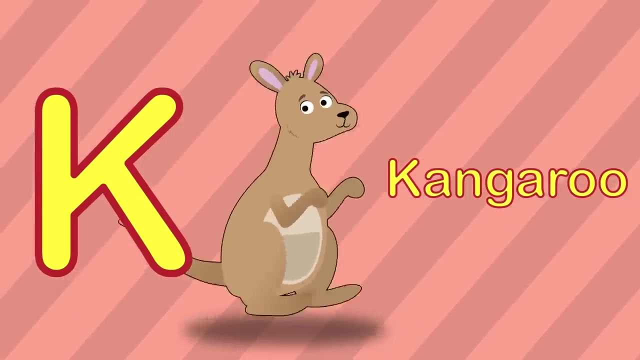 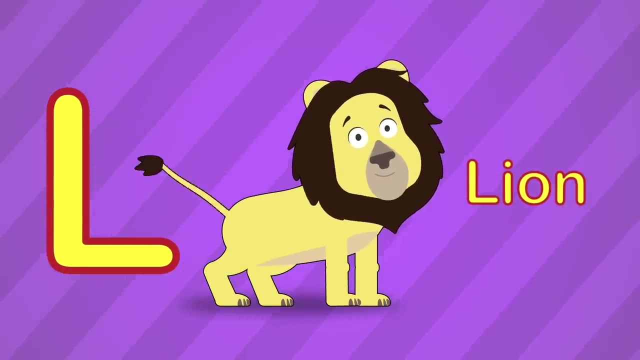 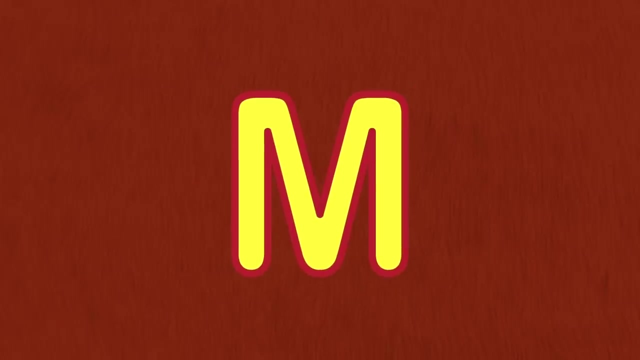 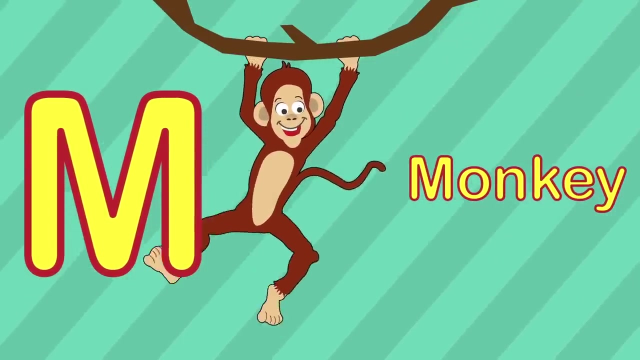 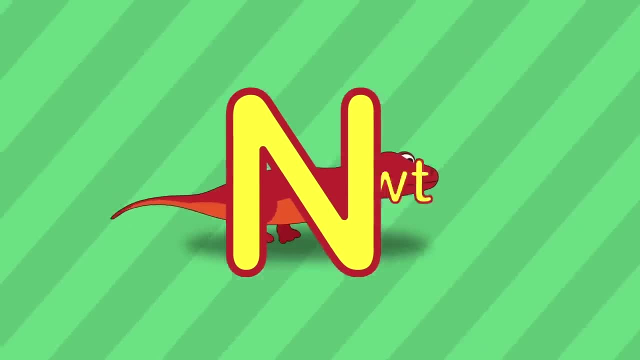 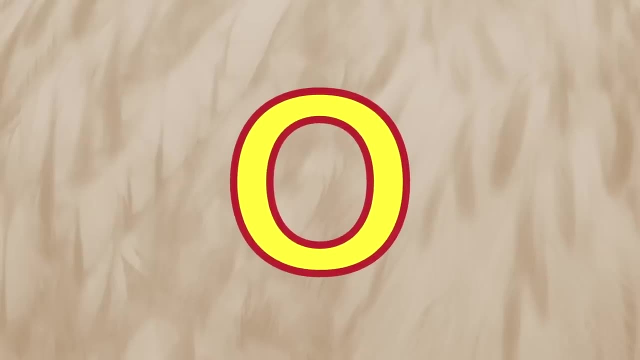 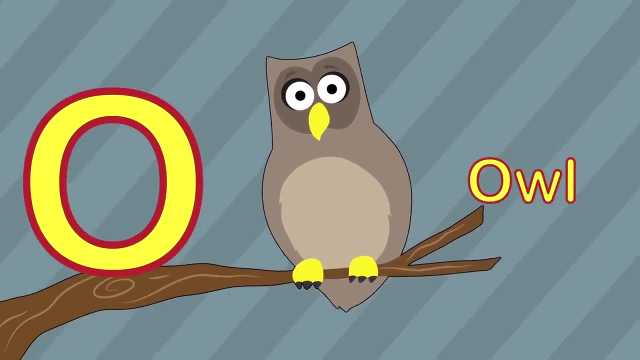 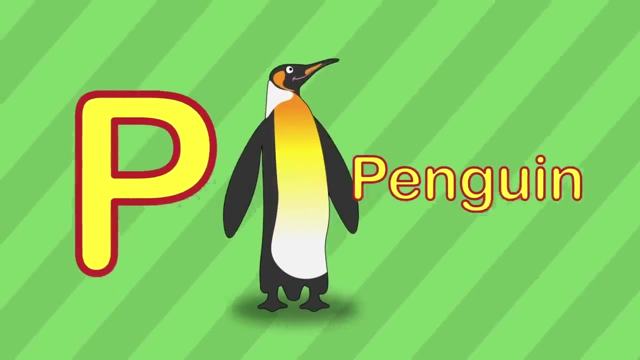 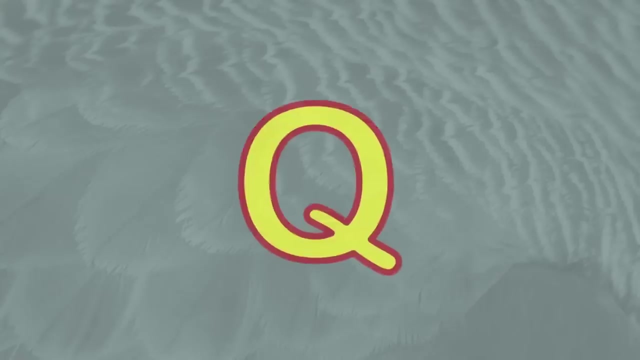 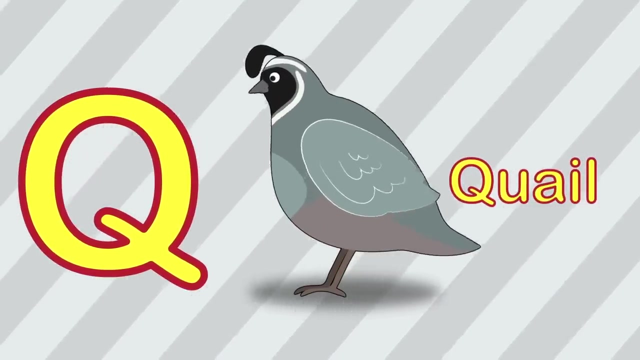 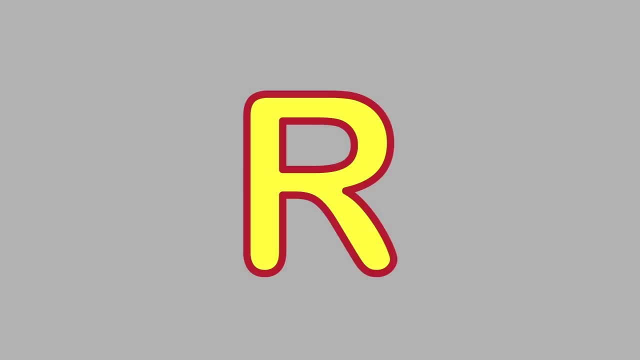 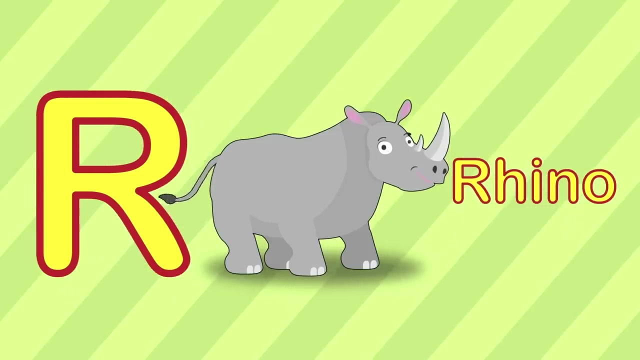 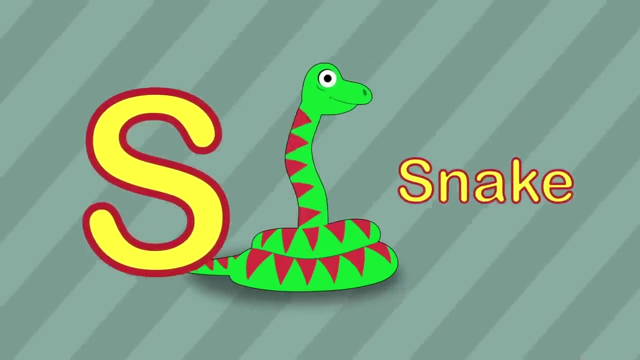 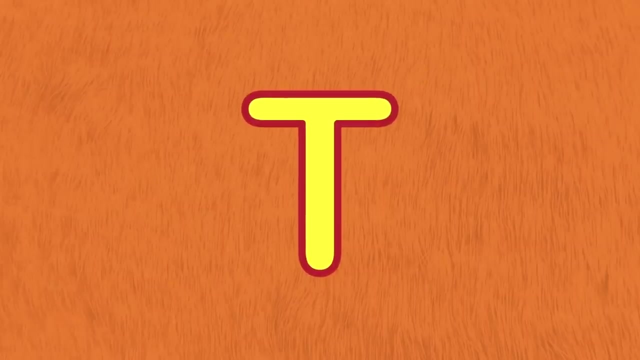 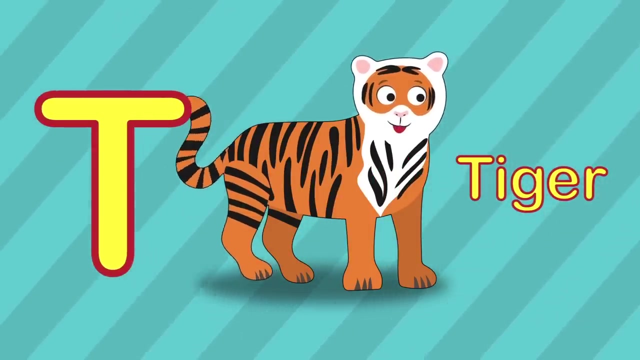 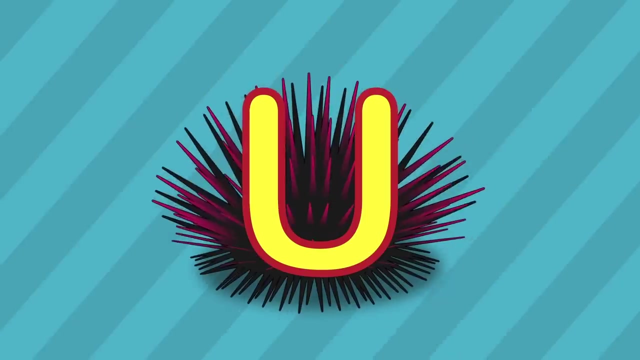 M. M is for Monkey, N, N is for Newt, O, O is for Owl, P, P is for Penguin, Q, Q is for Quail, R, R is for Rhino, S, S is for Snake, T, T is for Tiger, U. U is for Urchin. 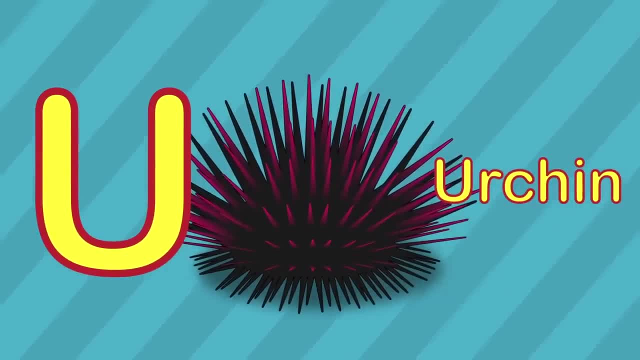 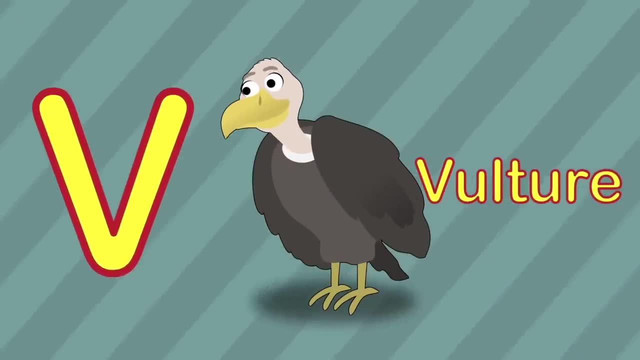 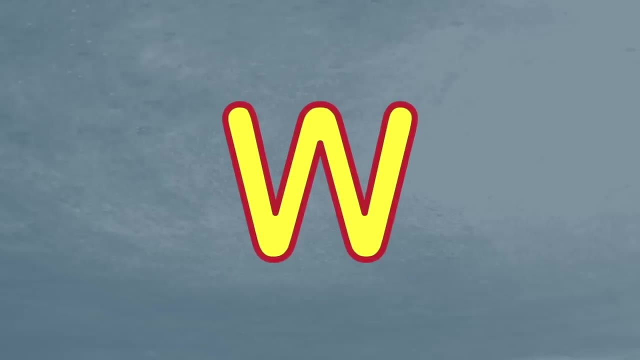 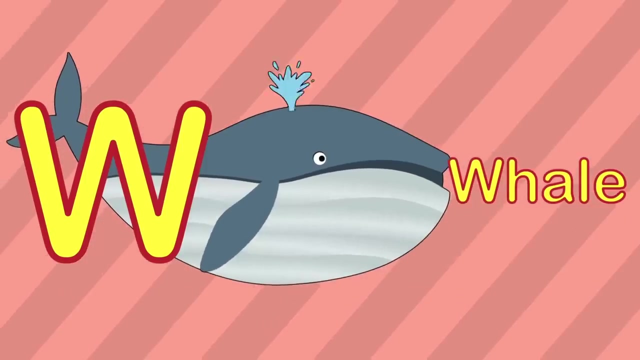 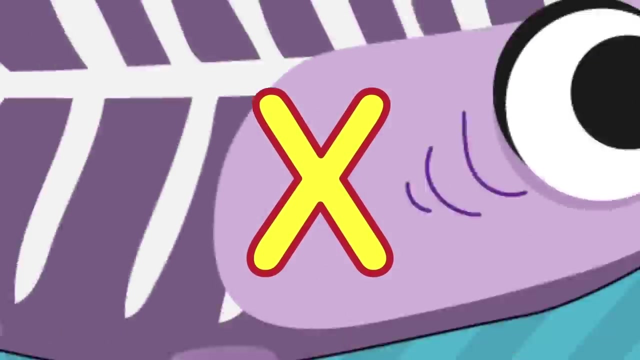 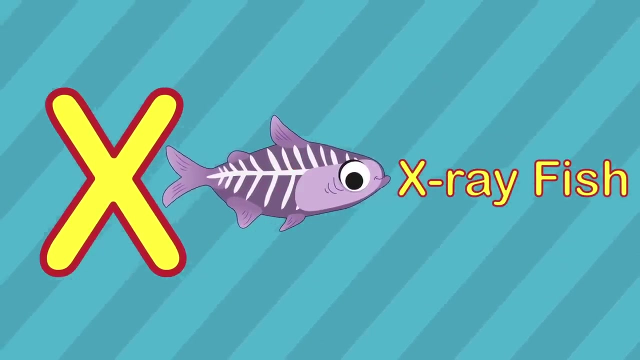 S. S is for Snake S. S is for Snake S. S is for Snake V, V is for Vulture, W, W is for Whale X, X is for Fox S. S is for Fox S. S is for Fox X. X is for X-Ray Fish. 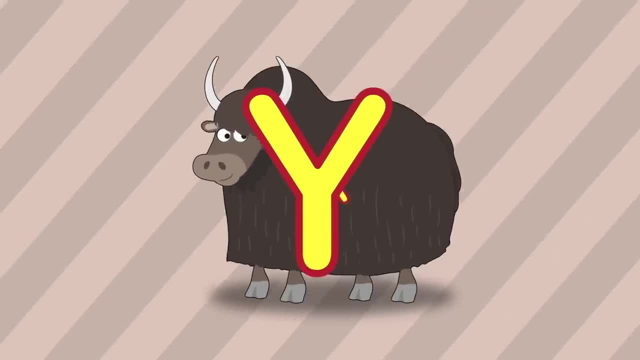 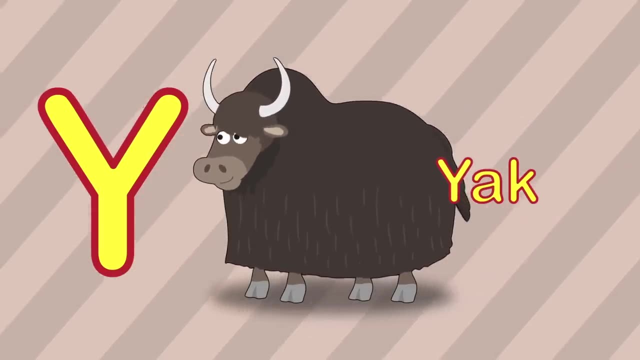 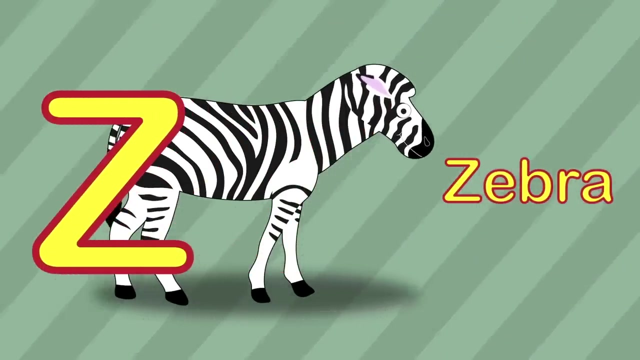 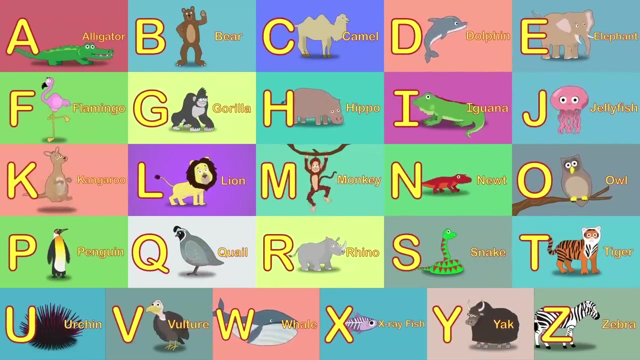 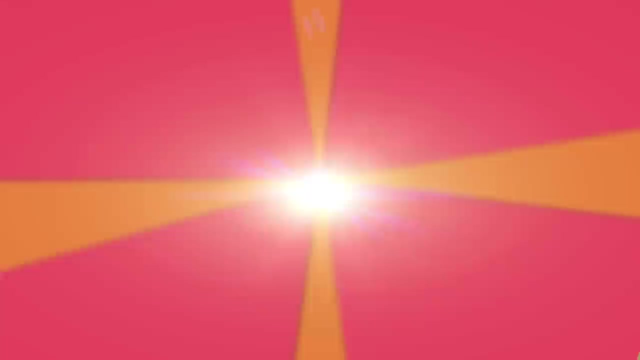 Y. Y is for Yak and Z Z is for Zebra and Z? Z is for Zebra. Thanks for learning Animal ABC with us. See you again next time. Welcome to Puppy Park. It's Alphabet Day here at the park. The pups are learning some new words. Would you like to join in? 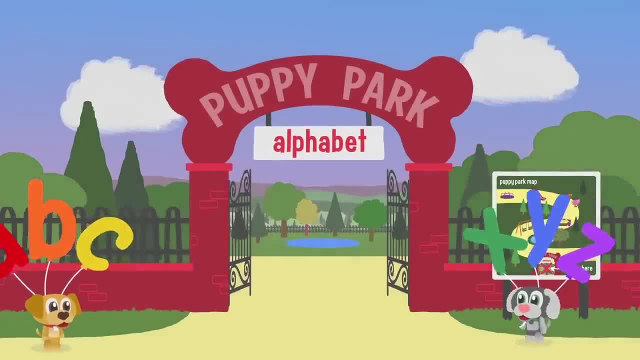 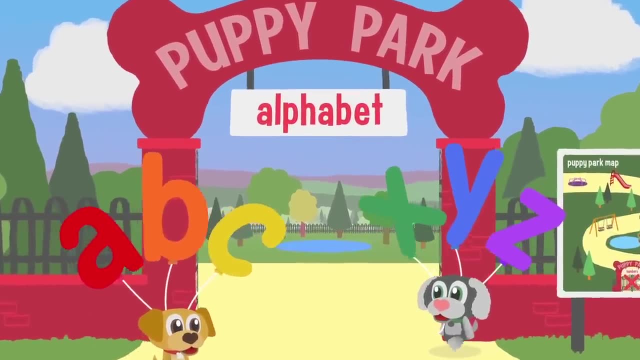 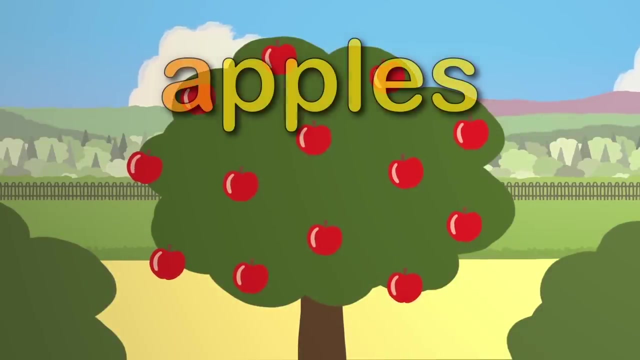 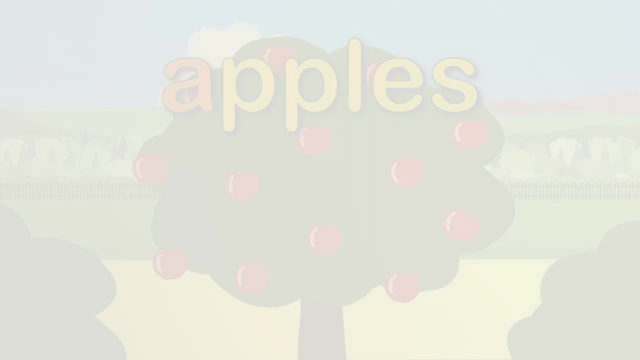 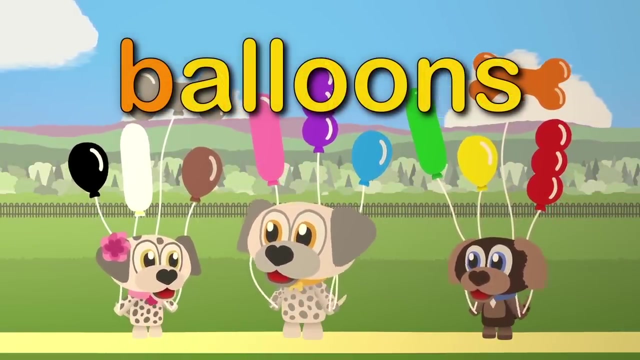 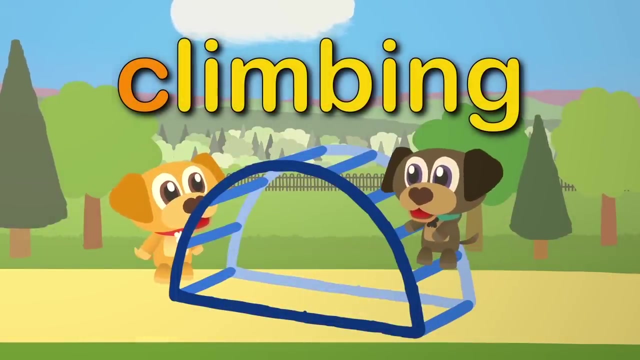 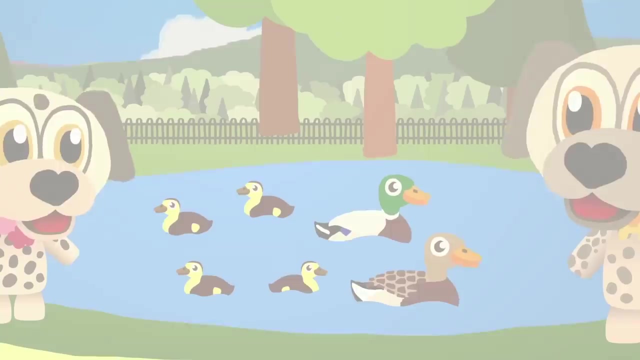 Welcome to Puppy Park. It's Alphabet Day here at the park. The pups are learning some new words. Would you like to join in? A is for Apples, A is for Apples, B is for Balloons, C is for Climbing, D is for Ducks. 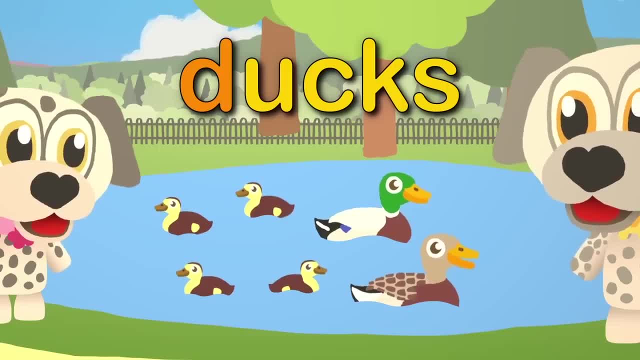 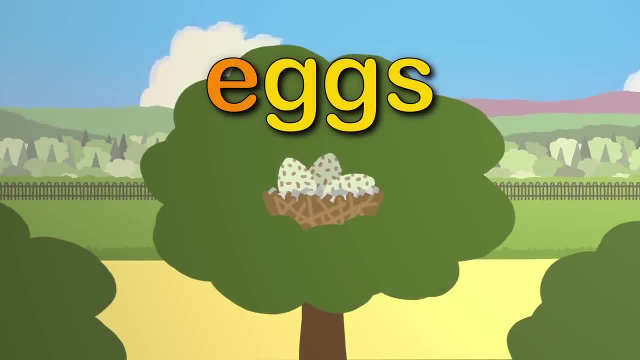 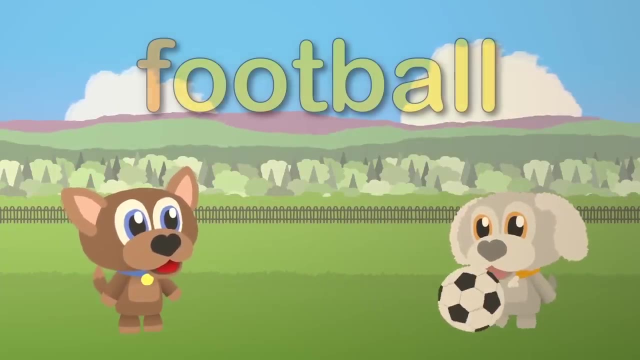 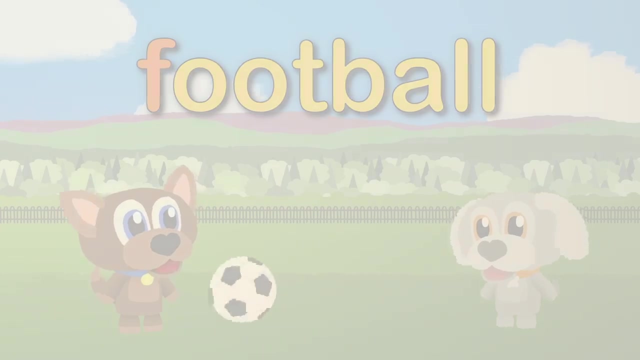 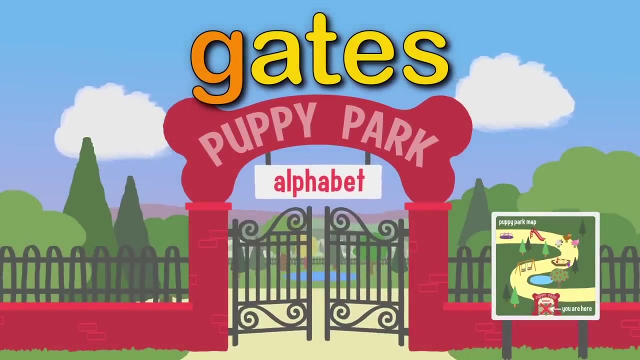 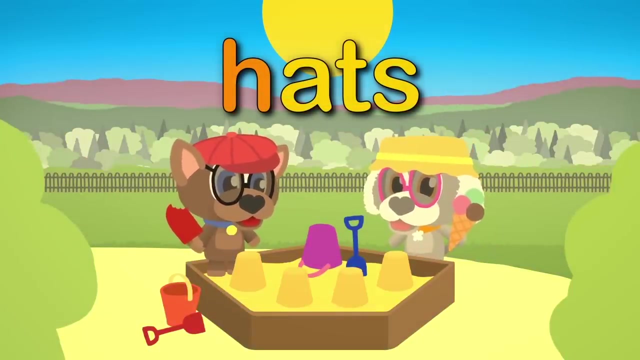 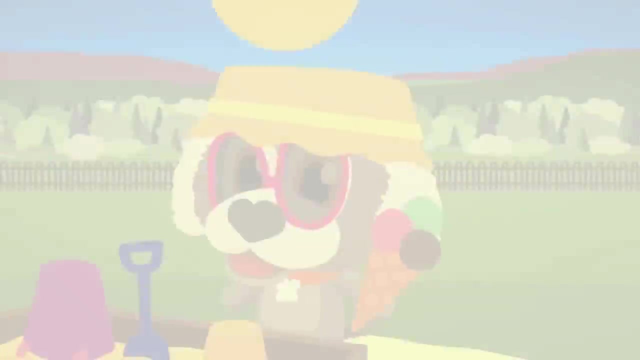 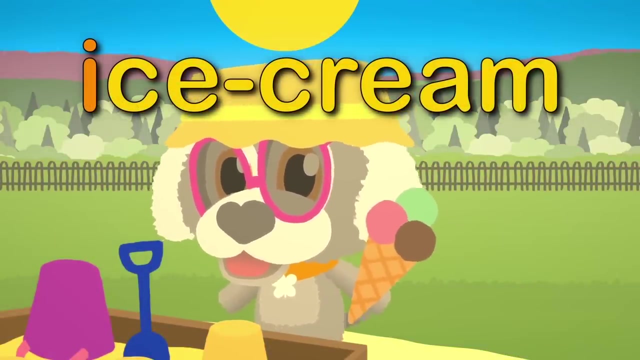 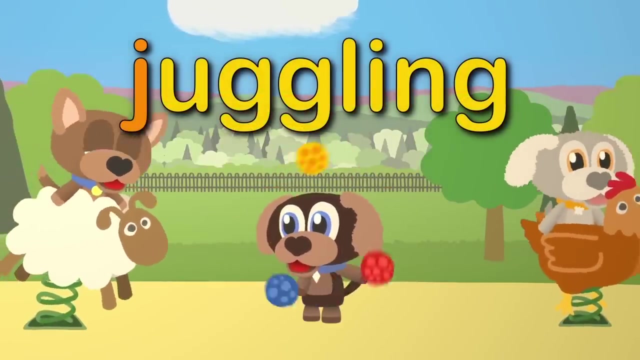 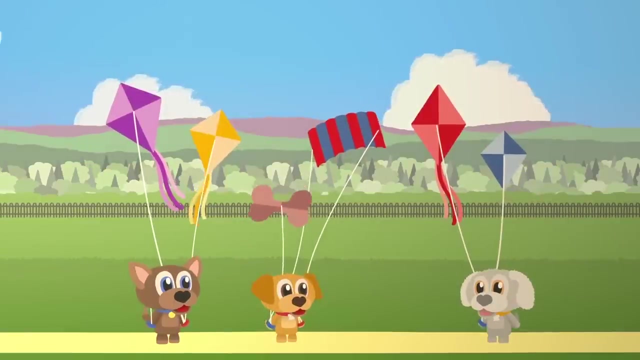 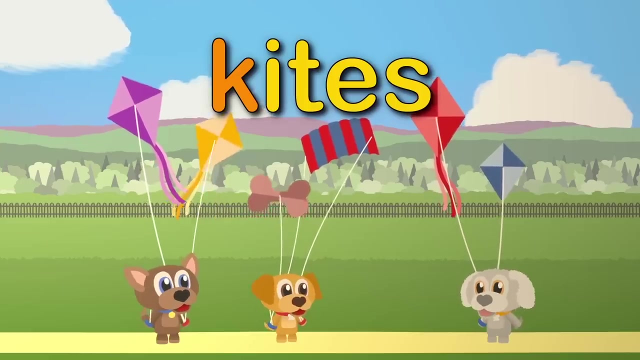 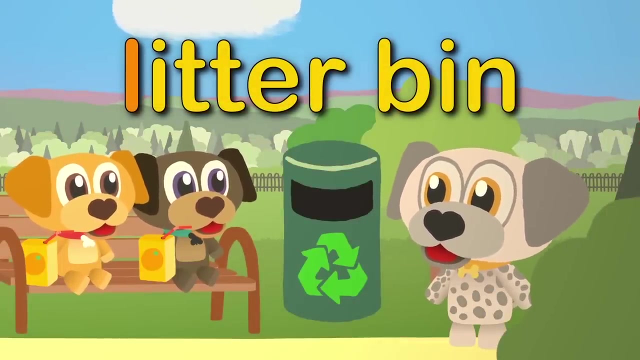 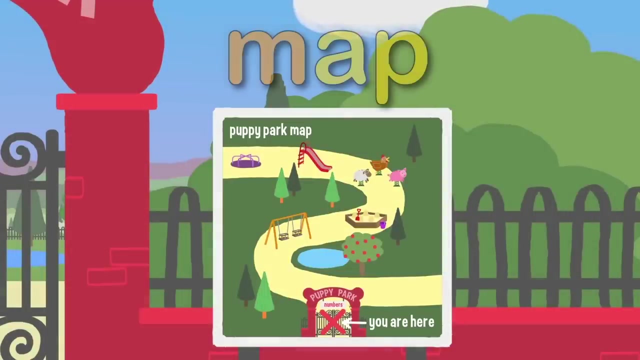 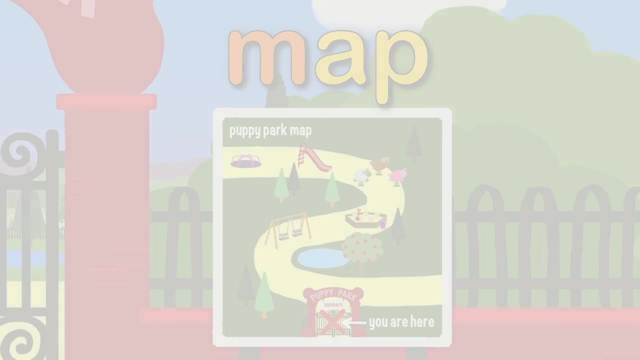 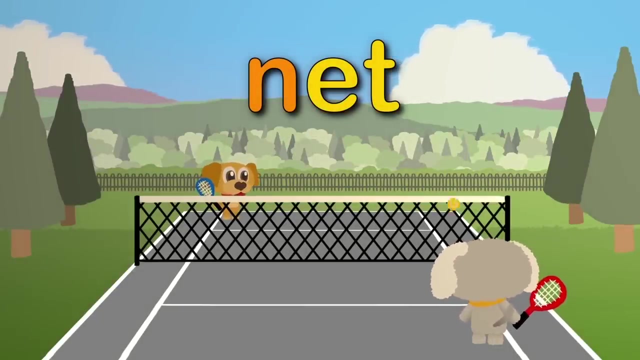 Ducks Ducks. E is for Eggs Ducks, Ducks Ducks. F is for Football Football, Football Football. G is for Gates. G is for Gates For Gates, H for Hats, I for Ice Cream, J for Juggling, K for Kites, L for Litter Bin, M for Map, N is for Net. 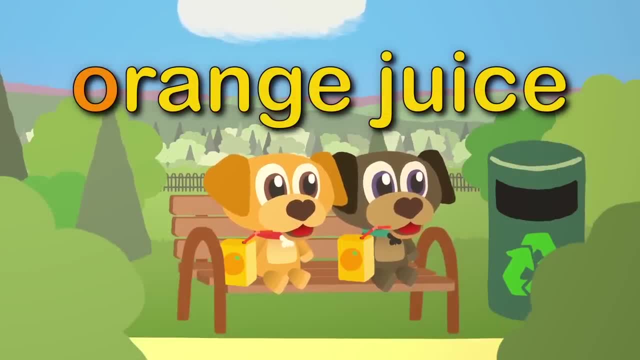 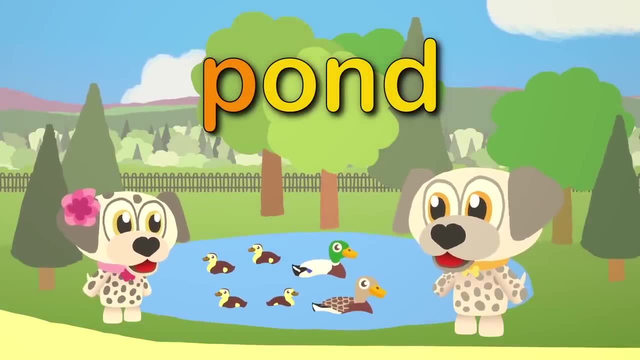 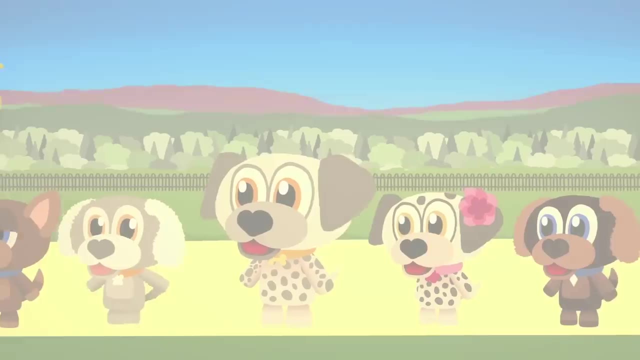 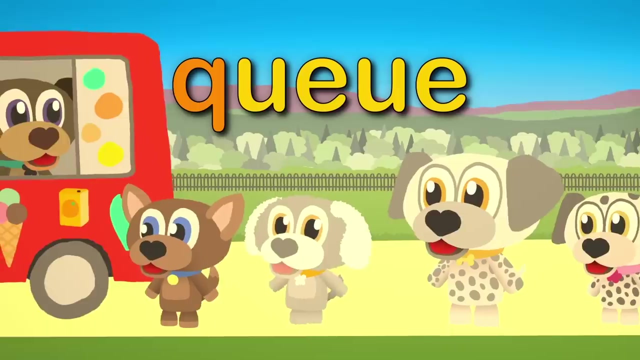 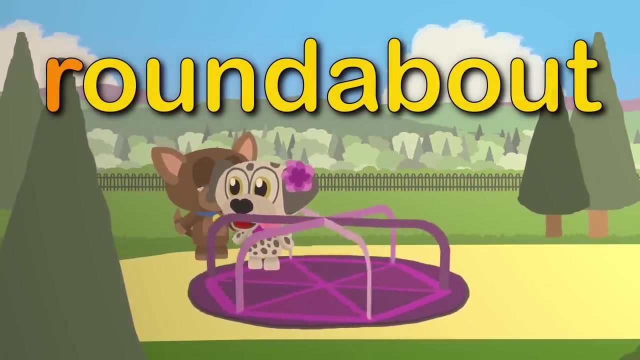 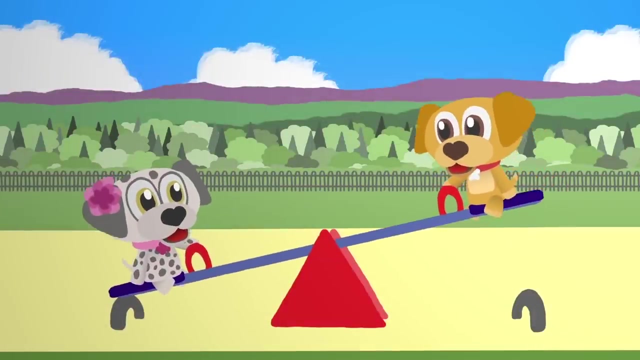 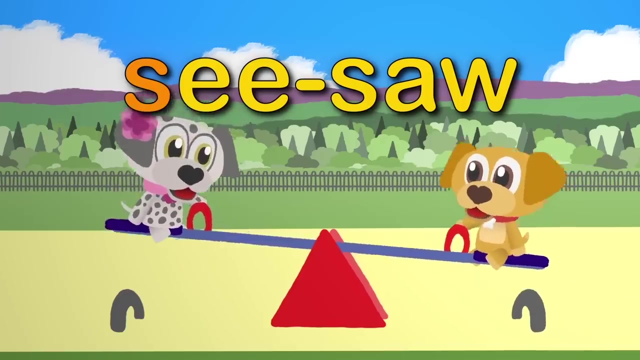 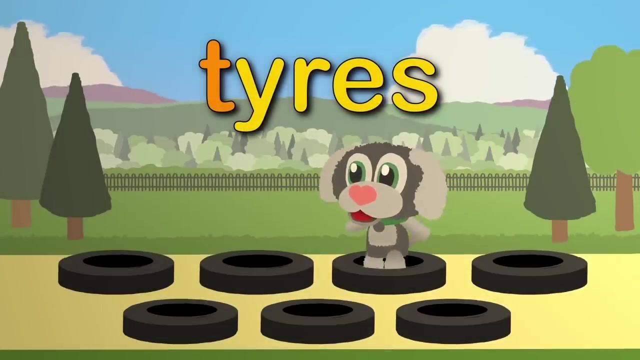 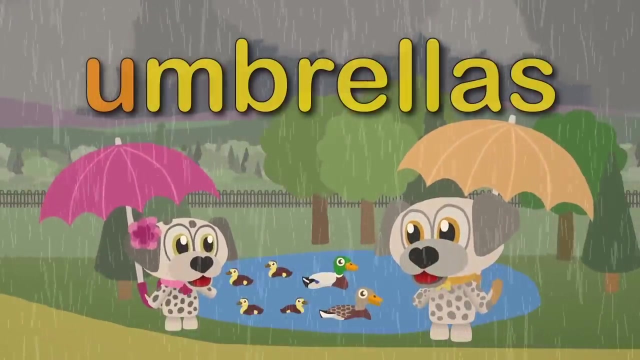 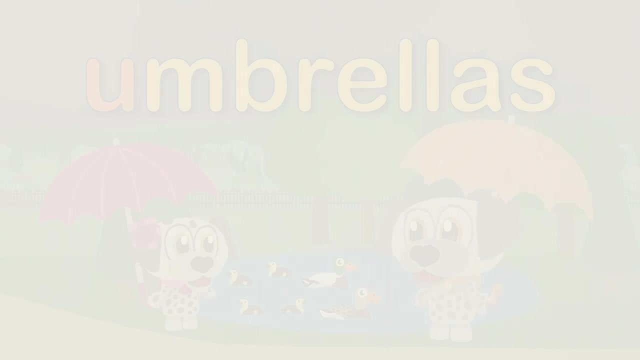 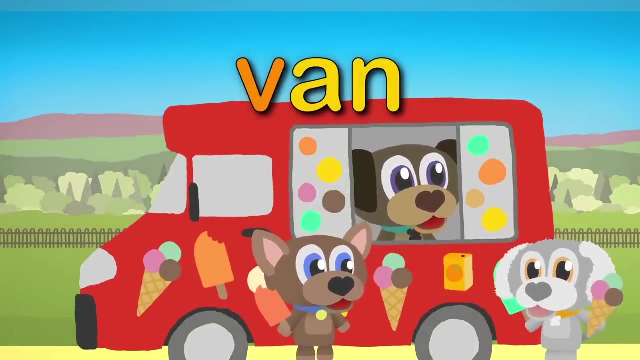 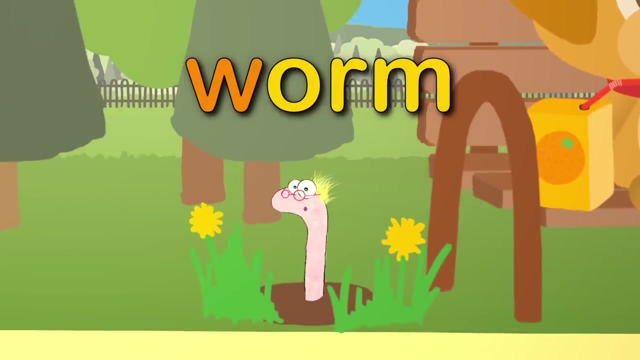 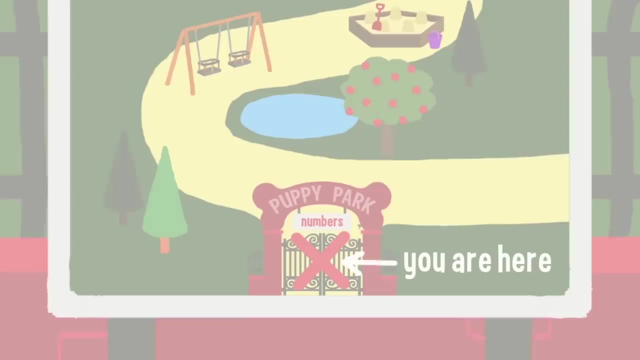 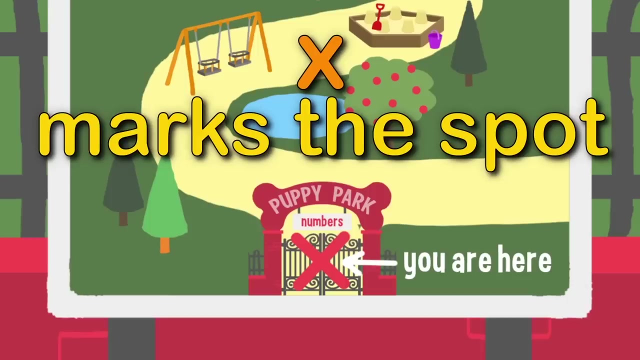 O is for Orange Juice, P for Pond, Q is for Queue, R for Roundabout, S is for Seesaw, T for Tyres, U for Umbrellas, V for Van, W for Worm, X for X. Marks the Spot That will show you where you are on the map. 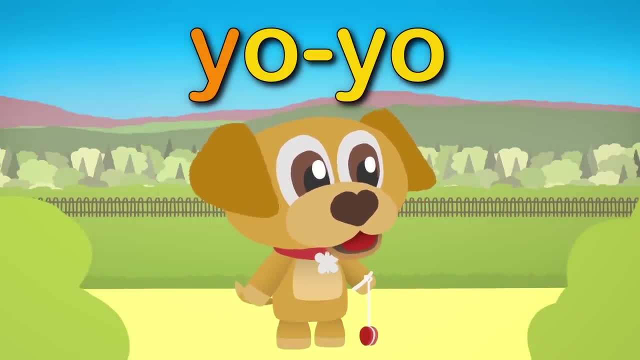 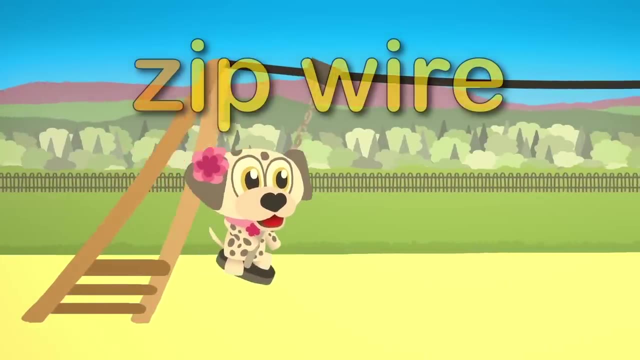 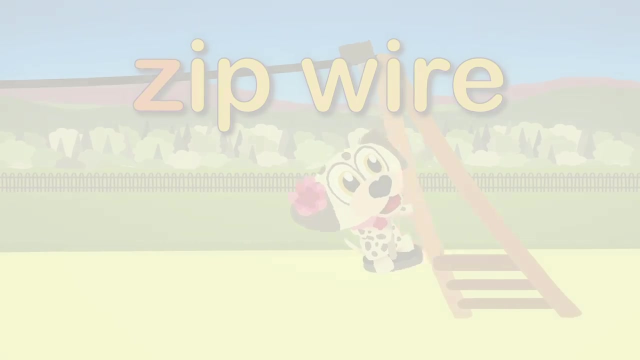 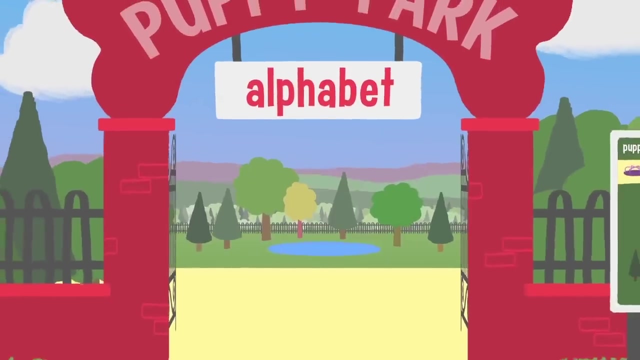 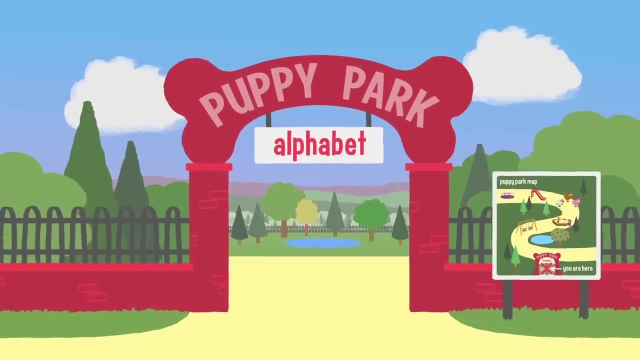 Y is for Yo-Yo, Z is for Zip Wire. We hope you've enjoyed your time at Puppy Park and learnt some new words When you're out and about. why don't you see if you can use the alphabet To help you spot new things? 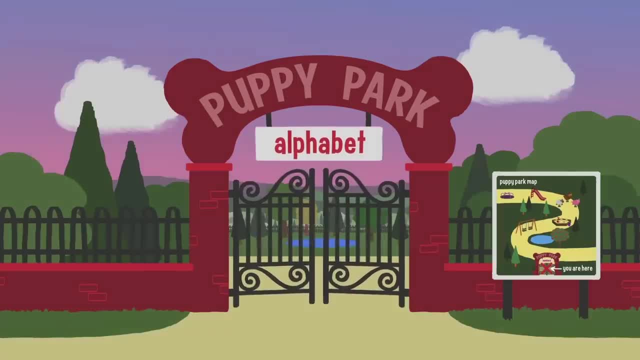 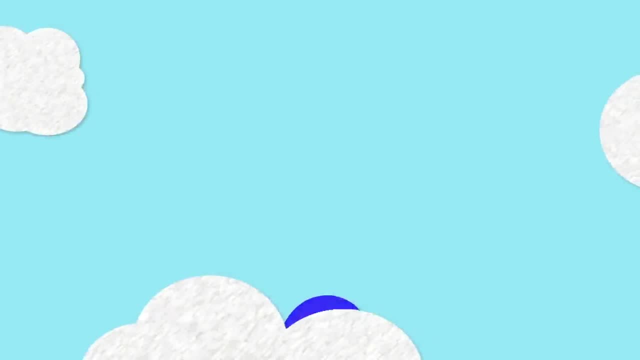 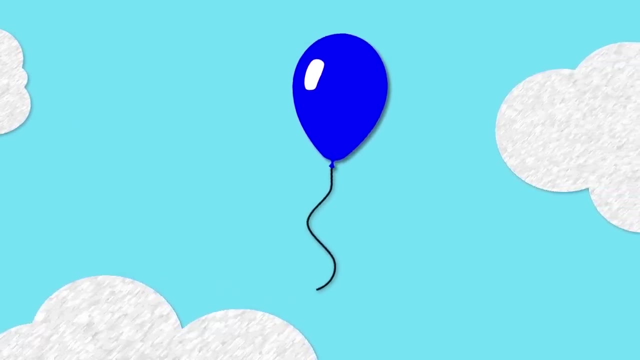 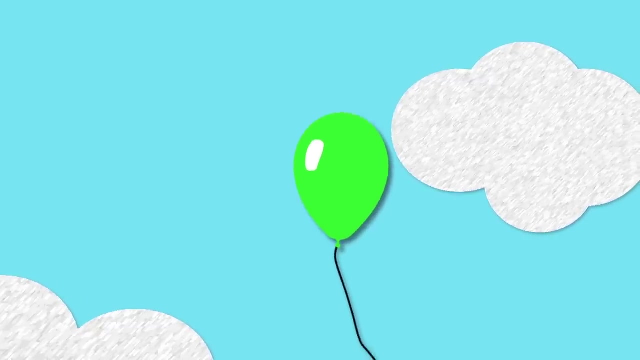 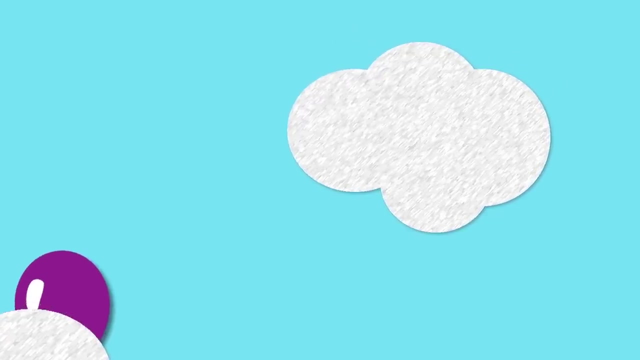 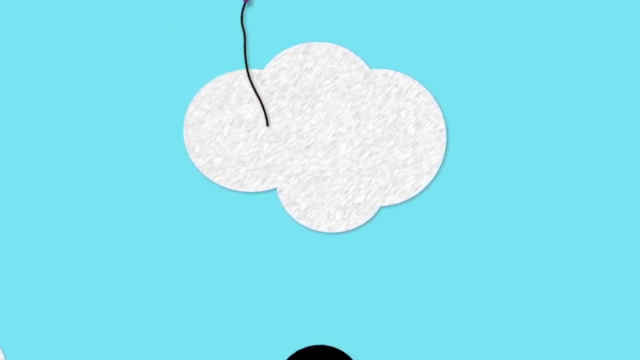 Why not try playing I Spy, Goodbye. Look, Here's a floating balloon. What colour is it? This balloon is blue. Green Balloon- Purple Balloon- Purple Balloon. Purple Balloon- Black Balloon, Black Balloon. 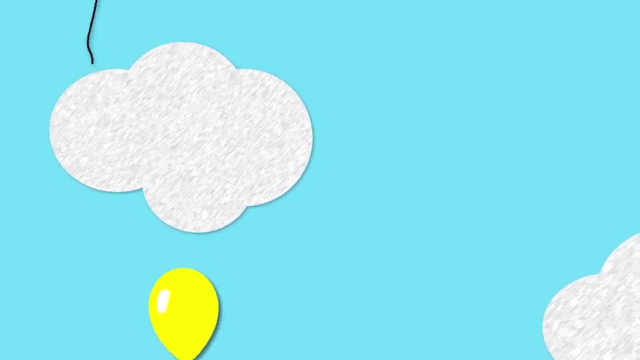 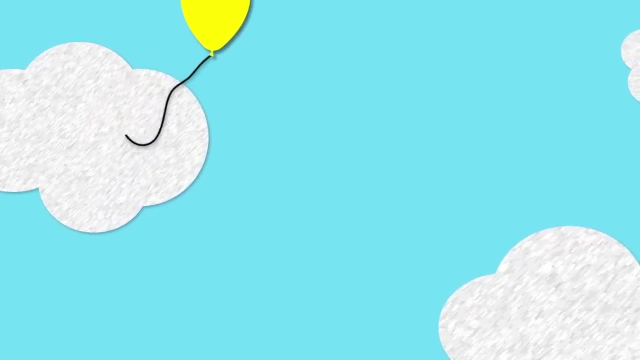 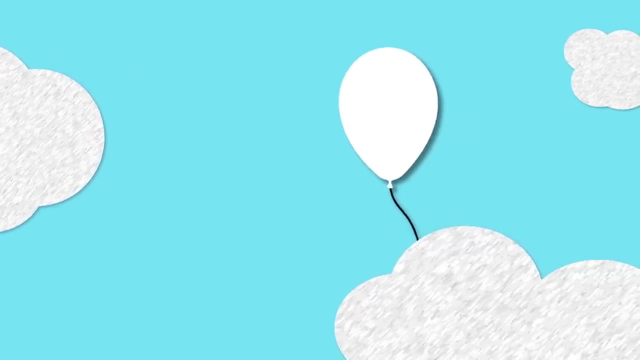 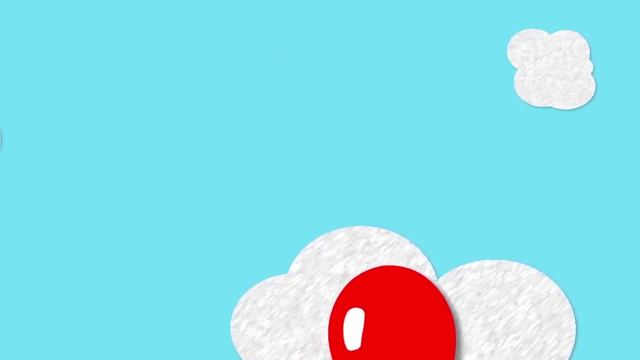 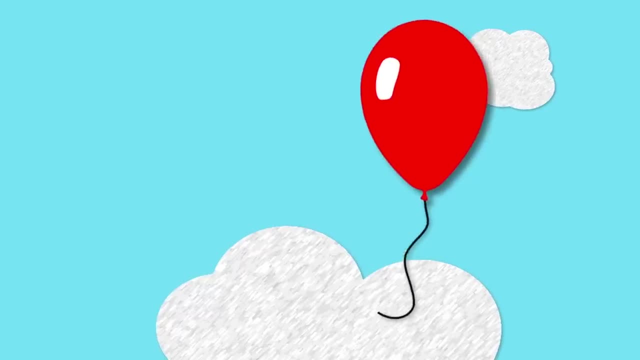 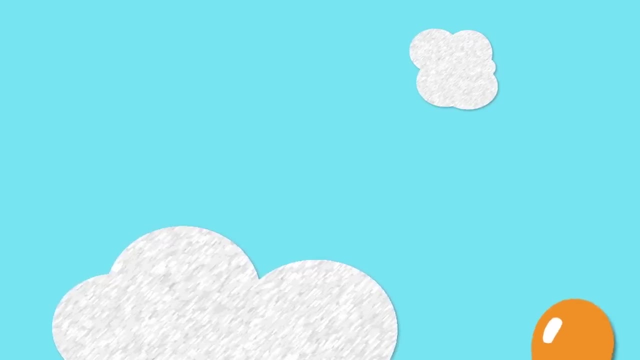 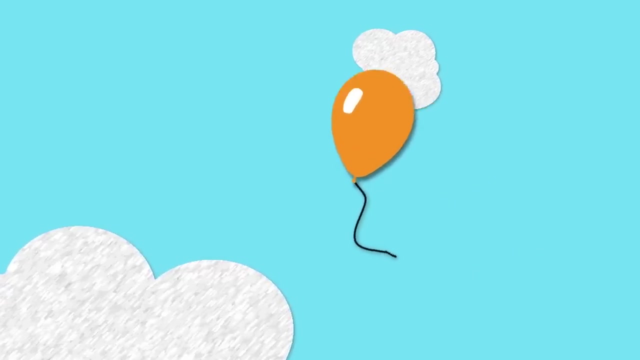 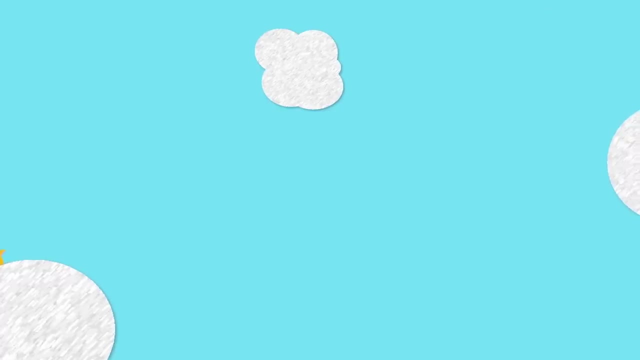 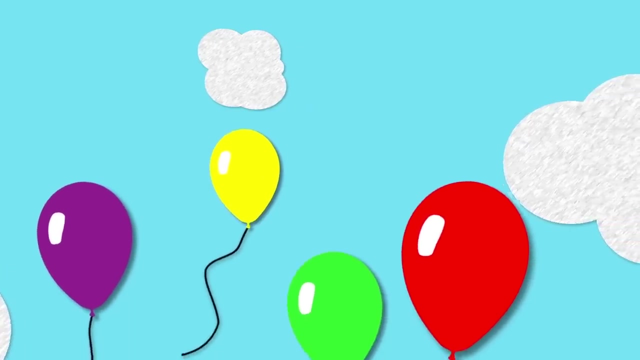 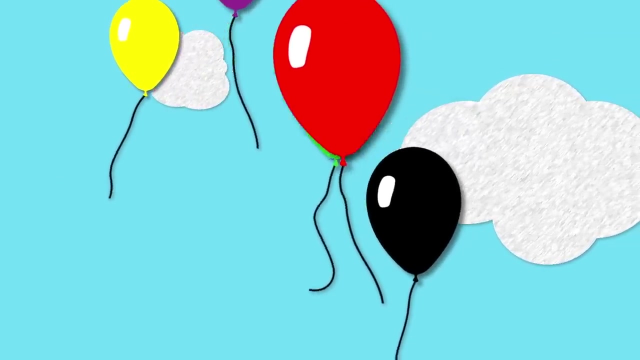 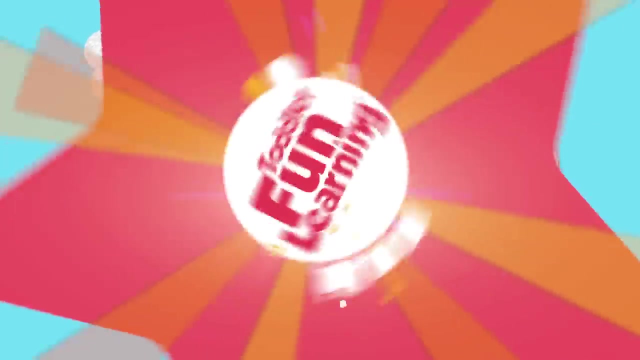 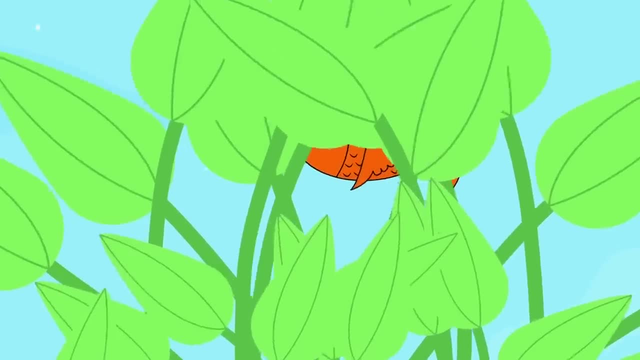 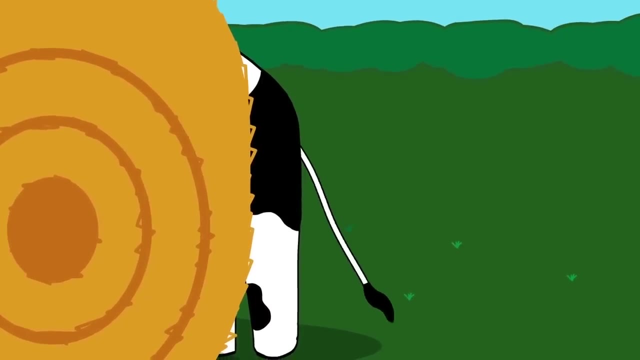 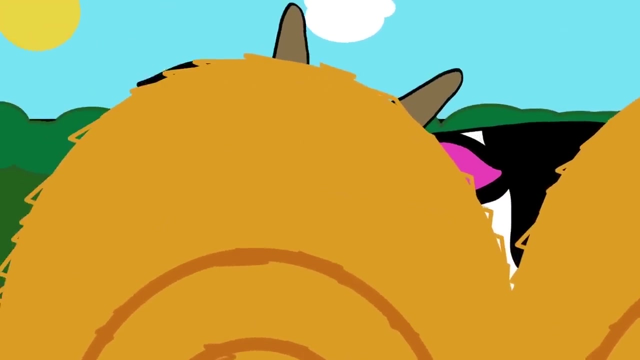 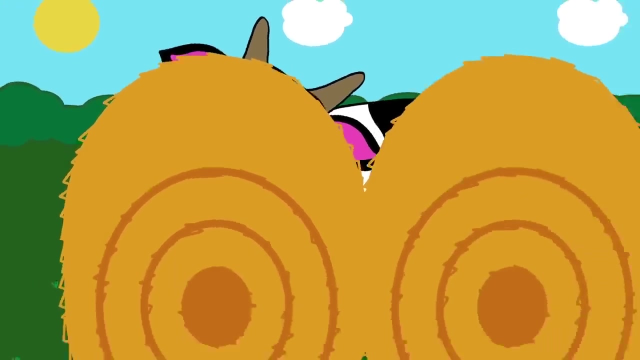 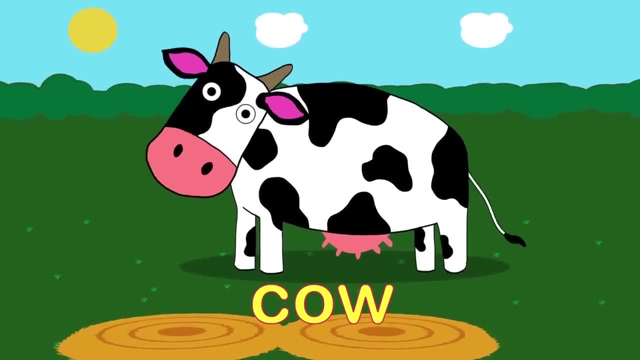 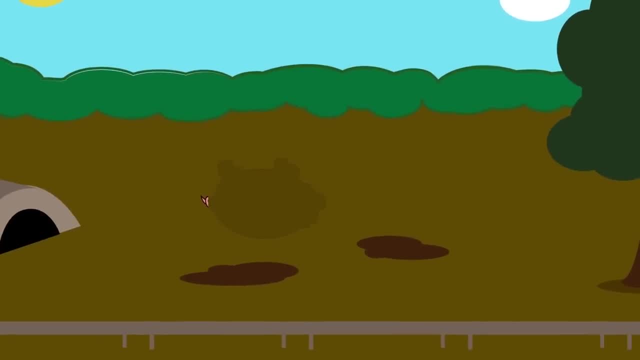 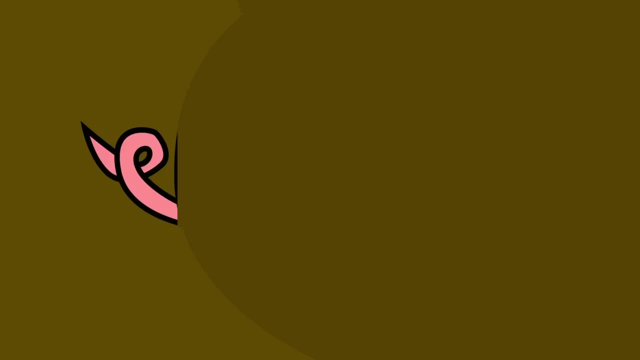 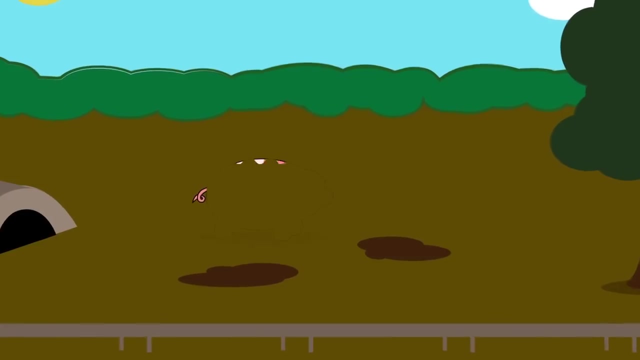 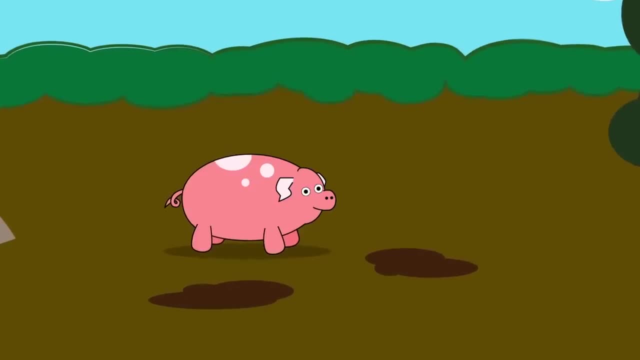 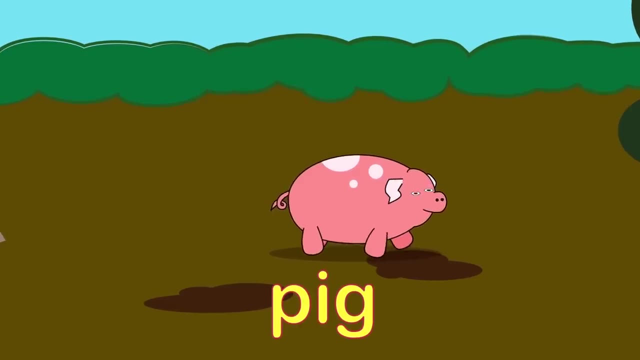 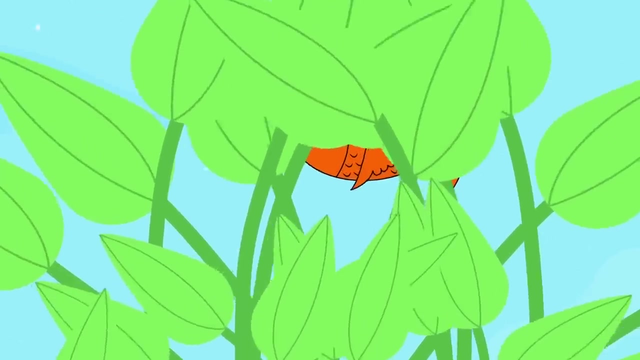 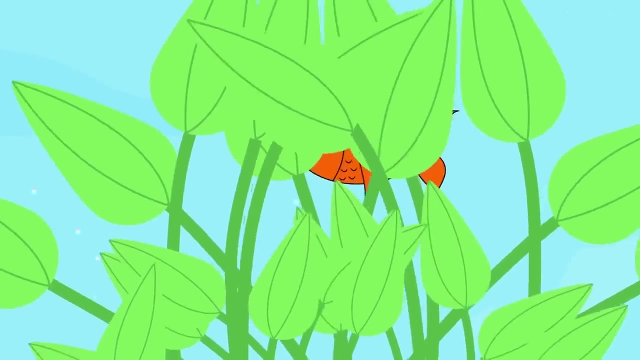 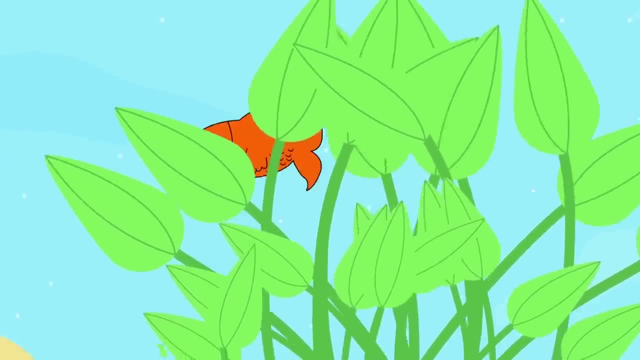 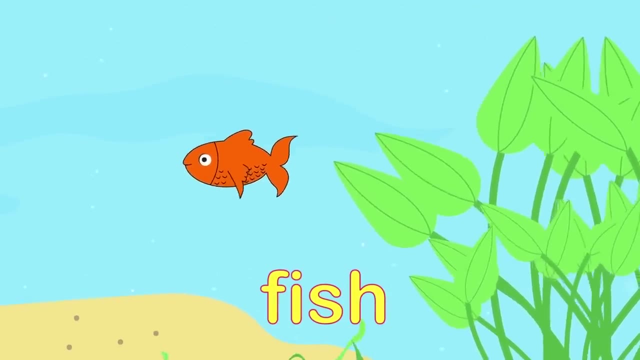 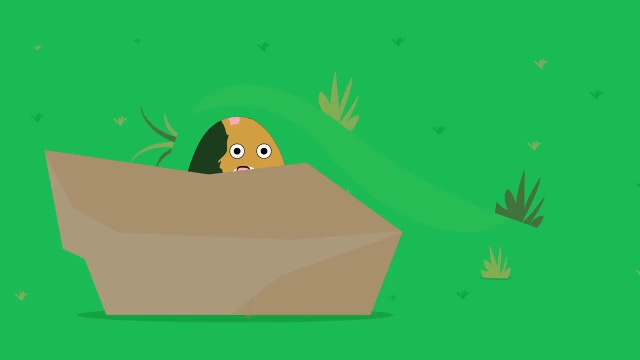 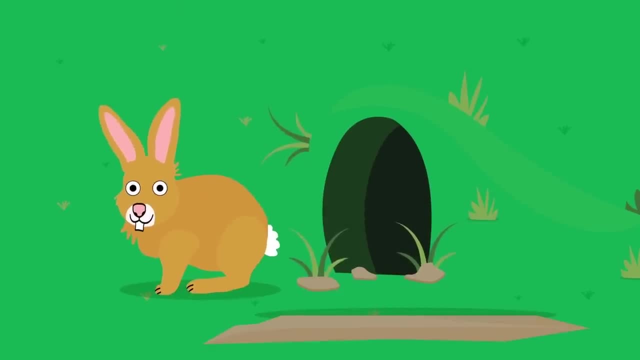 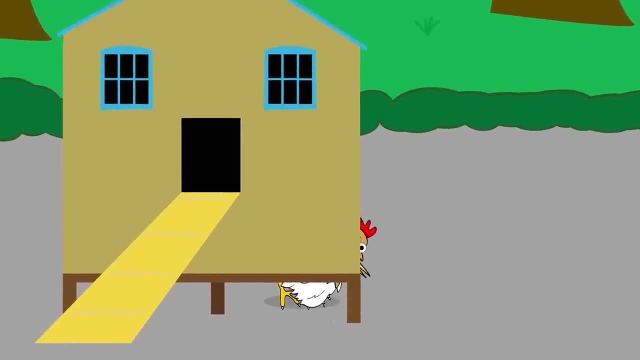 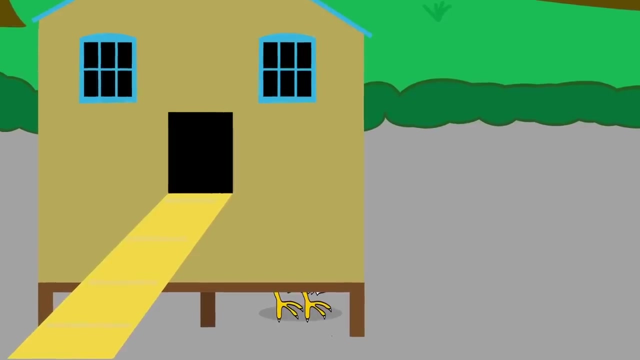 Pink Balloon, Pink Balloon. Oh, hello, rabbit, There's something pecking at that grain. Peck, peck, peck, peck, peck, peck, peck. And what noise is it making? Cluck, cluck, cluck, Cluck, cluck, cluck, cluck. 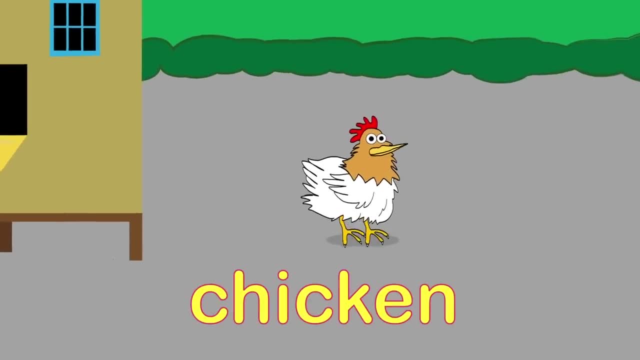 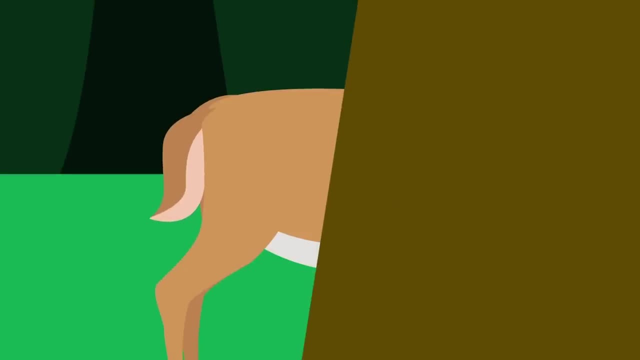 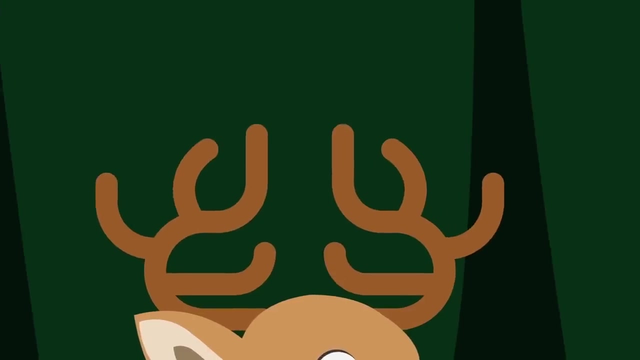 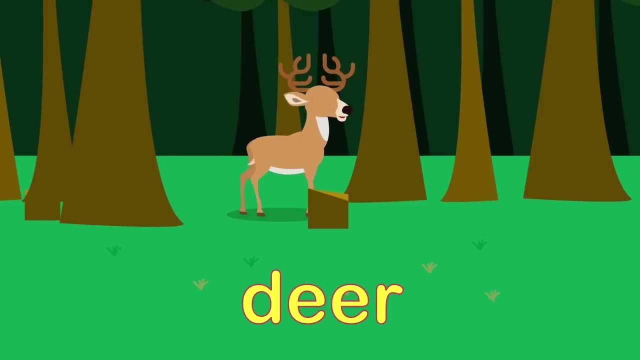 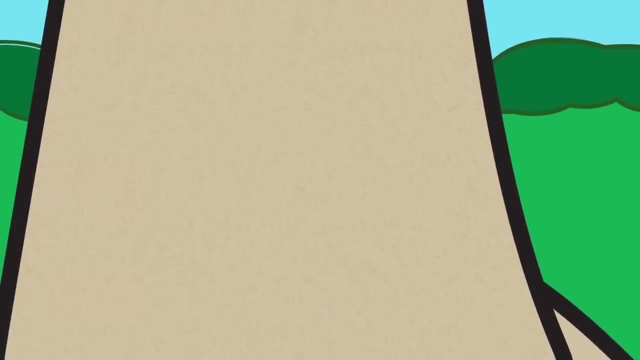 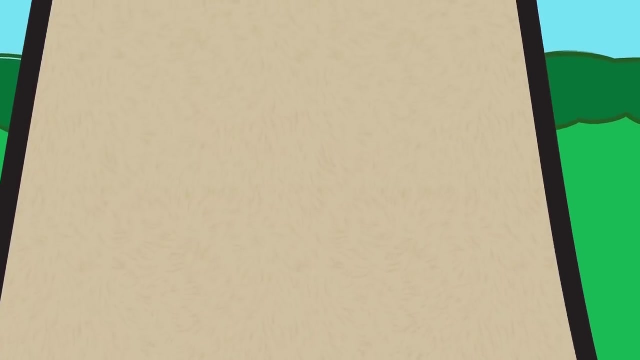 It's a chicken. This animal has beautiful brown fur and very strong antlers on its head. What sort of animal do they belong to, I wonder? It's a deer? This animal is very fluffy, with lovely, warm wool. It's not a sheep, No, no, it has a longer neck than that. 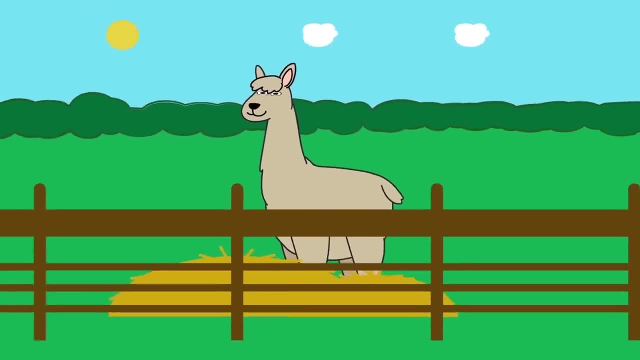 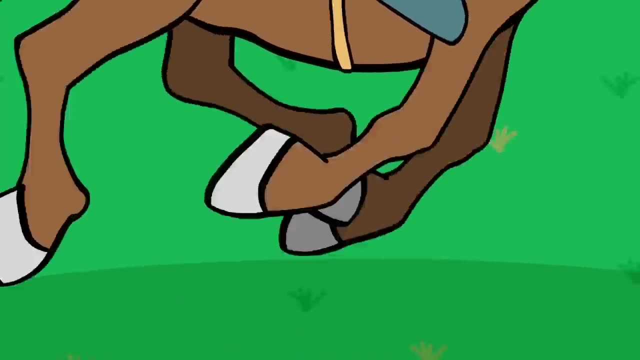 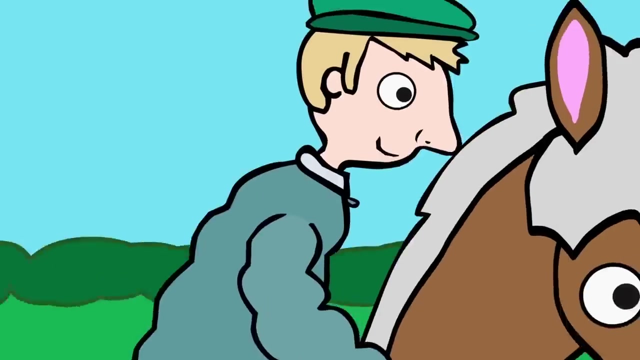 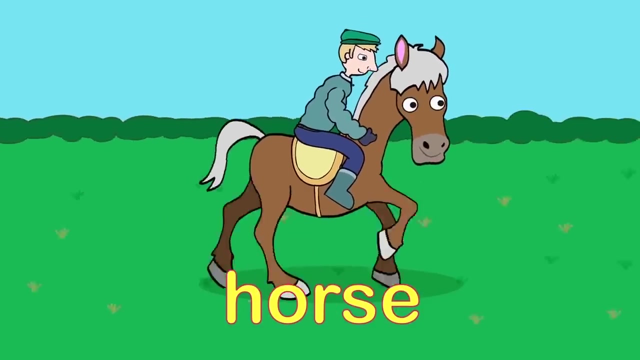 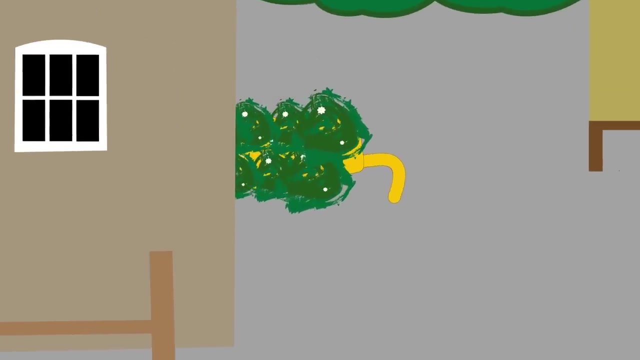 Do you know? It's an alpaca. What's this animal trotting so quickly? Wow, Farmer George is even riding on its back. Can you see its furry mane? It's a horse. Is that a snake behind the bush? No, it can't be. Snakes are scaly, not furry. 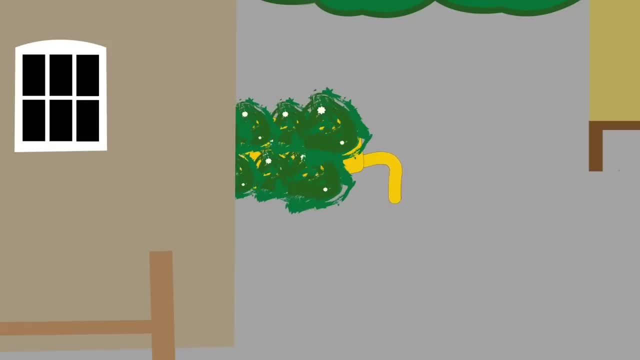 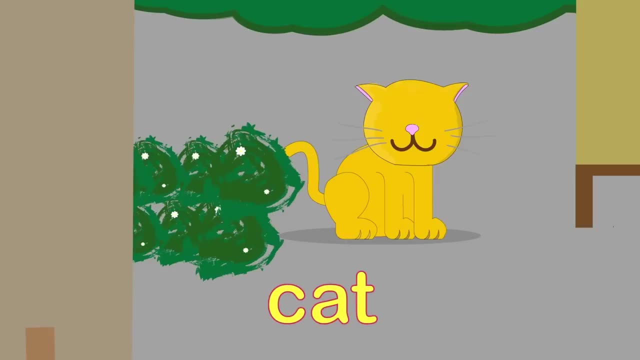 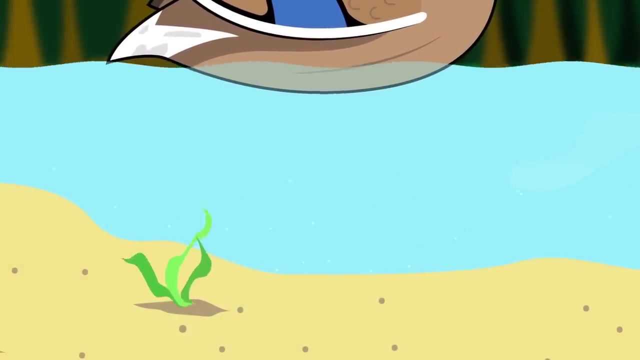 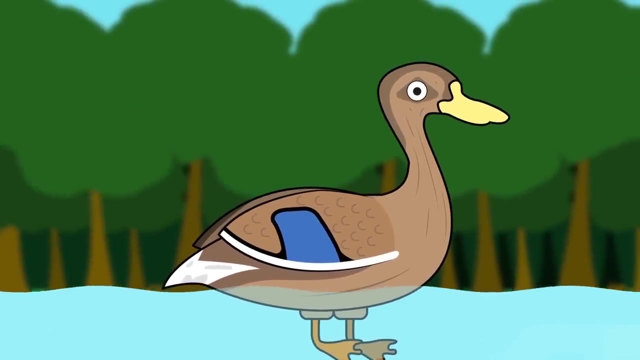 And listen. can you hear that purring sound? Oh, it's the orange cat. We're under the water again. There's something floating above us on the surface of the water. Look at its webbed feet paddling away. Let's go up and take a look. It's a duck. 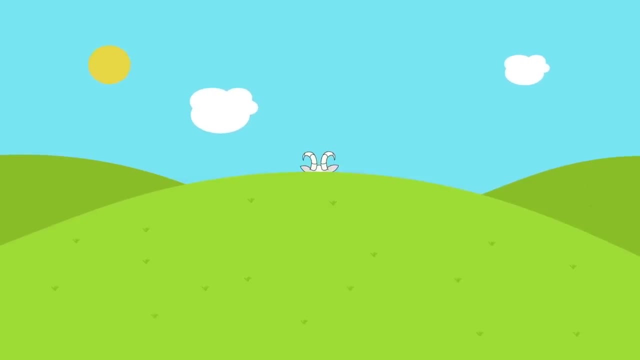 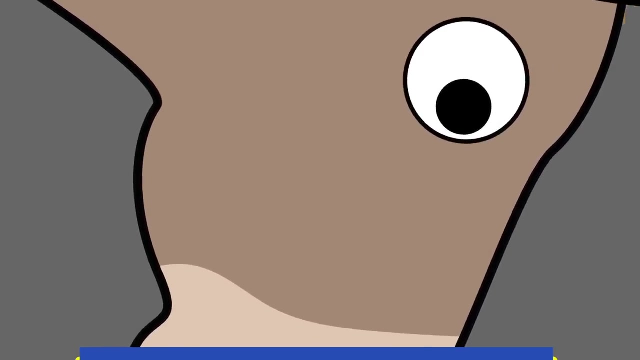 What's this coming over the hill? Pointy, curly horns And a loud bleating sound. It's a goat. Someone is very hungry today, Eating lots and lots and lots of yummy hay. There's a long, fluffy mane, But I don't think it's a horse. 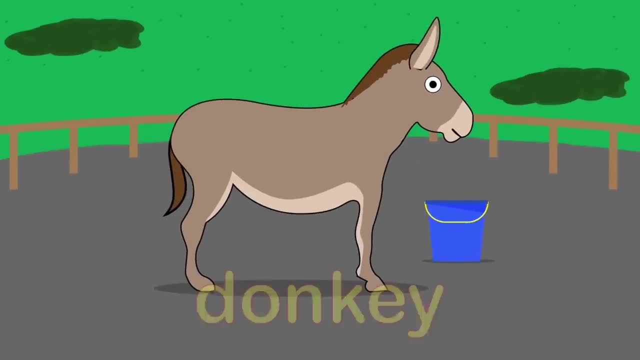 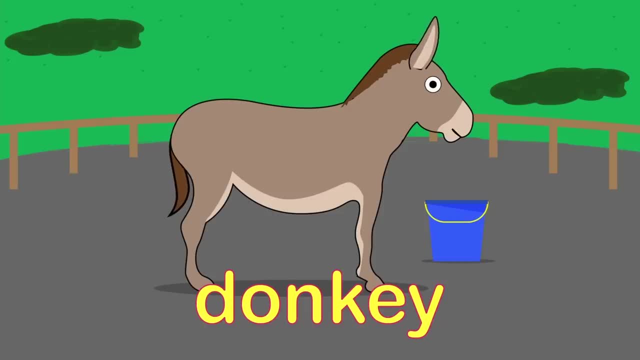 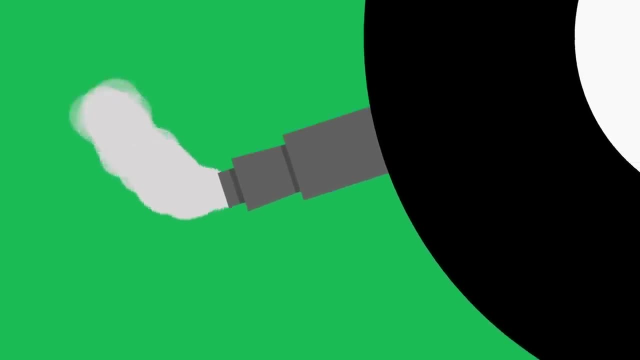 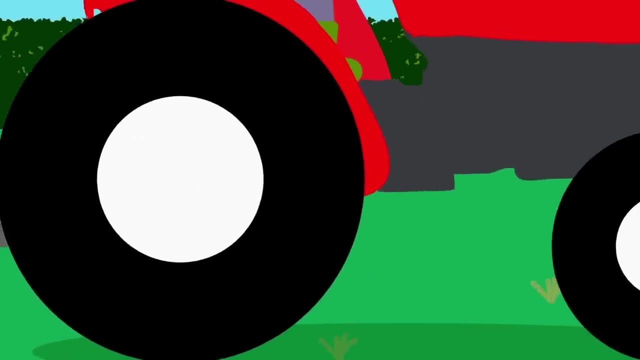 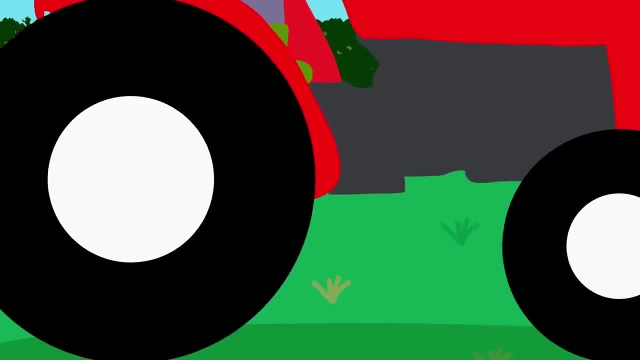 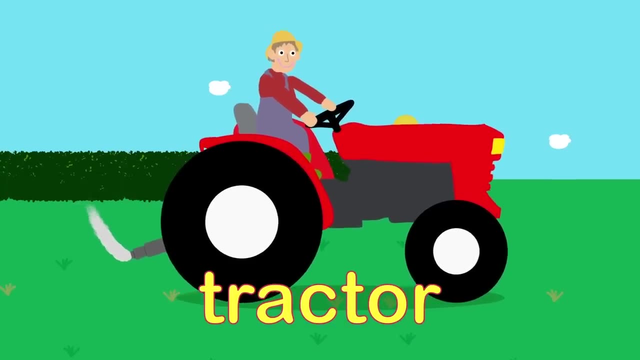 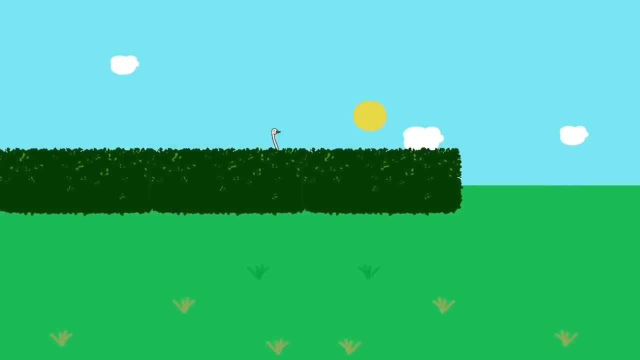 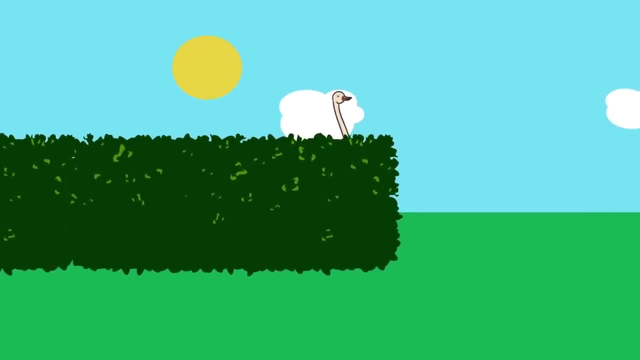 No animal I know has wheels. It's not an animal at all. It's a tractor. There's a face above that hedge running back and forth. It's got a beak, so must be some sort of bird. Wow, what a long neck. 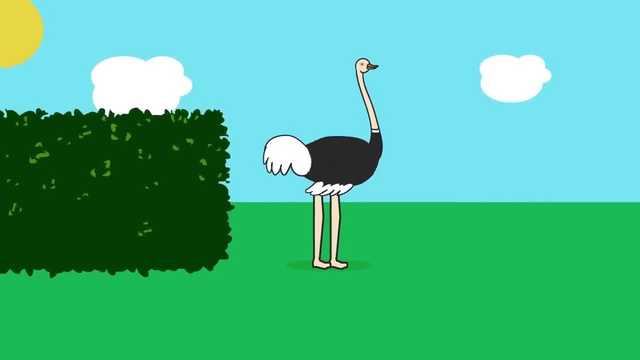 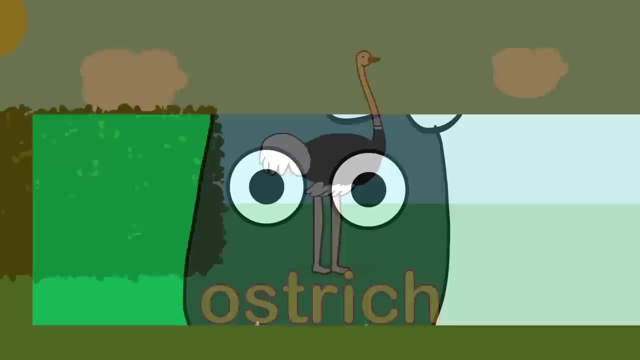 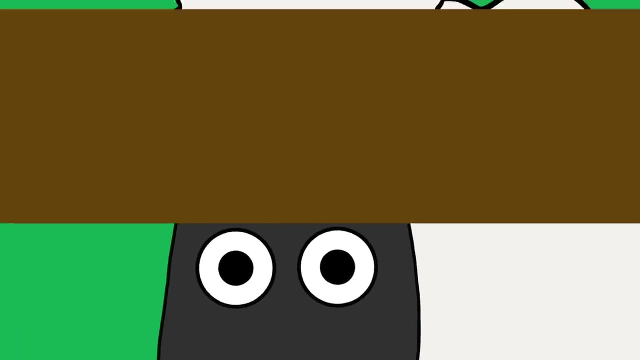 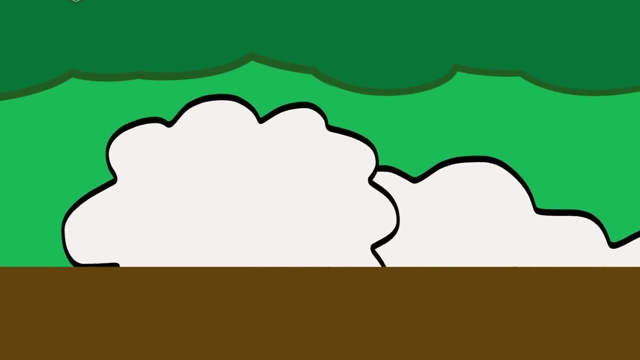 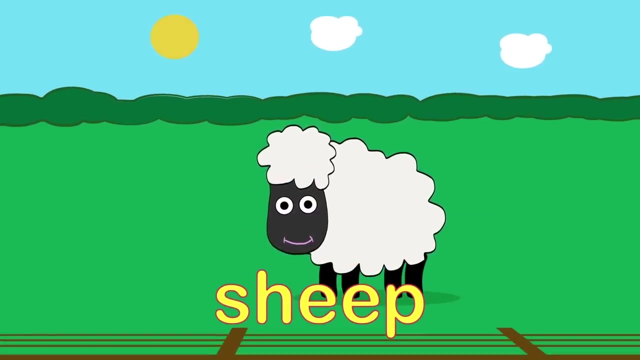 Come on out, It's an ostrich. Hello, little face, are you hiding behind that fence? What lovely, woolly fur you have. and listen, can you hear that baa baa, baa, it's a sheep. 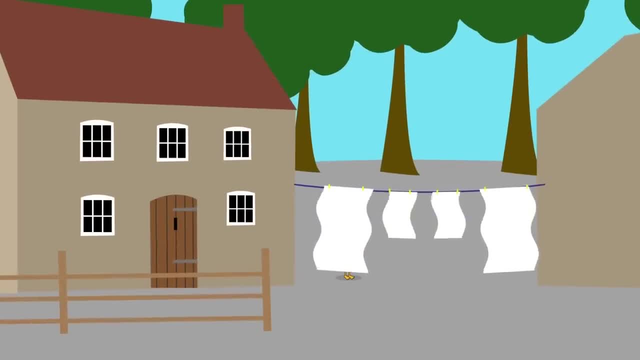 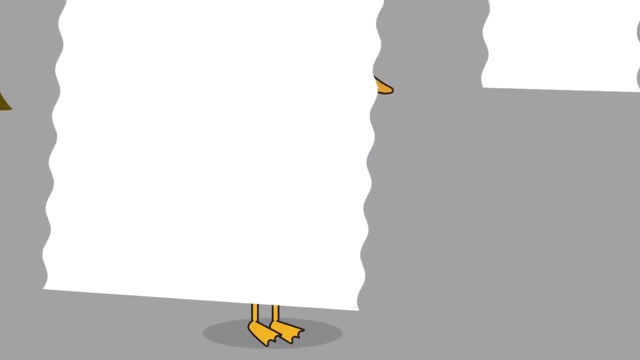 There's no animal here. Surely this is just the washing hanging up on the line. baa baa baa, listen baa baa. can you hear that? baa baa baa, and is that a beak behind the sheet? 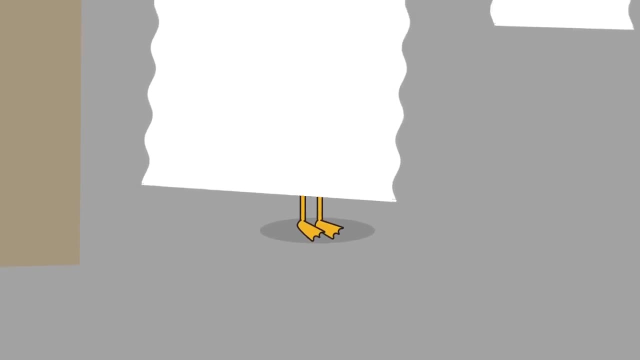 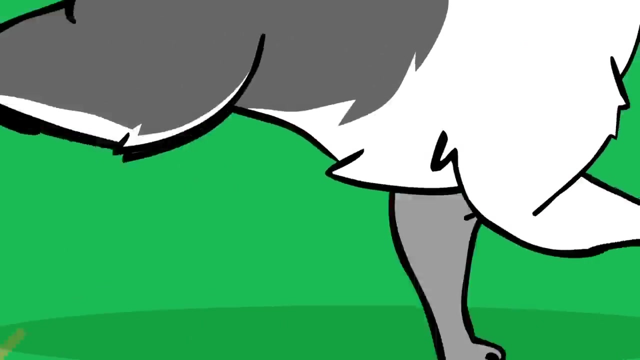 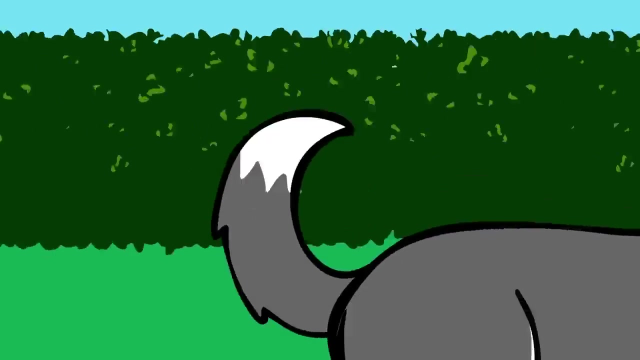 And are they feet? Yes, look orange webbed feet. baa baa baa, it's a goose. baa baa baa. the sheep are being chased. But what's that chasing them? Four legs, a long bushy tail, a loud bark, and he's very good at rounding up the sheep. 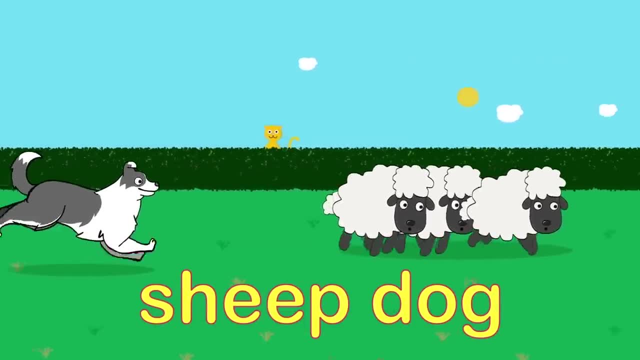 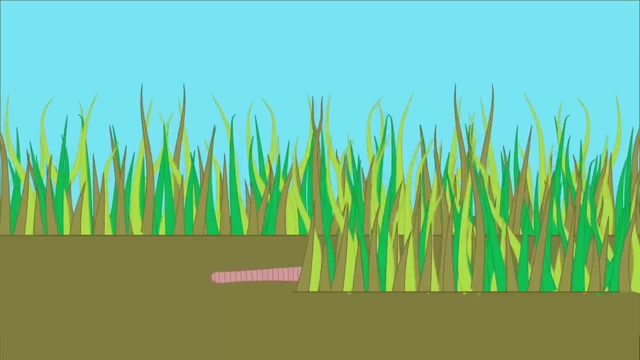 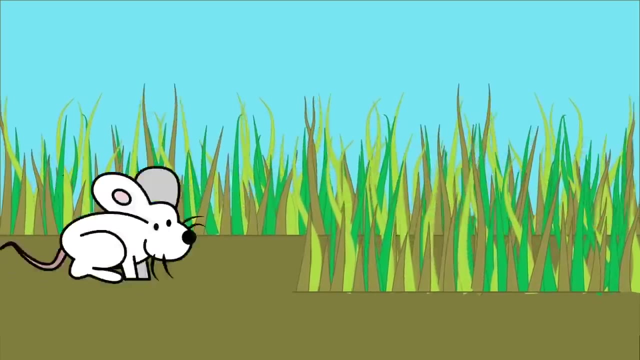 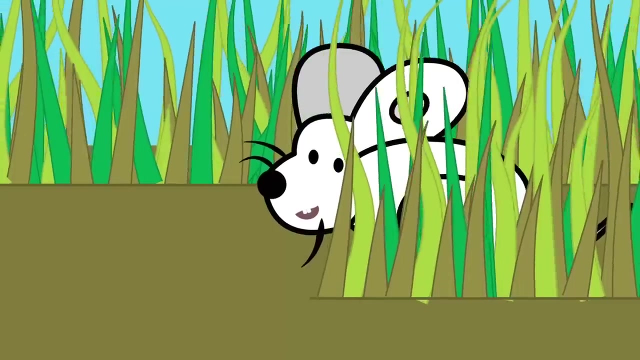 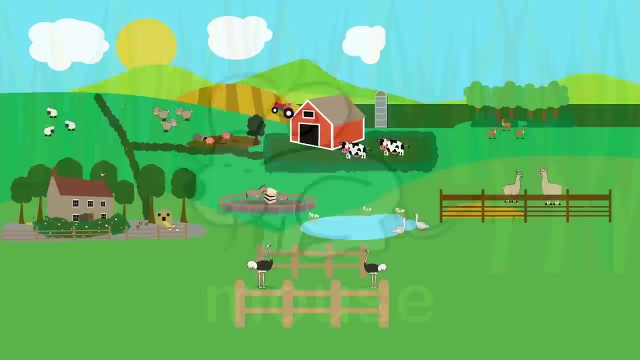 It's a sheepdog. Look, there's a worm popping out of the ground. Look out for birds, Mr Worm. Hold on, that's no worm, it's a tail. There's two pointy teeth and long tickly whiskers. it's a mouse. 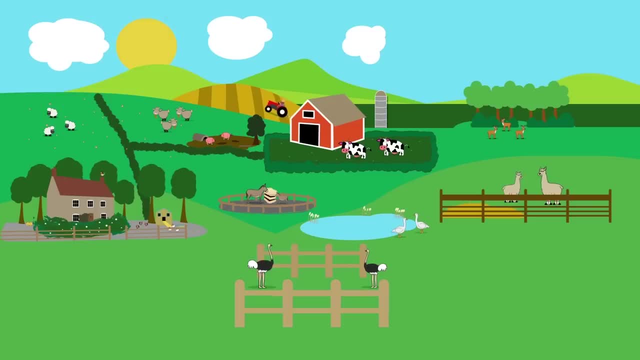 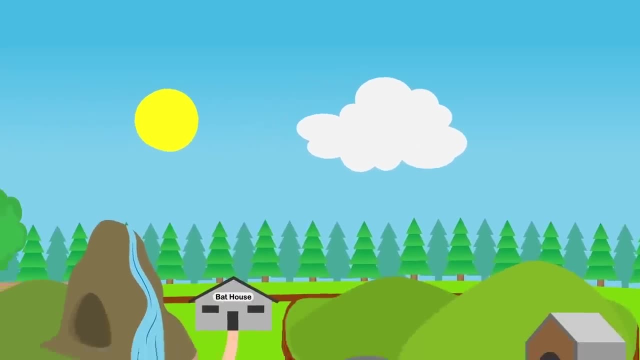 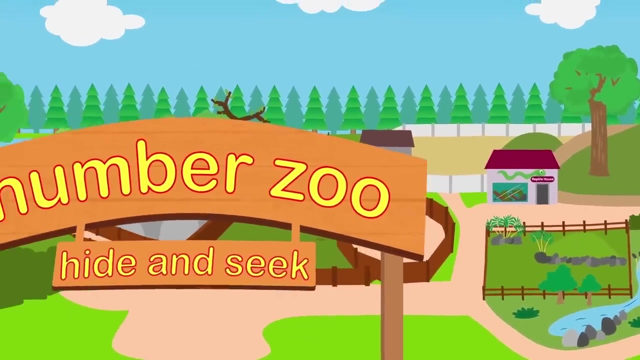 What fun we've had playing hide and seek today. we'll see you again soon down at Number Farm. Bye, We're playing a game here at Number Zoo. The animals are hiding. It's up to me and you to spot a nose, a tail, some ears, a beak in this happy game. 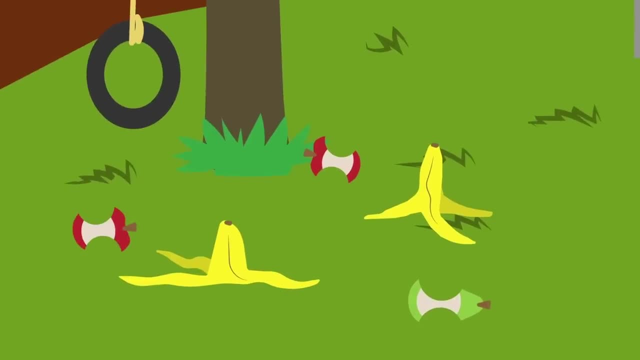 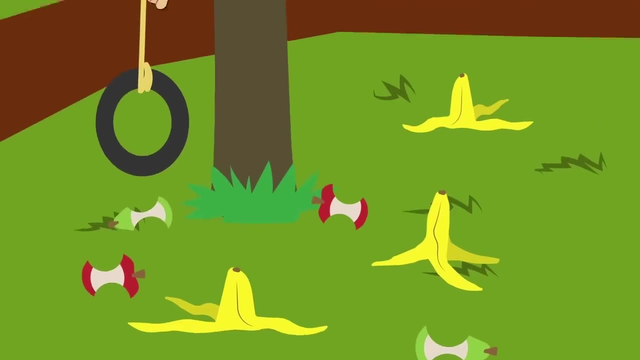 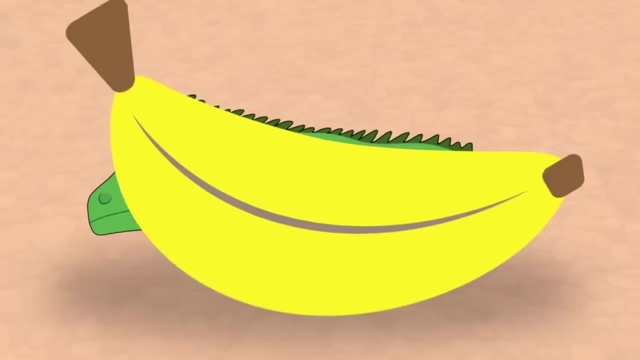 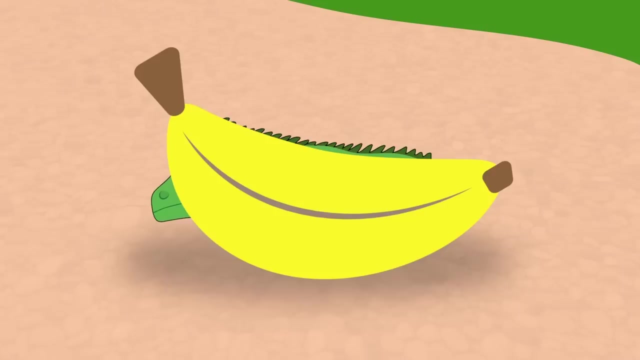 of animal hide and seek. Now what are these lying here strewn all around? And who threw that? now, Could you please turn around? It's a monkey. Oh, look, what's that now? Another monkey, Another banana, But with green scaly spikes. 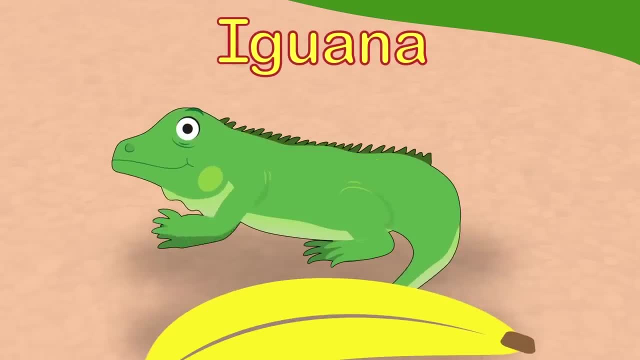 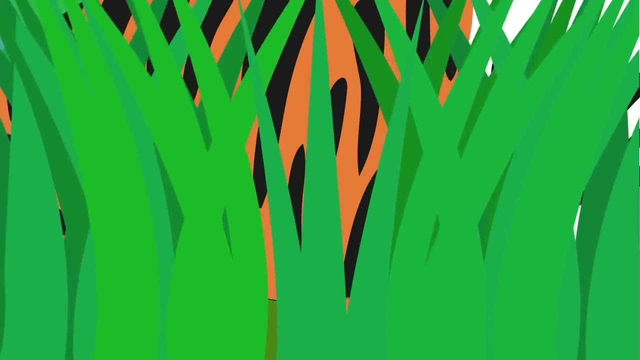 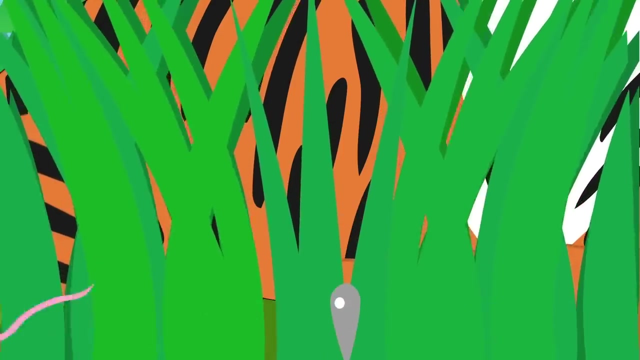 Ha ha, Of course it's an iguana Who's hiding now. And what are those Stripes? And what was that growling Mouse get out of here? Yikes, Of course a tiger. Did you get that too? 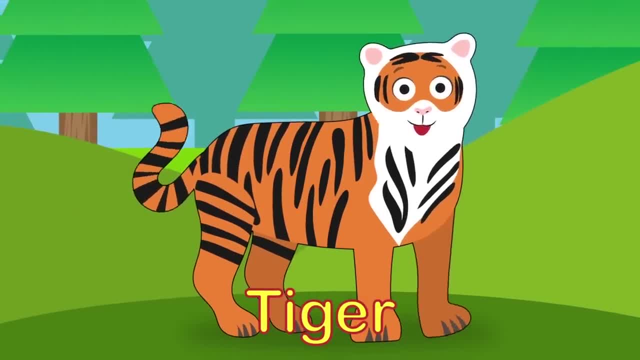 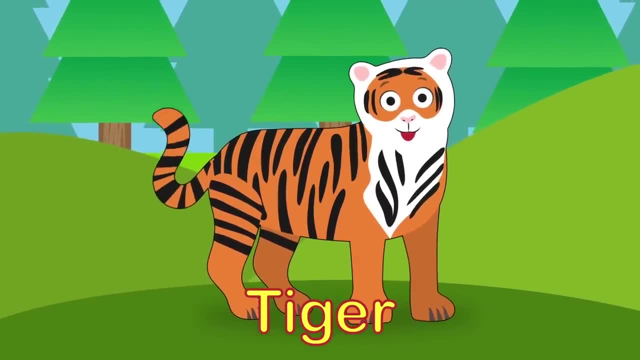 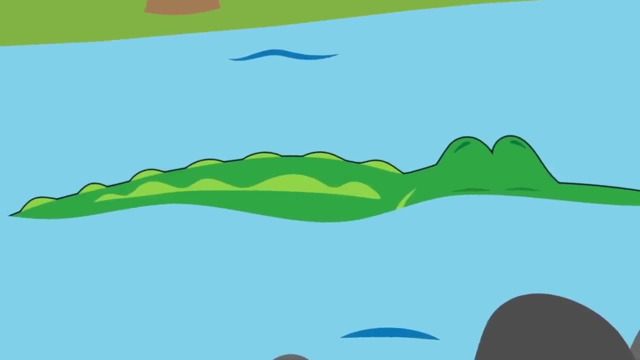 You did, Wasn't he scary? I hope we don't meet any more scary creatures now. Come on, let's go somewhere less jungly. Oh look, we can cross on this log by this stream, But wait, are they claws? 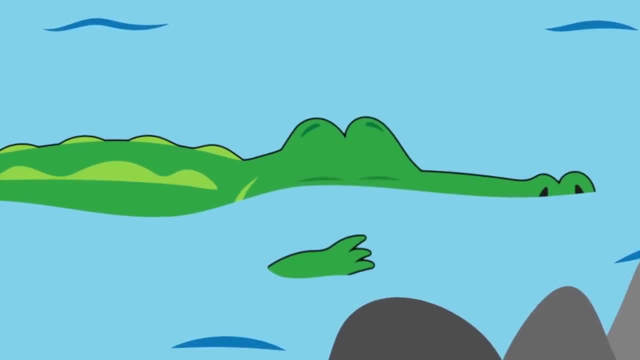 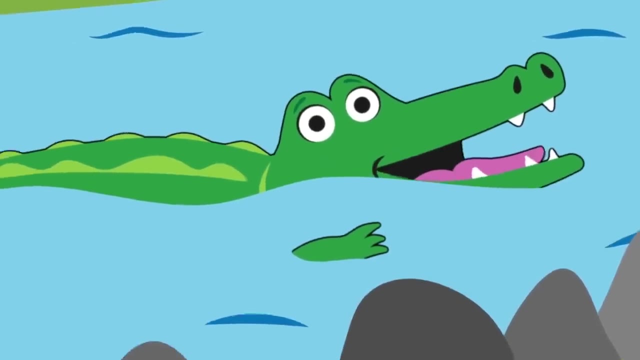 Surely logs aren't this green Unless? Yes, it is, It's an a-a-a-alligator Run. Phew, That was close. No more scares, please, Just hiding. okay, Let's sit for a while, Have a snack, then we'll go. 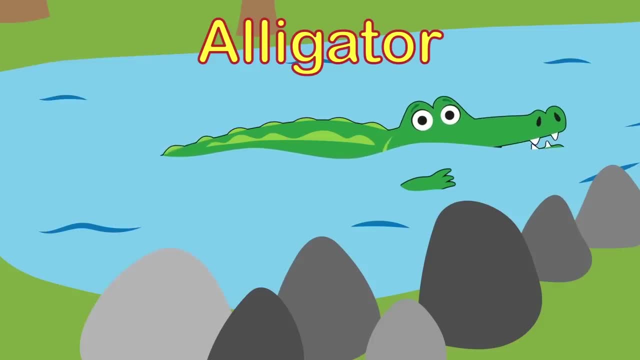 Hey, that's not a hook, it's a horn, It's a rhino. What a good hiding place, Mr Rhino. Oh look a squirrel, It's a rabbit. Oh look A squirrel. Oh, look a frog. 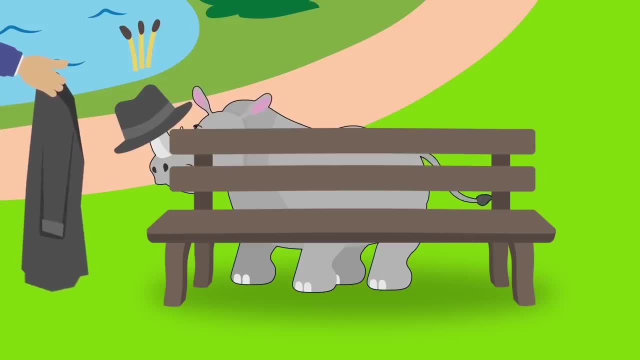 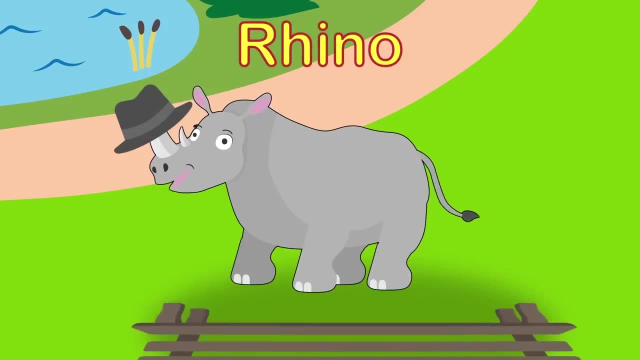 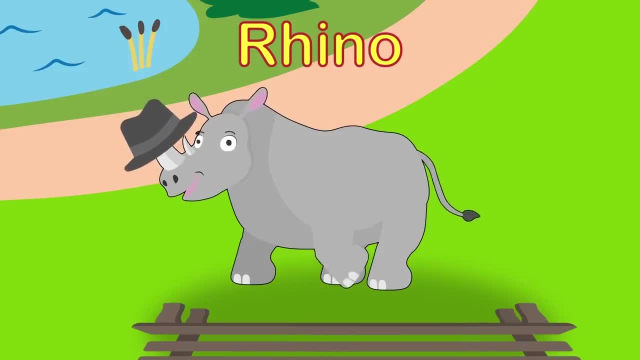 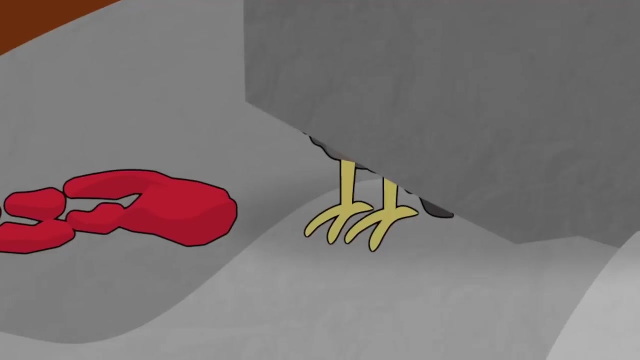 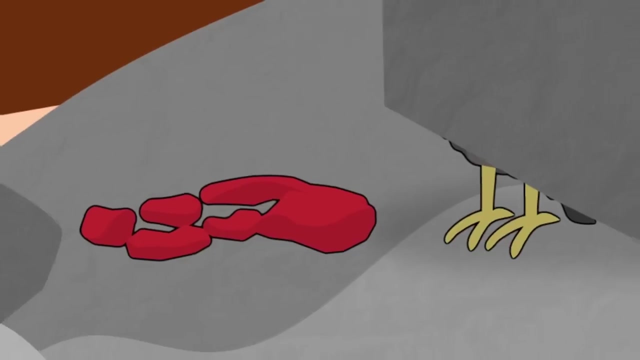 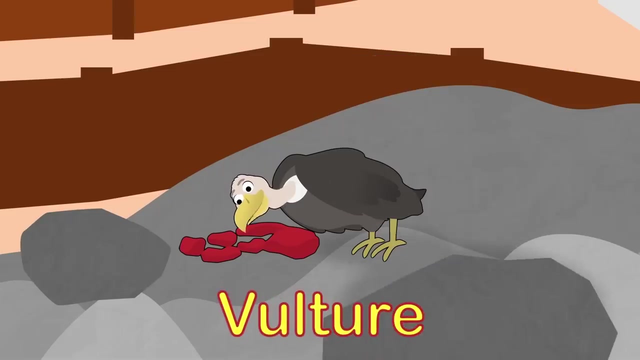 A frog, Mr Rhino. what a good place to hang a hat. funny clever Rhino who could be hiding. now what's by that big rock? look, there are some feet. and whoo, what's that smell? it's raw rotten meat. you animal would eat that- a vulture, of course. who will we? 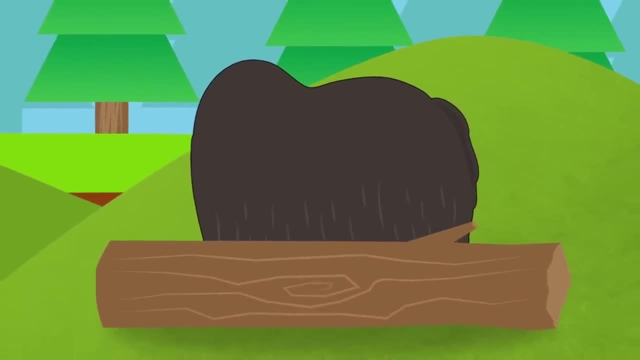 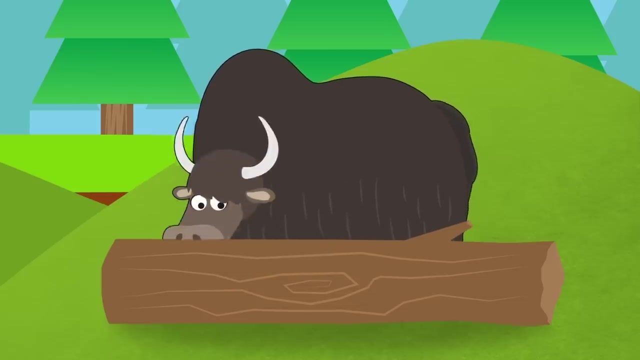 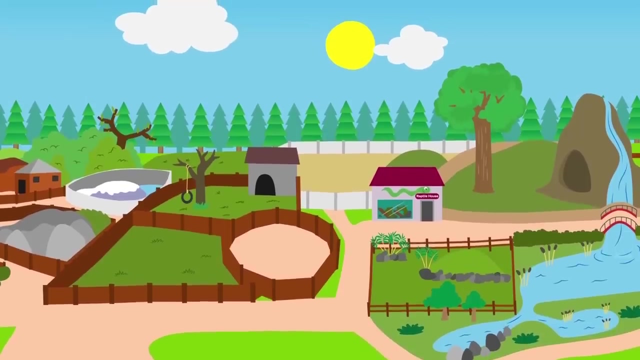 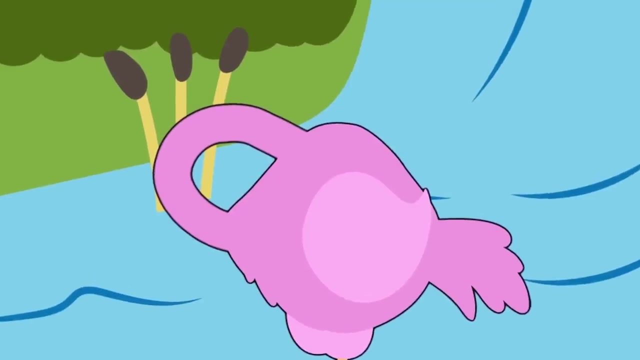 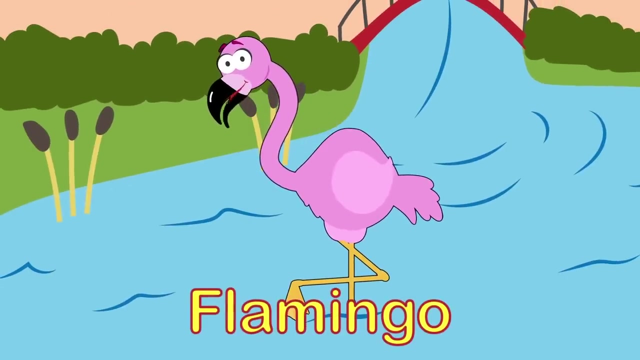 find next? I wonder. this sofa looks comfy. love the warm, fluffy back. wait a second, it's moved. haha, that's because it's a yak. who else might be hiding? do you think? how strange, how absurd. one leg and no head hang on. it's a rather sleepy flamingo bird. that's a funny way to. 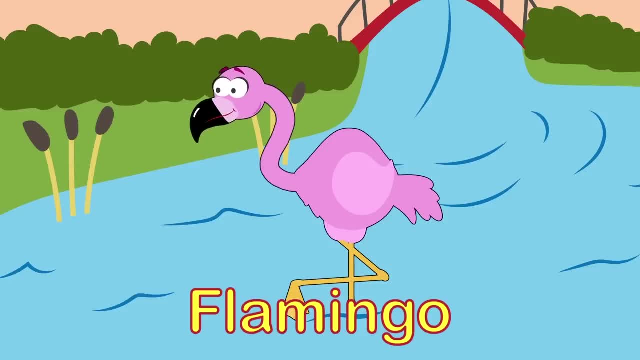 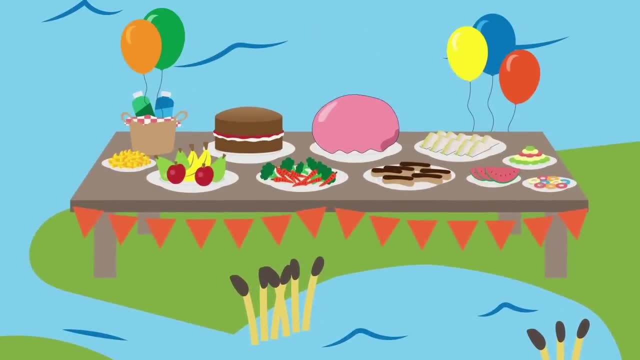 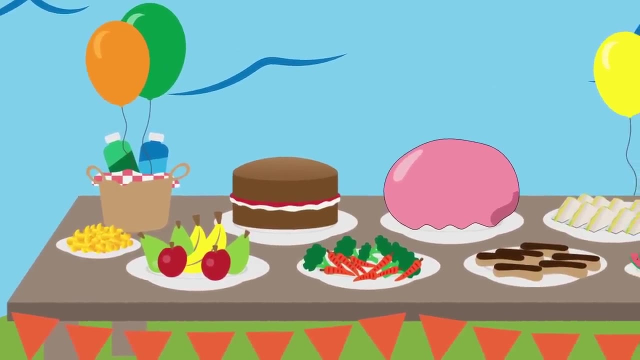 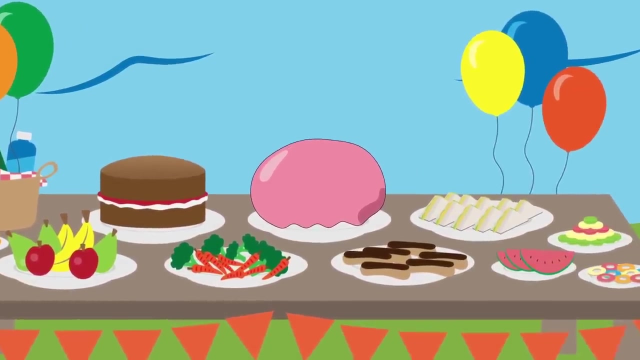 sleep now. who'll be next? who's hiding, do you think? look a party with lots and lots of delicious looking food. yum, mmm, cake on a plate, jelly on a dish, but wobbling that much. hey wait, that's not food, it's a wibbly wobbling. 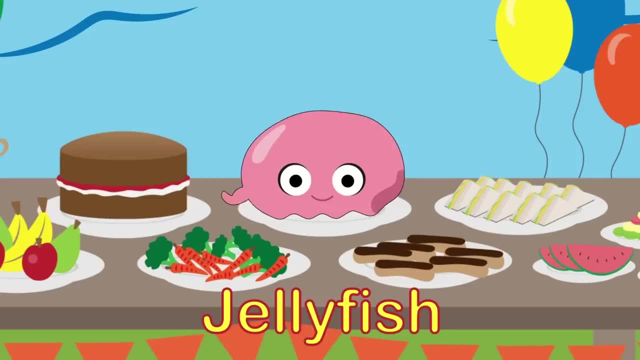 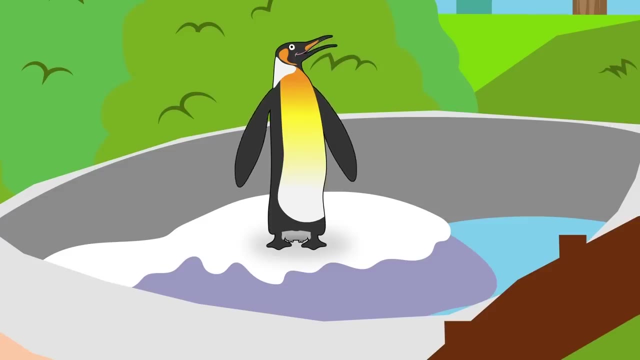 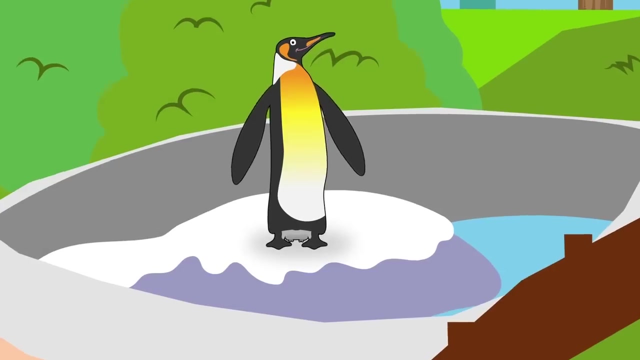 jellyfish. haha, cheeky jellyfish. were you pretending to be party food? a? that could have been nasty, you crazy wobbling jellyfish. I wonder who's hiding now? a penguin, but you're not hiding, are you, Mrs Penguin? hey, wait, what are those underneath by your? 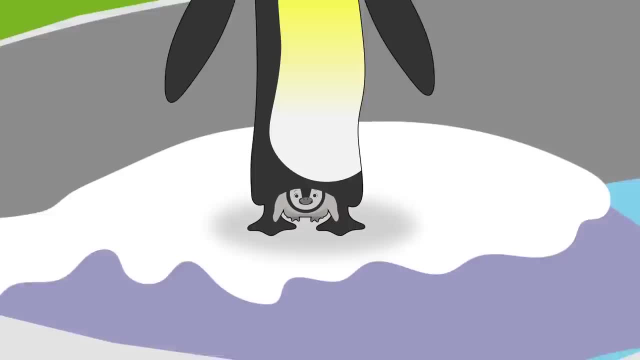 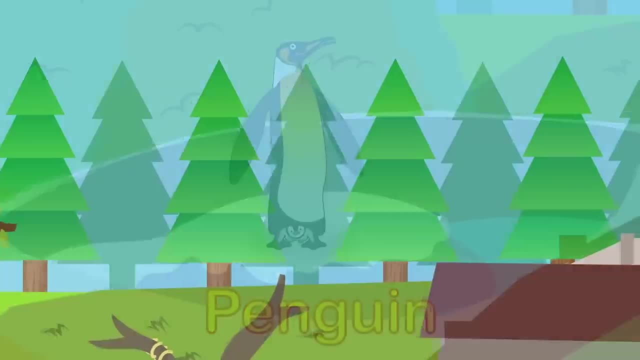 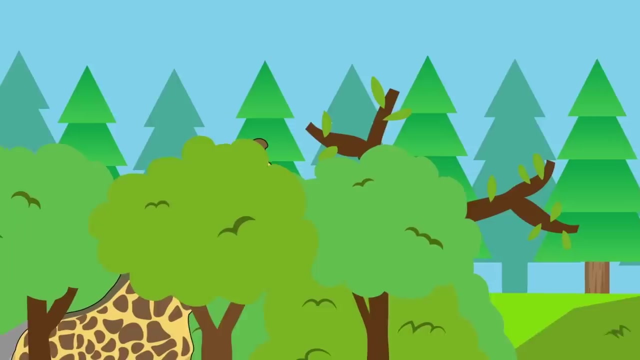 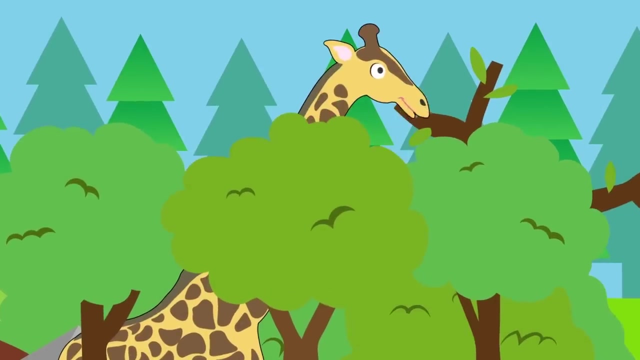 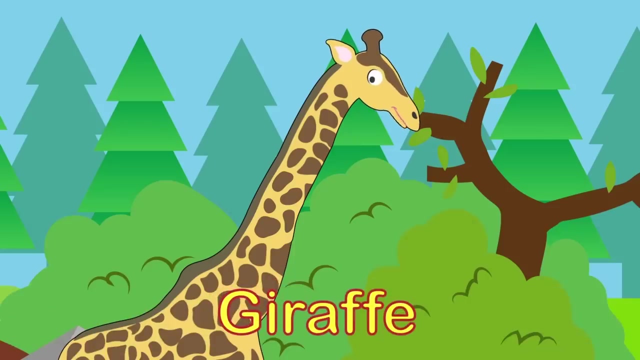 tummy four feet. no, that's a baby and you are its mummy. what a cute baby penguin that was. I wonder who else might be hiding in the zoo. hey, stop, what was that moving their in the leaves? look, it's a munching giraffe that's as tall as the trees time. 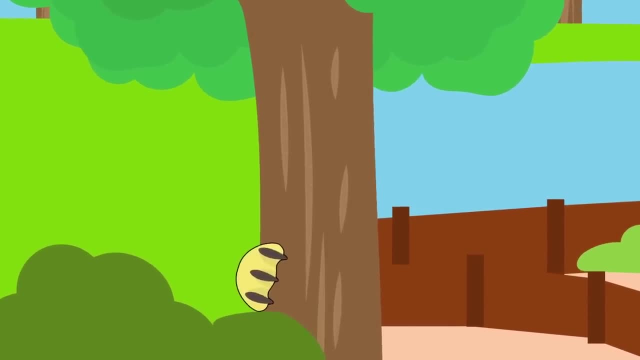 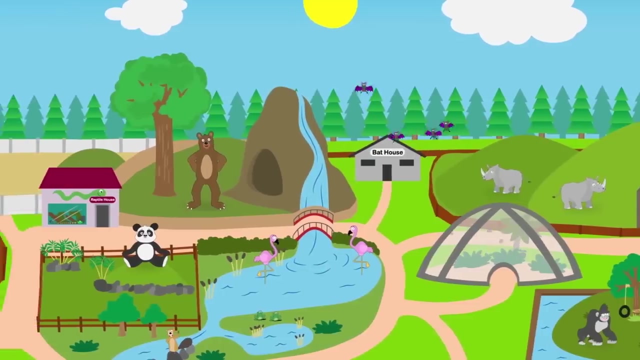 to go home. now let's finish our game. what's there by the tree? A claw, Now a mane. Of course it's a lion. Well done, Mr Lion. I must say you've all hidden really well. I've had a lot of fun, Have you. 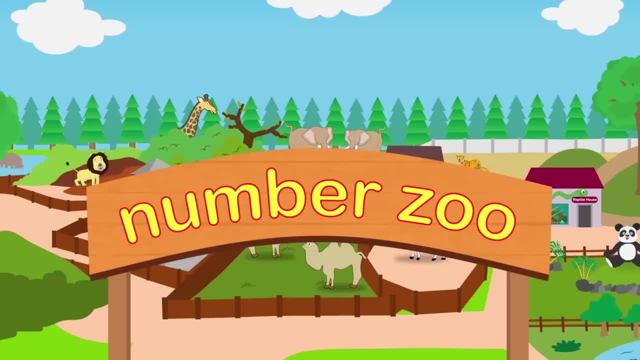 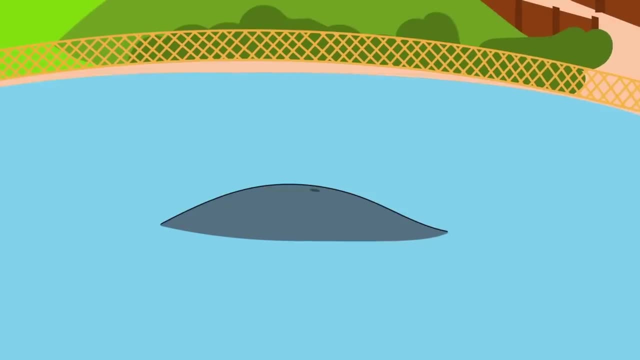 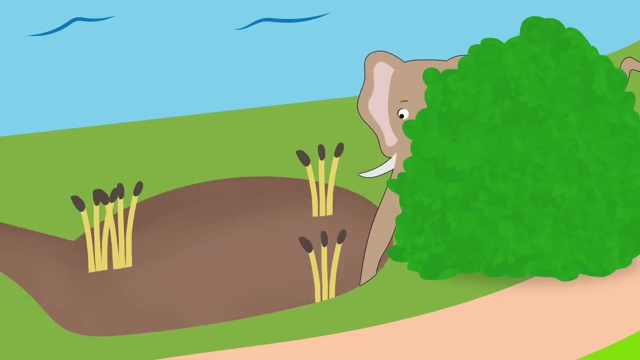 So see you next time down at Number Zoo. There's more animals hiding down at Number Zoo today. Shall we see who wants to come out and play? Now, where did that pond go, And who used that hose? Aha, now I've guessed it: An elephant's nose. 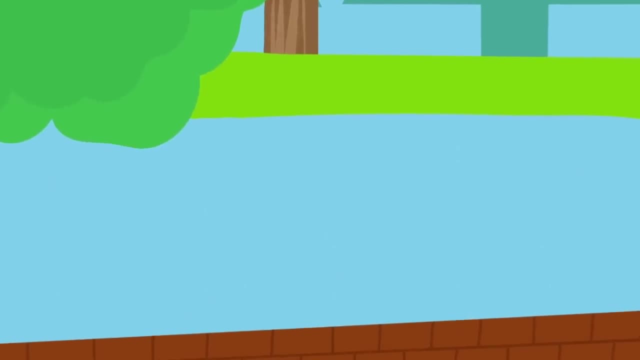 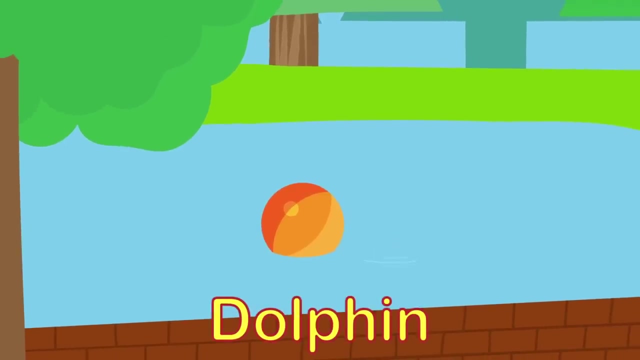 Hey, another splash- Who made that? And a ball. Now why did that ball roll away from the wall? Aha, I know That's a dolphin's nose- Good hiding place, Mr Dolphin, But the ball gave you away. 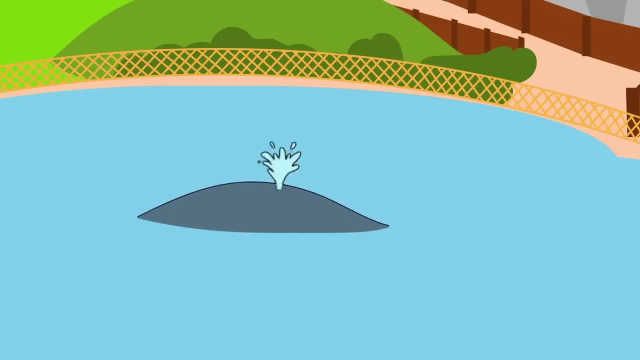 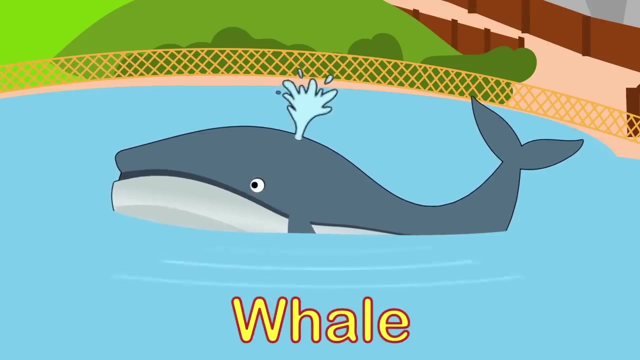 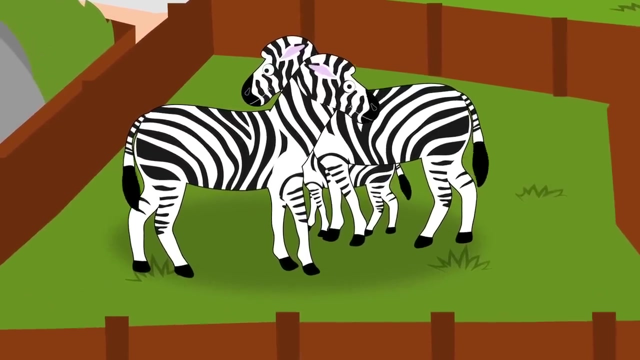 I'm sure that small island just moved about And there Did you see all that water shoot out? You did too. It's you. Well done, Mr Whale. You're so big, you nearly got away with that. Oh look, some zebras. A dad and a mum, But twelve legs between them. 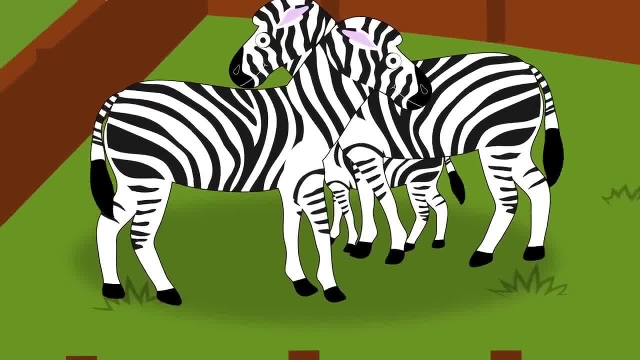 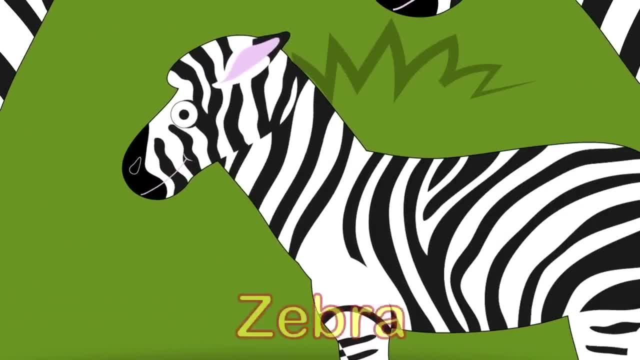 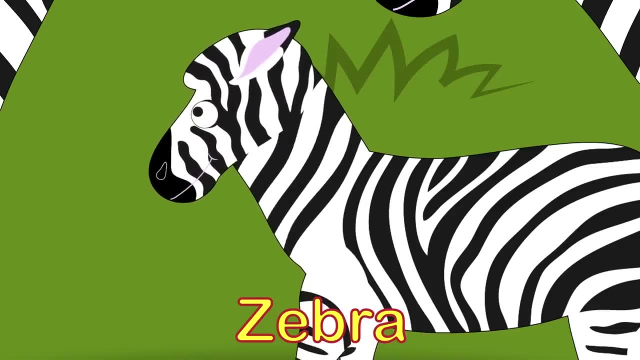 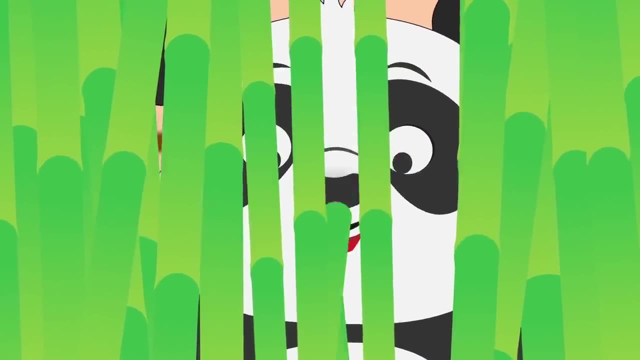 Well, that must be wrong, Unless. Ah, there is. I thought so. Hello, little zebra, What a fantastic way to use your stripes. Hey, what's that in there, Inside that bamboo? One eye, Now another. 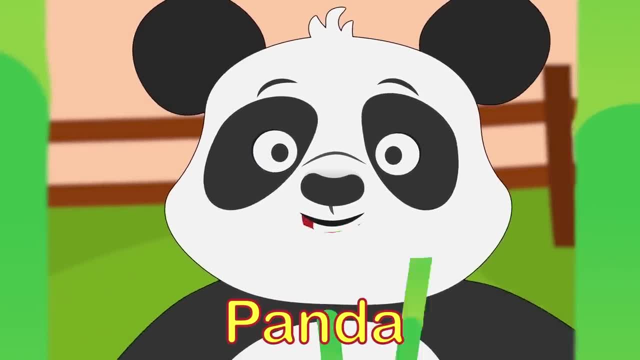 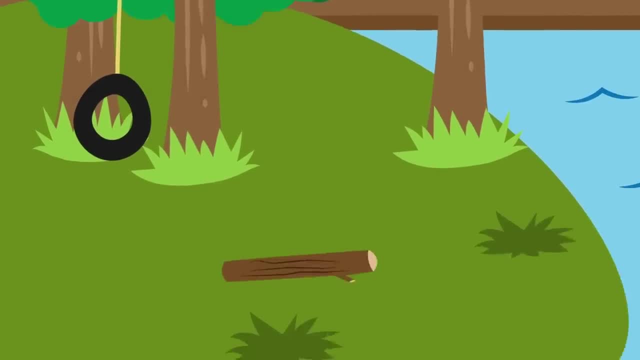 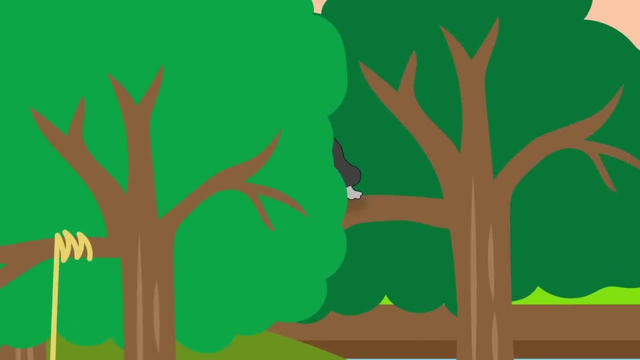 Hey, panda, It's you. Now. what hit my head then? A twig from a tree. A twig from a tree And that black shape there. Is it a knee? It is, It's a gorilla's knee. 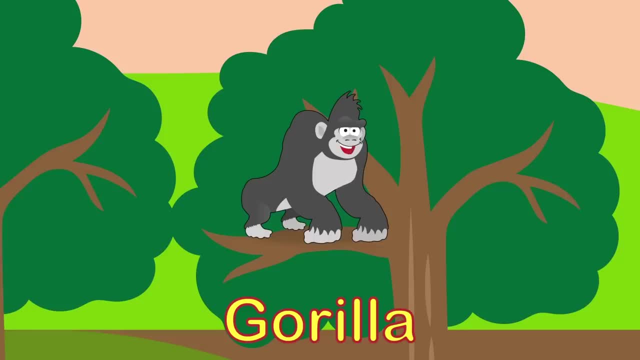 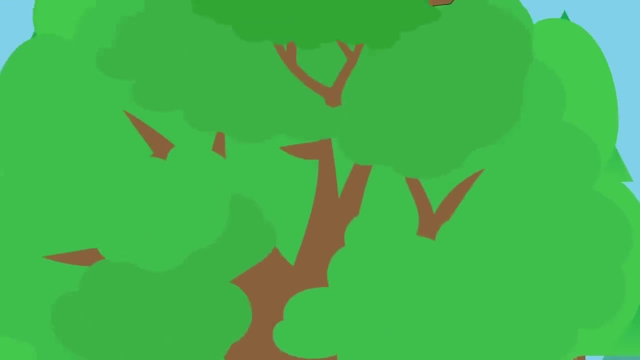 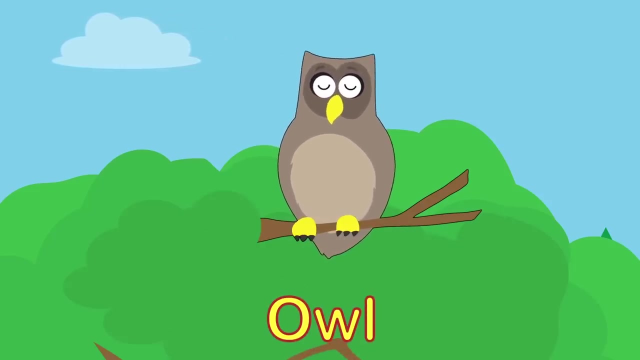 Of course You love hiding in trees, don't you? Now, what else would be hiding so high in the sky? Someone who climbs, Or someone who flies An owl? You do look tired, Mrs Owl. Have you been up all night chasing mice? 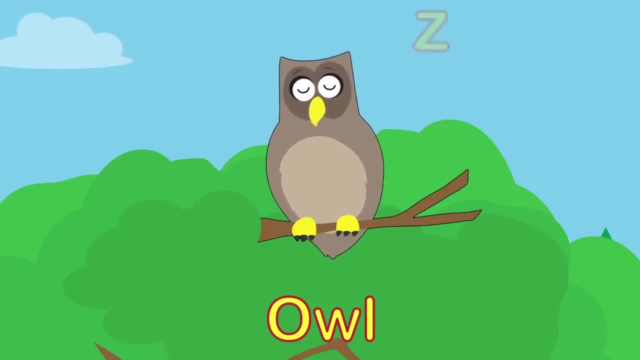 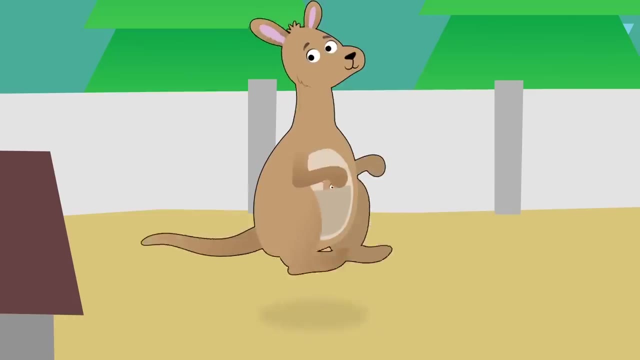 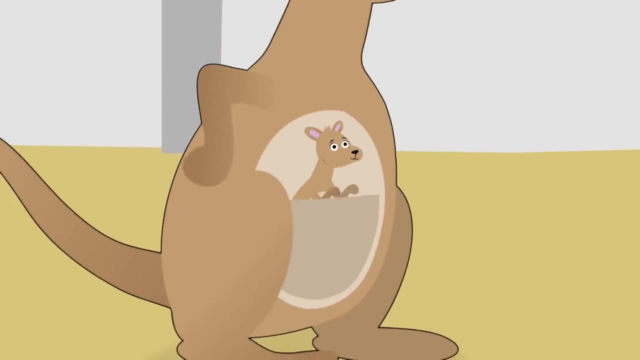 Well, no wonder you're tired. Are you having fun there, kangaroo mummy? Hey, what's that in there In that pouch on your tummy? Ah, hello little Joey, Were you hiding there all along? What a warm, safe place to hide. 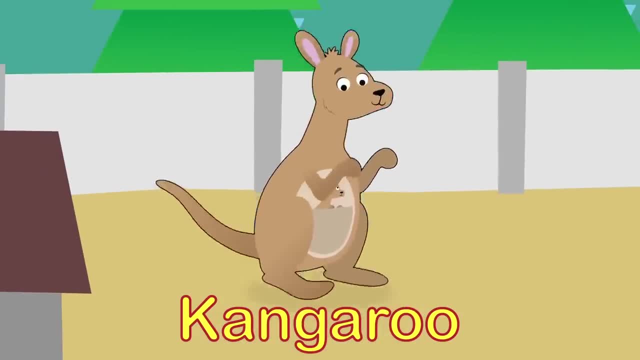 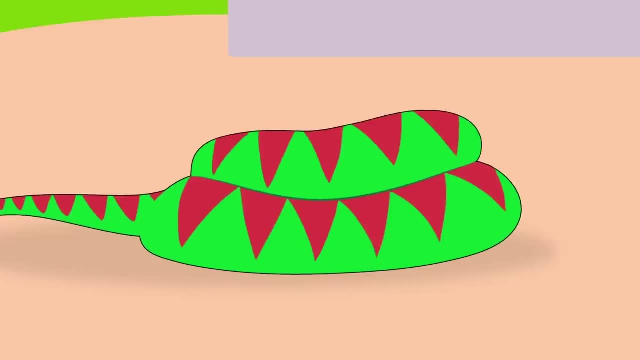 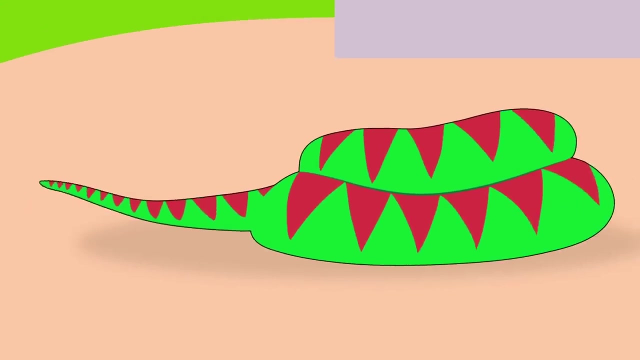 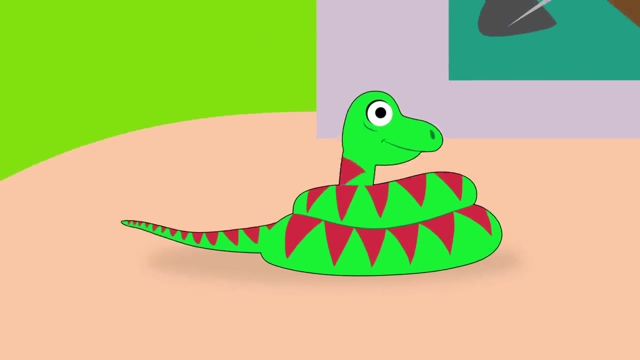 Great choice. I don't think I've noticed this hose before, With patterns all over Curled up on the floor. That's not a hose. It's hissing too much. I knew it. It's a slithering, hissing snake. 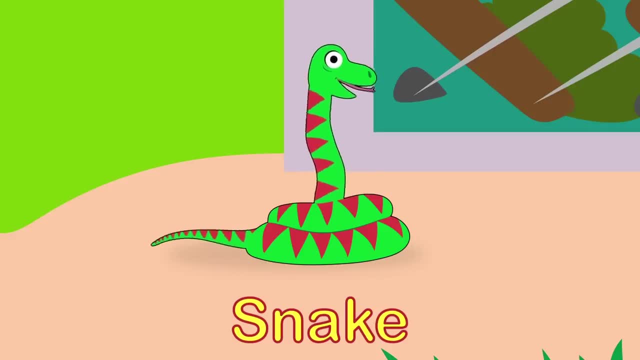 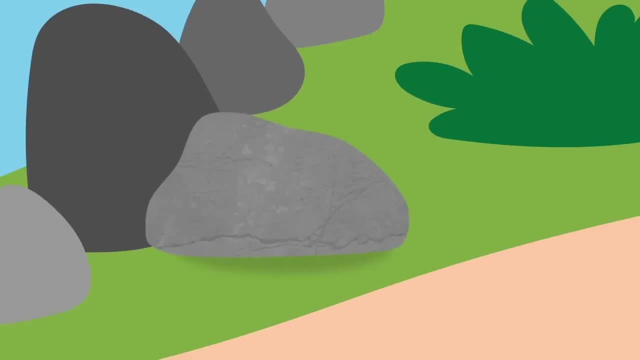 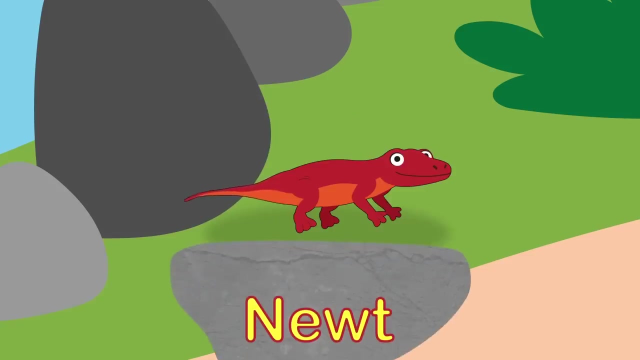 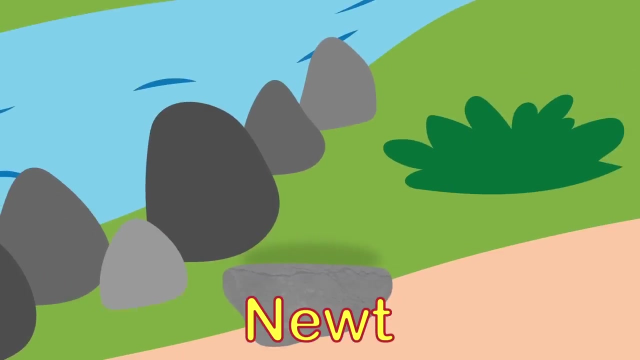 Yikes, What were they then? Somebody's toes, Somebody hiding? Oh look, now a nose, A newt nose. We found you Off. you go then, little newt, Have a nice swim. Hello, Mrs Quail, What's that by your leg? 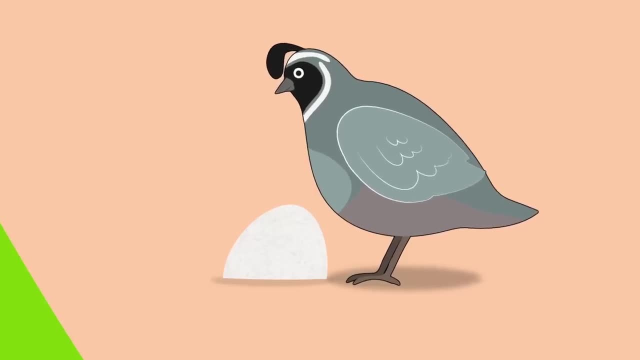 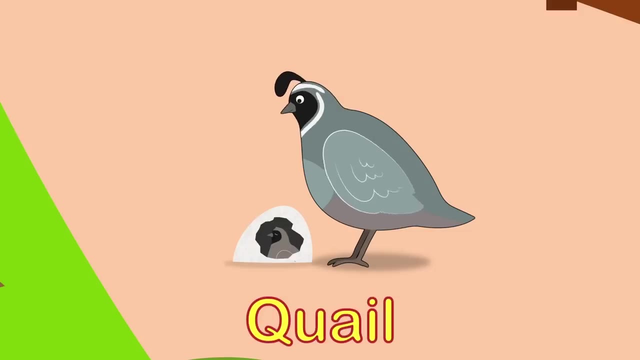 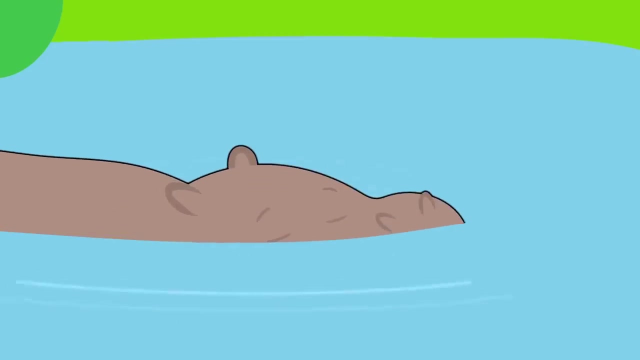 Half buried in the sand. Is it an egg? It is. Oh look, now it's hatching. You did hide your egg, so very well, Mummy Quail. Now what's this? I see in the water right here? Two funny nostrils, two eyes and two ears. 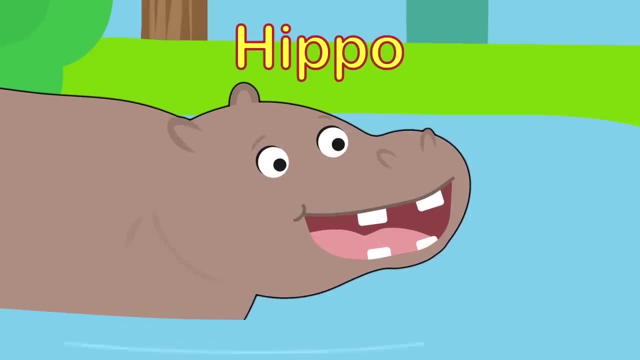 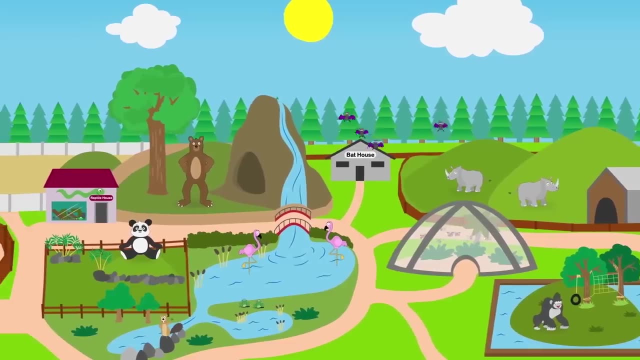 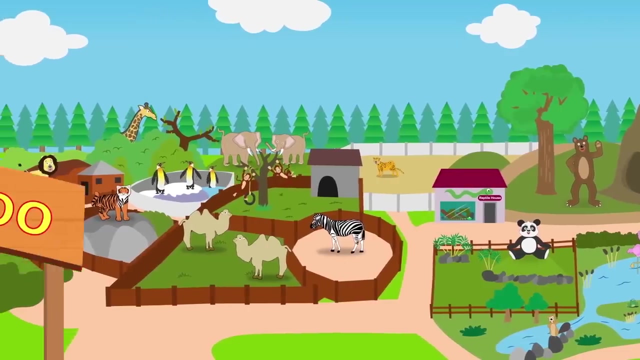 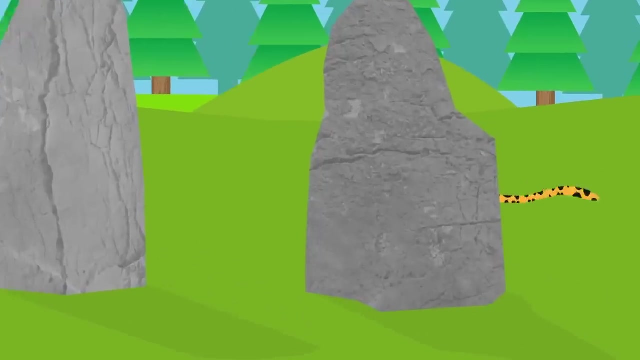 It's a huge hippopotamus. Wow, Good hiding, Mr Happy Hippo. I've had so much fun again, Have you. We'll see you next time for more Number Zoo. I see you, You're hiding Right under my nose. 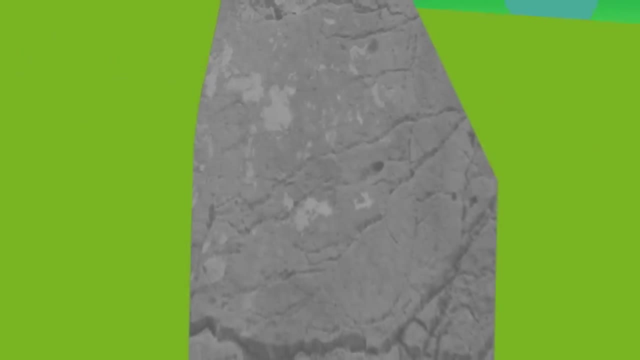 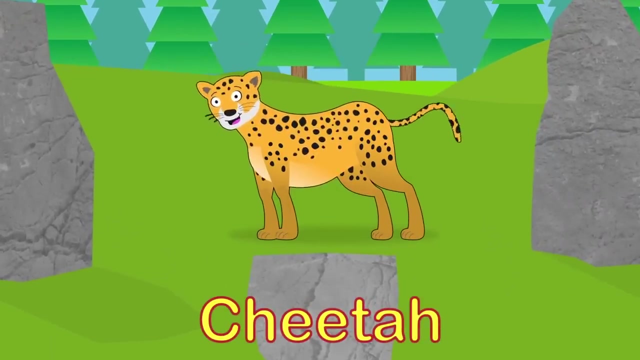 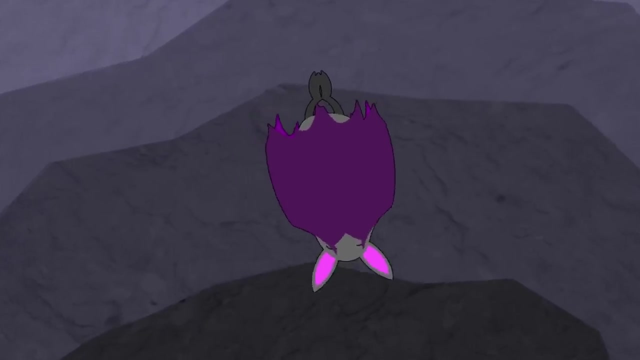 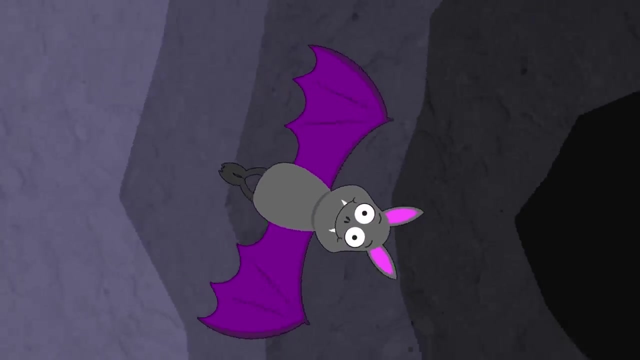 Ha ha, there I found you. Now. where did he go? Oh, you cheeky cheating cheater, You are simply too fast to see. What an odd looking shape. In fact, what is that? Ah, it's an upside down. turn around hanging down bat. 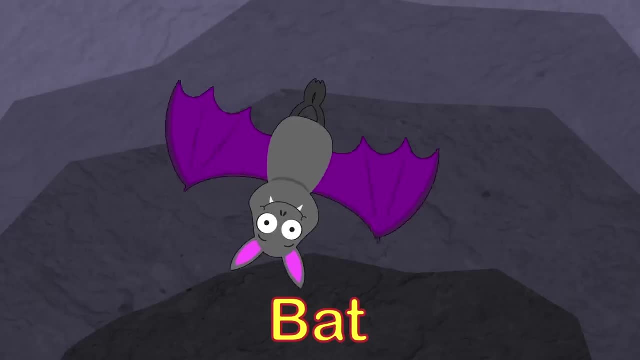 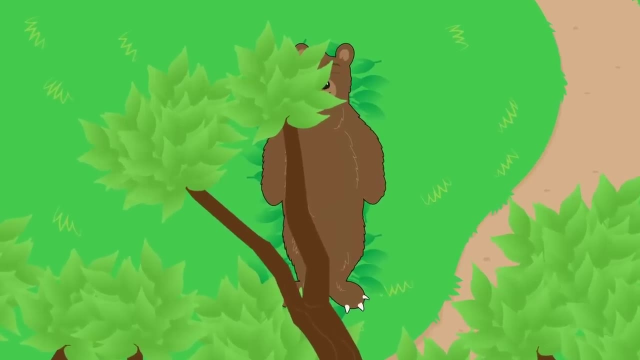 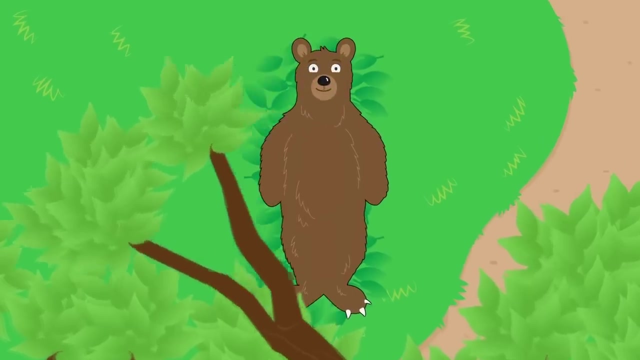 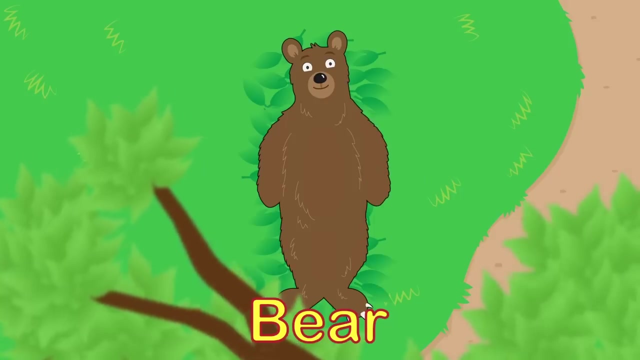 Wow, those wings make a very good cloak for hiding in, don't they, Mr Bat? Come on, let's sit down and rest over there. Hey, that's not a rug, it's a furry bear. Wow, Mrs Bear, you were so still. you really fooled me. 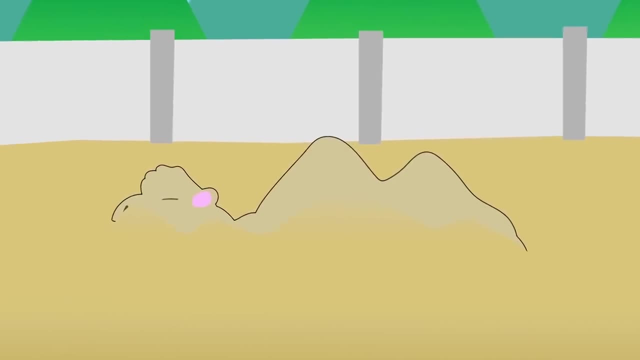 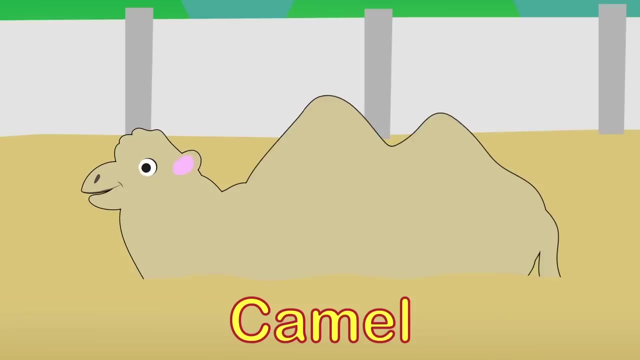 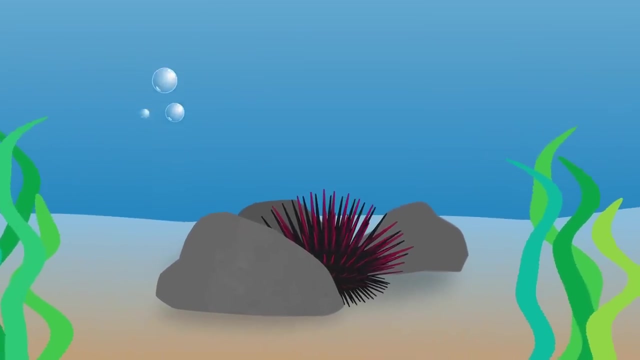 How strange. some sand just moved A big lump. Aha, that's not sand, it's a camel's hump. Great hiding place. But your hump gave you away, didn't it, Mr Camel? What's hiding there? 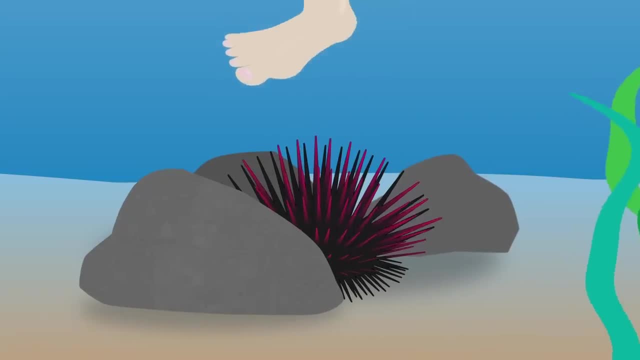 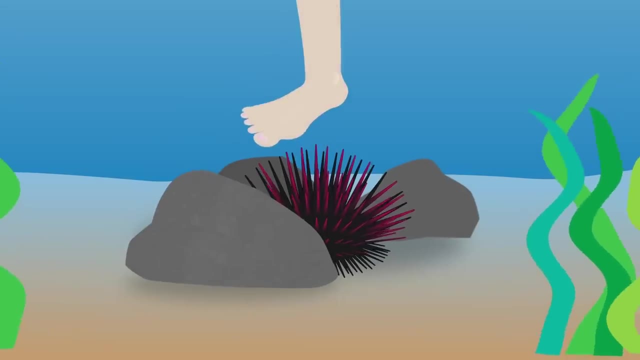 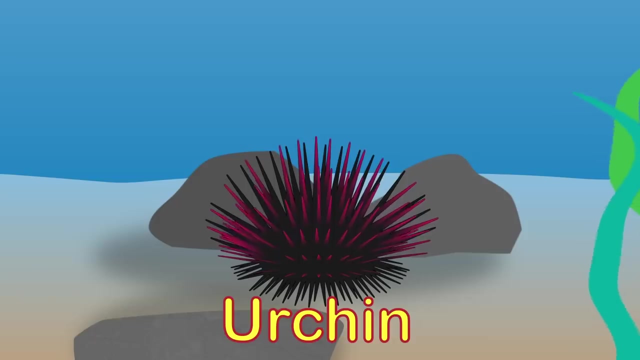 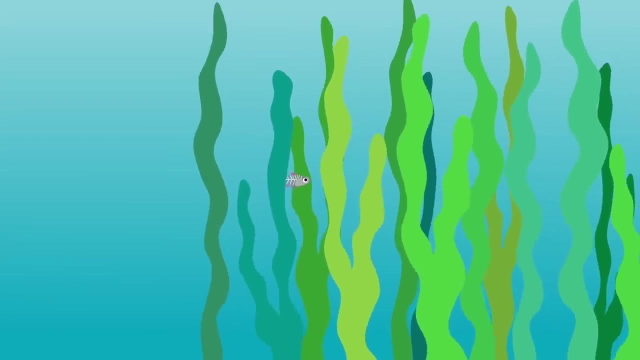 By that rock in the pool. Don't tread on it. No, no, don't act like a fool. Ouch, It's an urchin, of course. Just look at those spiky spikes. Yikes, I just saw something out for a feed. 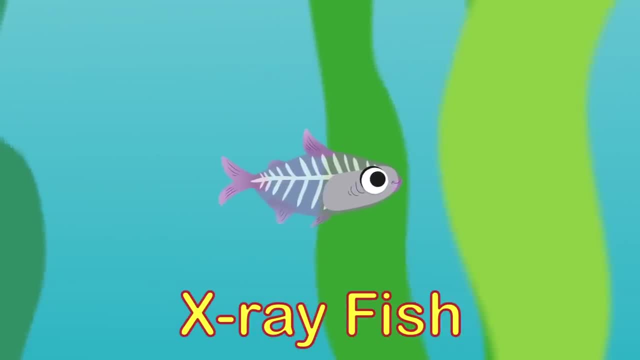 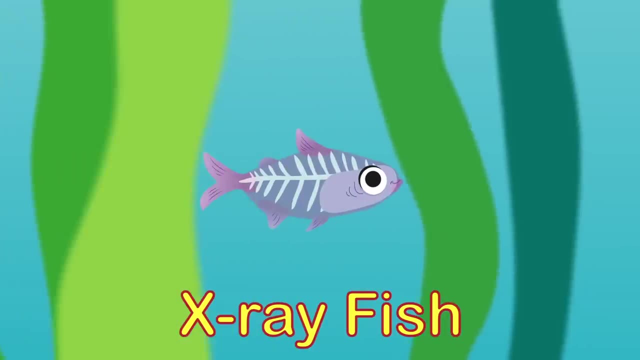 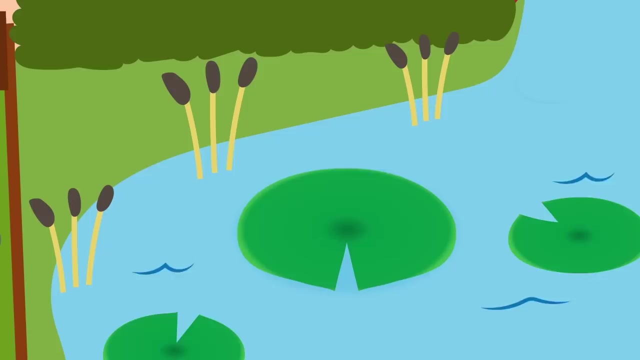 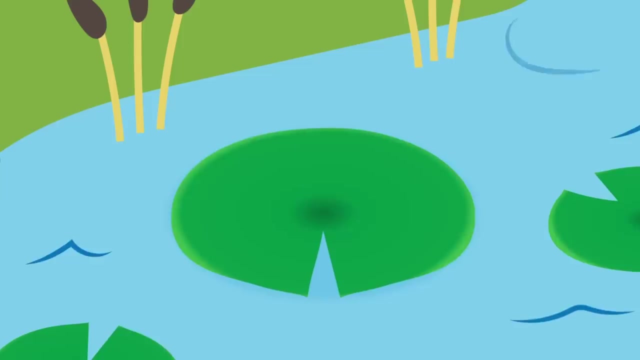 An X-ray fish Hiding in the seaweed. Wow, What a very see-through fish you are, Mr X-ray. Why is that moving That lily pad leaf? Aha, now I've guessed it: Someone's underneath. 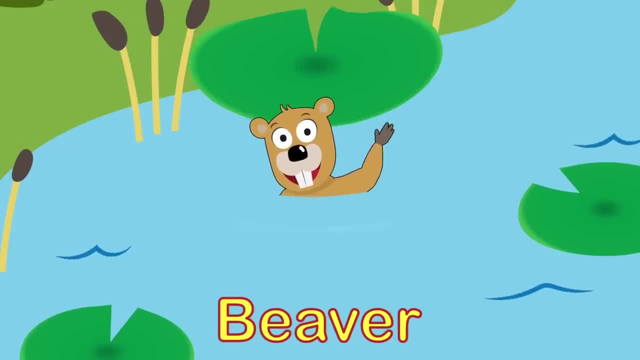 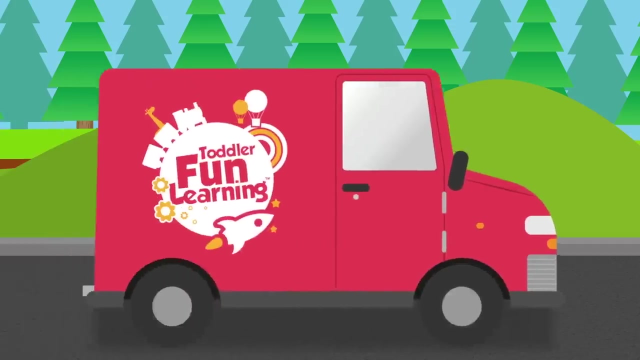 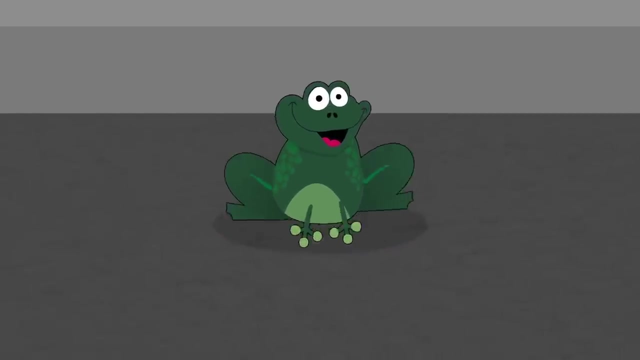 It's a beaver. Wow, You must have held your breath for a very long time to hide that. well, Hey, what moved just then Down there on the road? Is it somebody hiding? Aha, It's a toad. 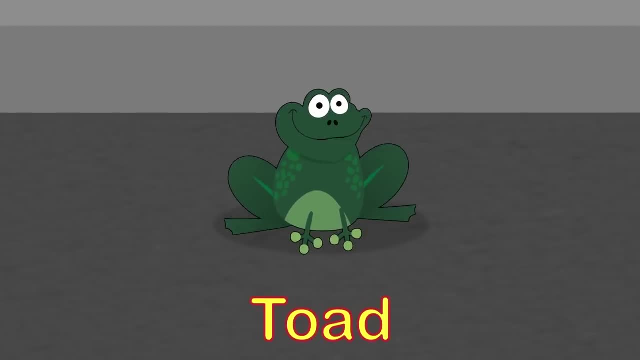 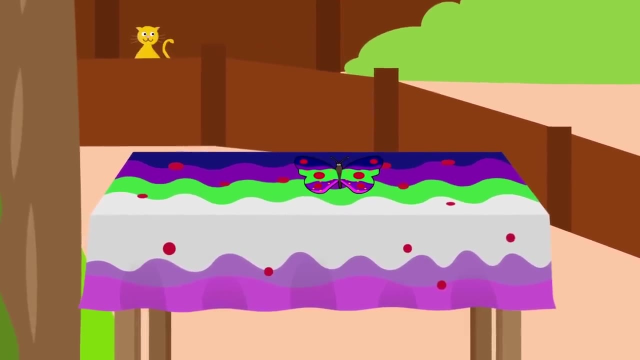 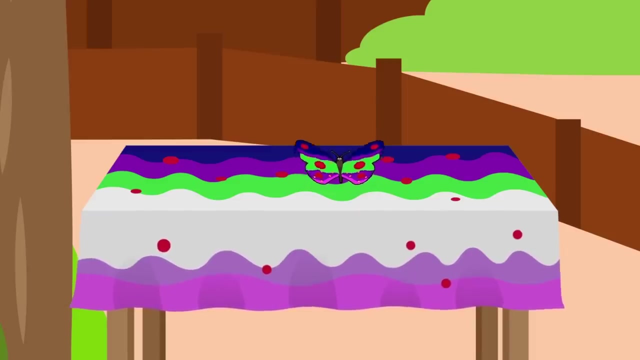 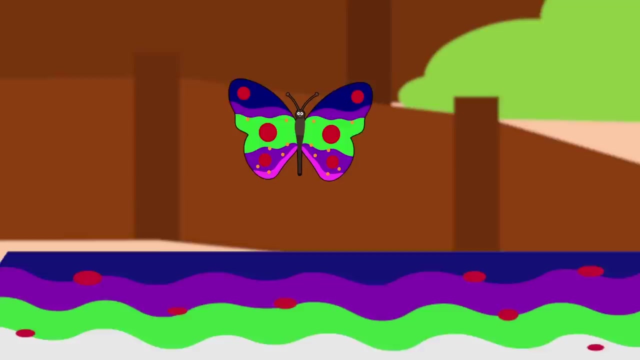 Mrs Toad, What a fantastic camouflage. Oh look, An adorable tablecloth. That pattern just moved. Or is it a moth? No, no, no, That's not a moth. Why? It's a colourful fluttering butterfly. 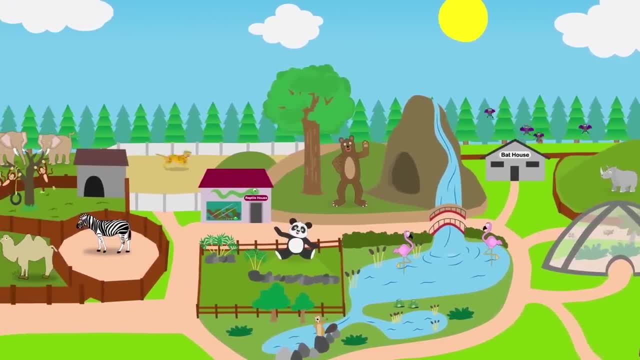 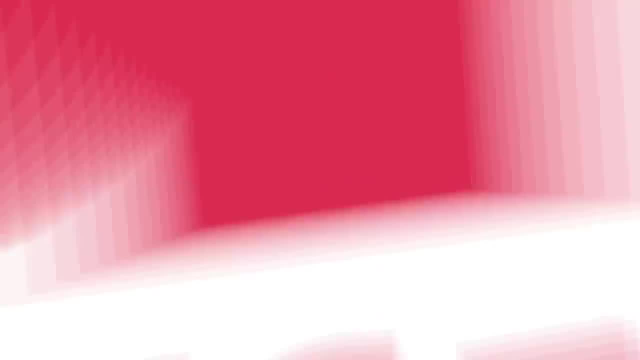 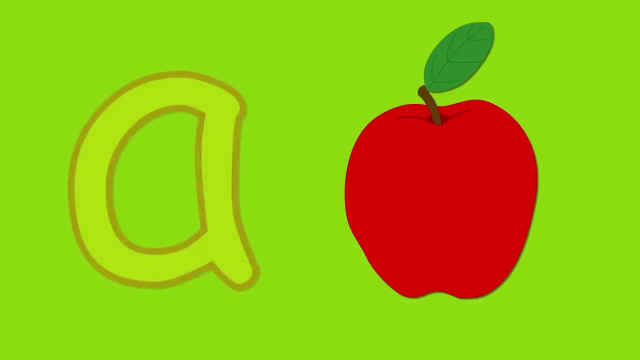 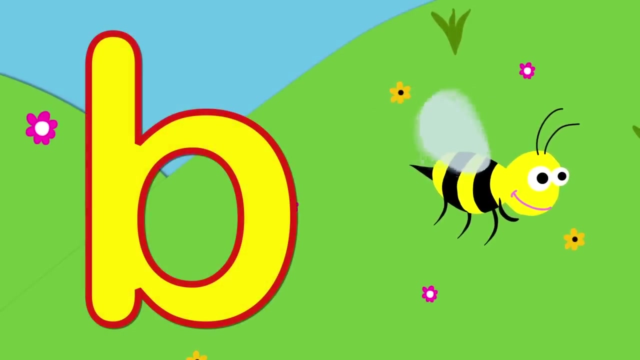 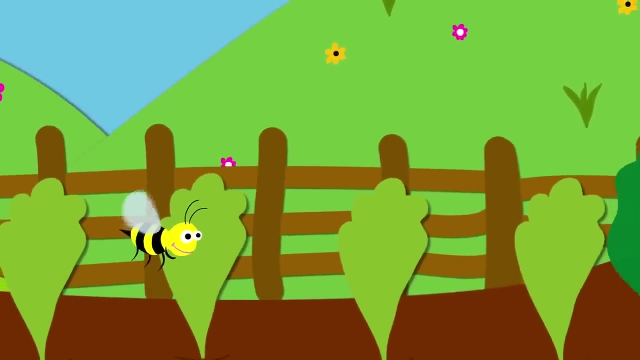 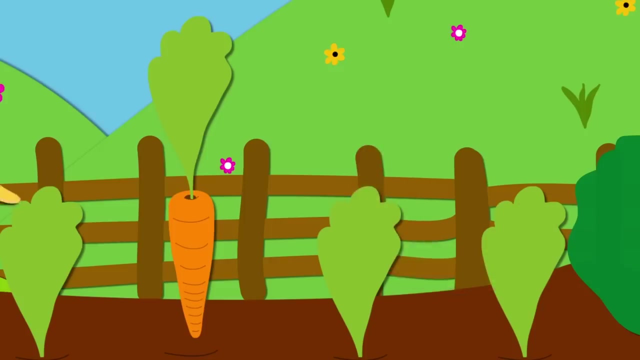 I've had so much fun again. Have you. We'll see you next time down at Number Zoo. A for apple, B for Bumblebee, B for C for B a C, A for C, B A B. 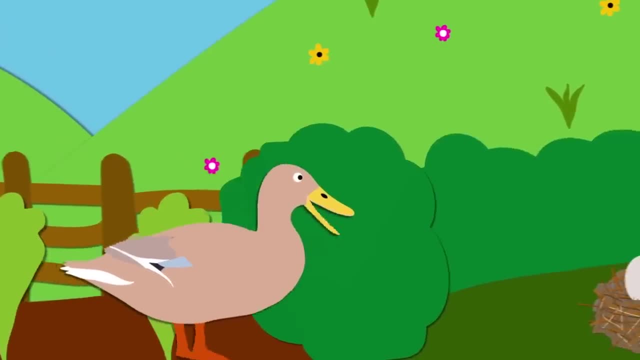 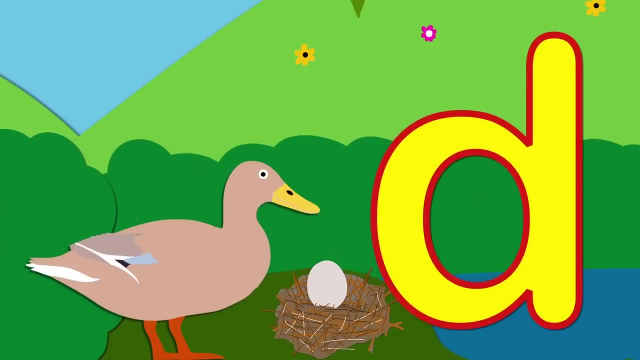 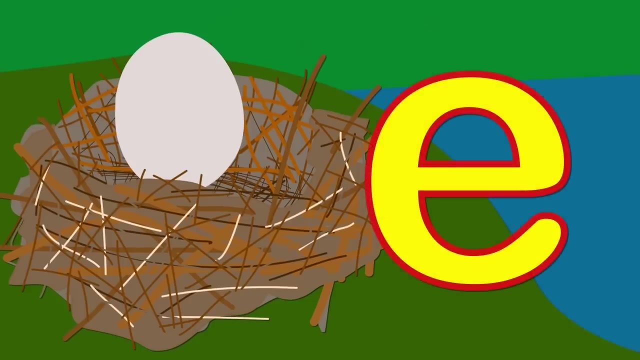 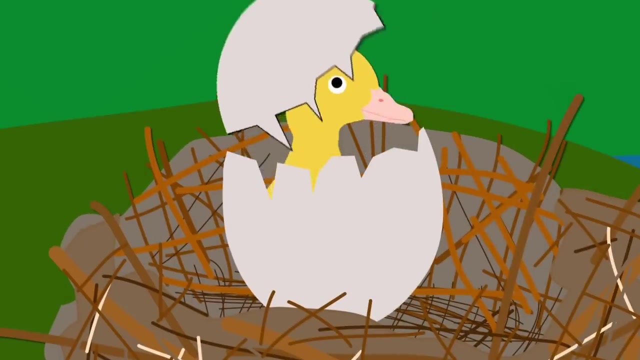 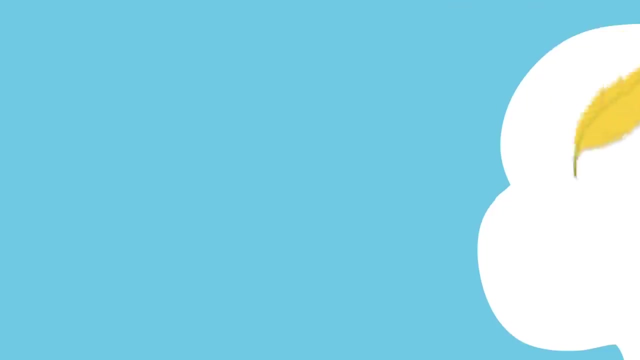 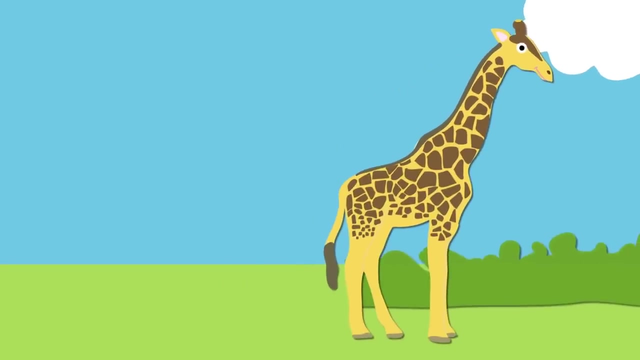 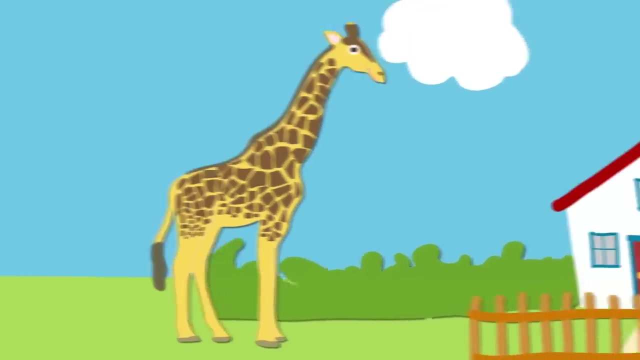 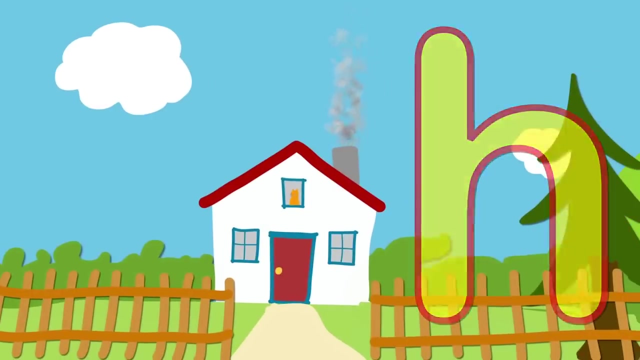 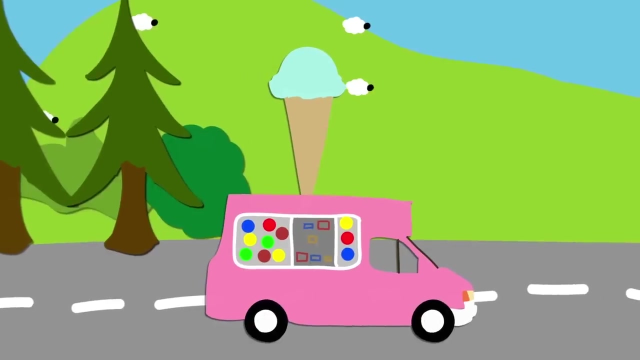 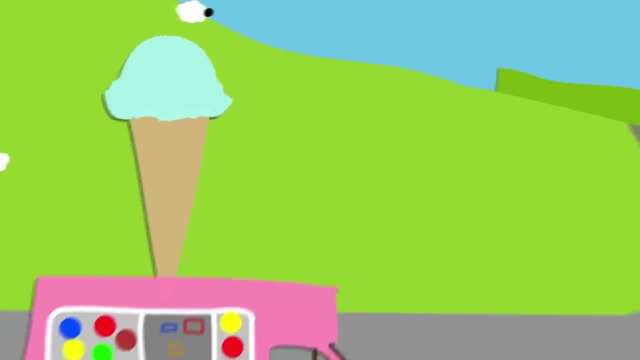 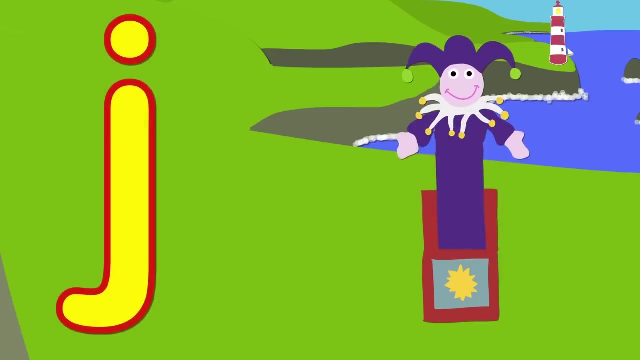 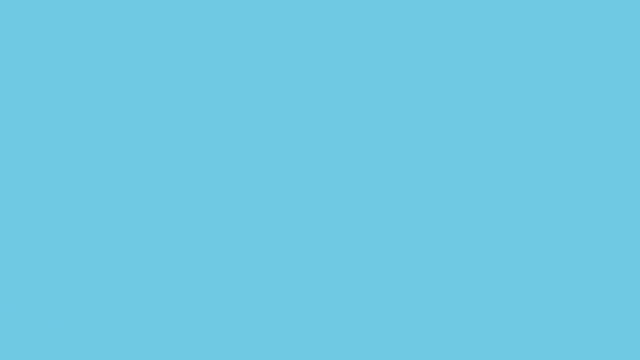 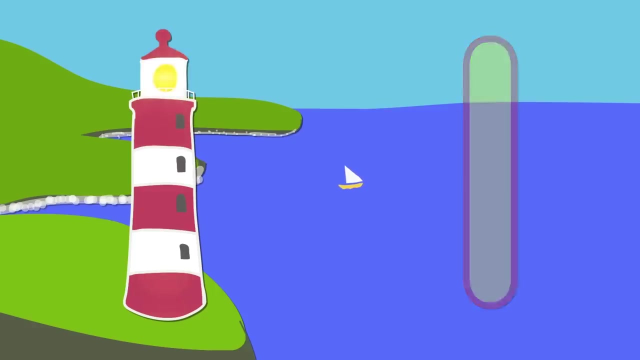 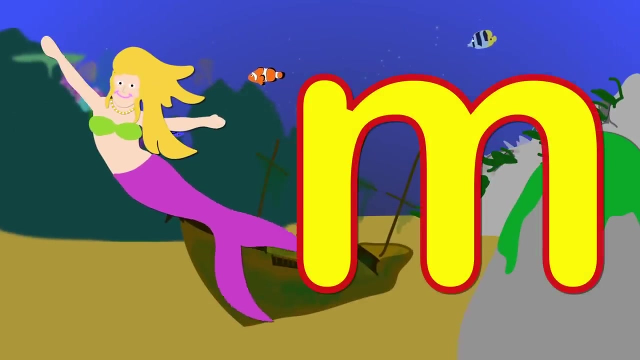 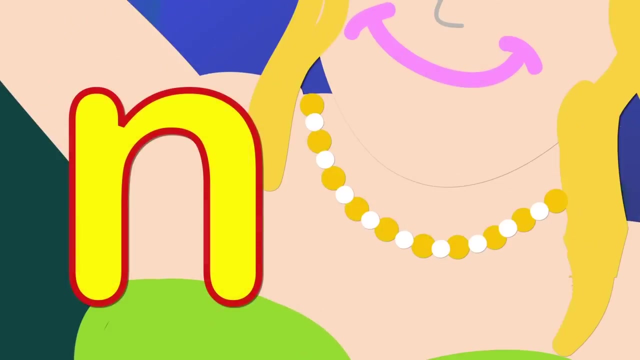 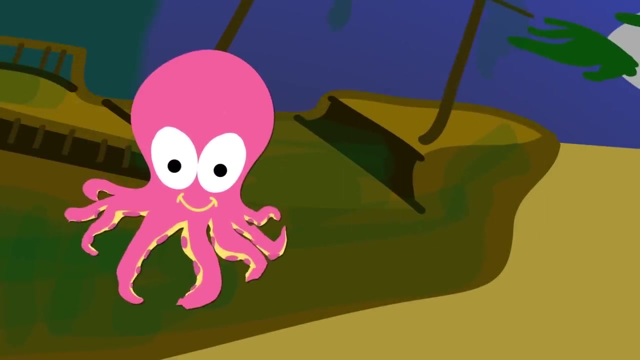 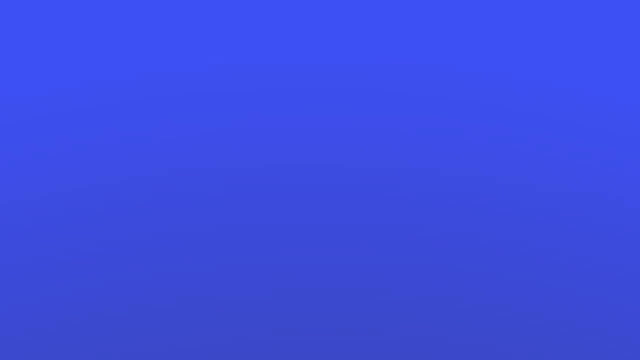 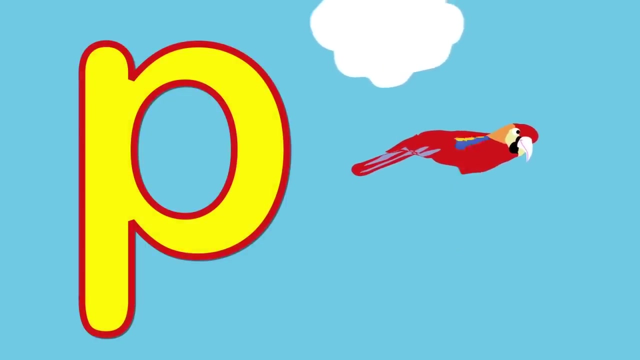 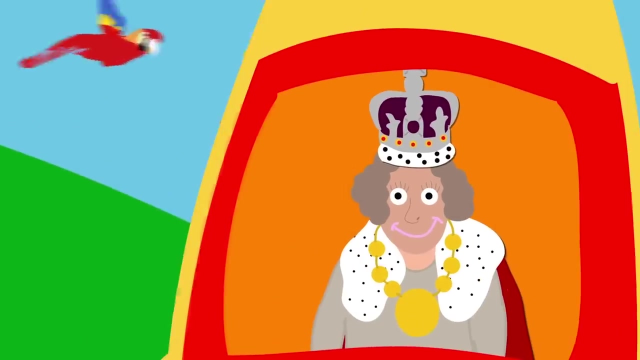 B. A, B. D for duck, E for egg. F for feather, G for giraffe. H for house. I for ice cream. J for jack-in-the-box. K for kite. L for lighthouse. M for mermaid. N for necklace. O for octopus, P for parrot.